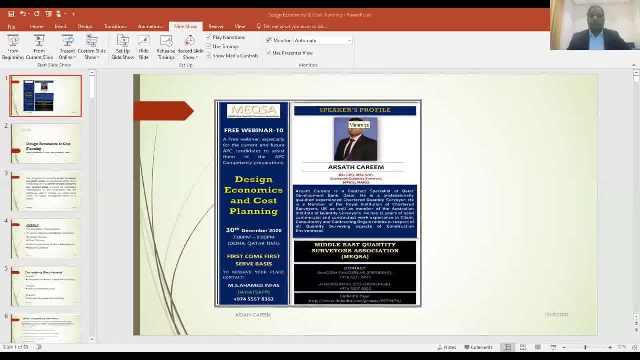 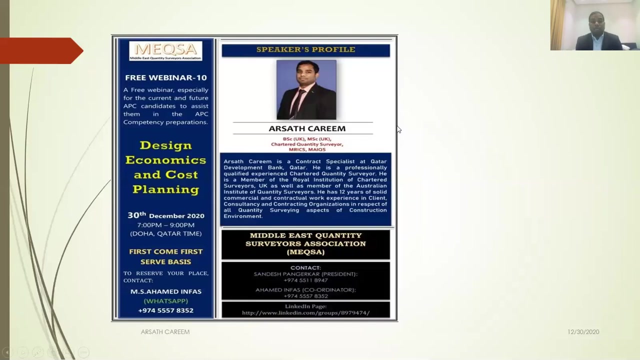 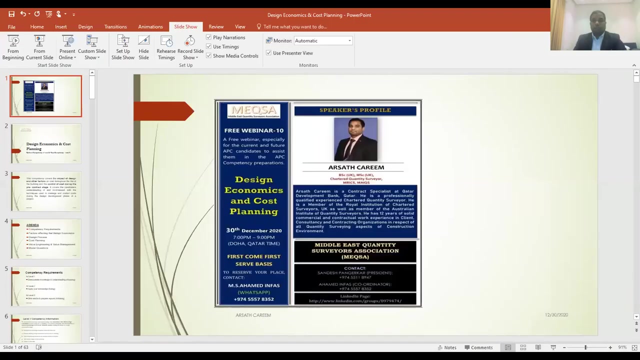 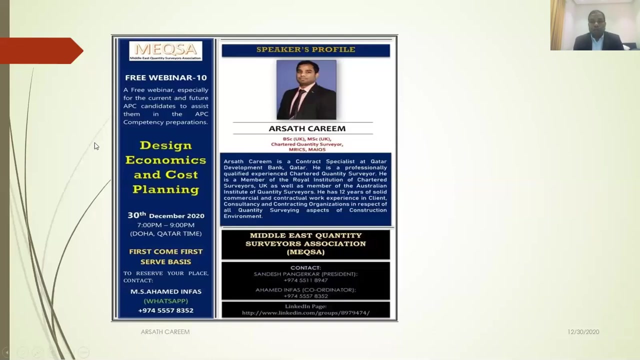 Still waiting everyone to join. Thank you, Thank you, hello everyone. good evening, assalamualaikum. welcome to webinar number 10. this webinar is specially arranged for current and future apc candidate to assist them in the apc competency requirement. today topic is design, economics and cost planning. it's me, arshad karim. i'm a chartered 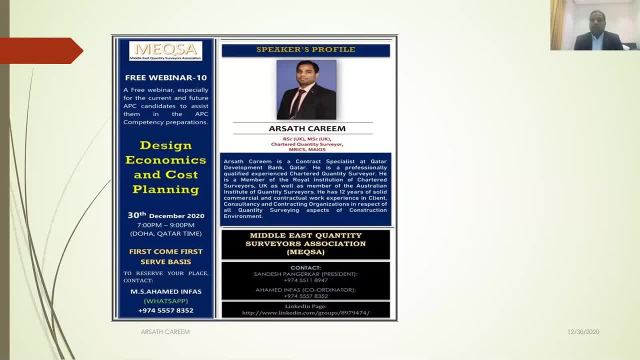 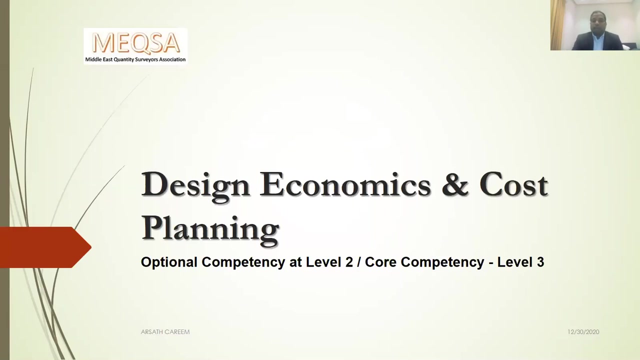 quantity surveyor currently working as a contract specialist with qatar development bank from last six years. totally overall, i have a 12 years experience with client organization, as well as contract organization and consultancy as well. today, our topic is design, economics and cost planning. this is a core competency for level three, as well as optional competency for level two. 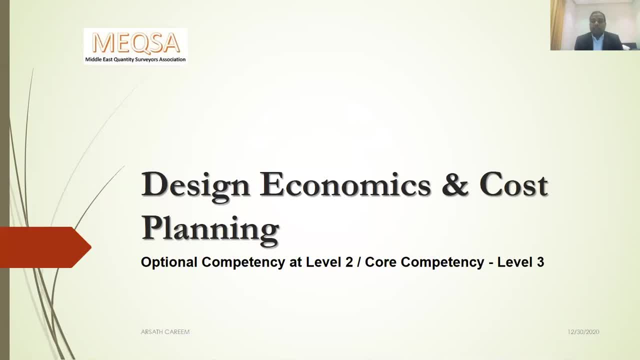 whoever working in consultancy organization you can choose as a co-competency for level three: whoever working with the contract organization, you can choose. you can choose as a competency level two: design, economics and cost planning. first of all, you have to understand from the wording what does. 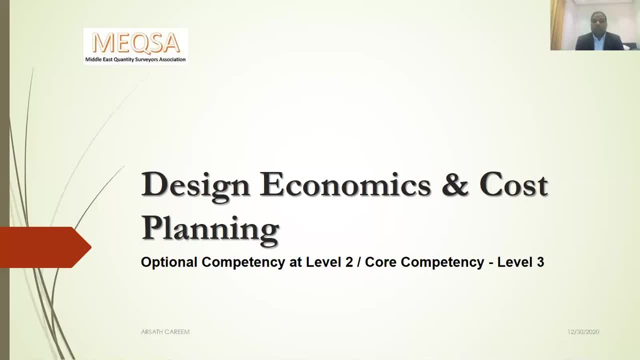 mean? what is design, economics meaning and cost planning? it's mean design the building in economic way. for that one, we are using cost planning as a major tools. that is what all about we are going to discuss in next two hours. please stay with me. according to the rics, competency guidance. 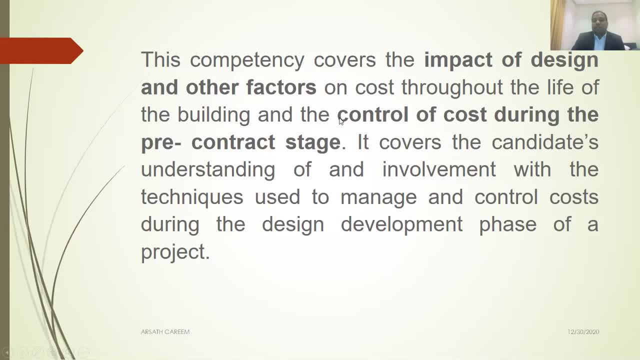 this competency covers the impact of design and other factors on cost throughout the life of the building and control the cost during the pre-contract stage. you will learn to this competency what are the factors affecting the costing of design and how you control the cost. what are the mechanism available to control the cost. 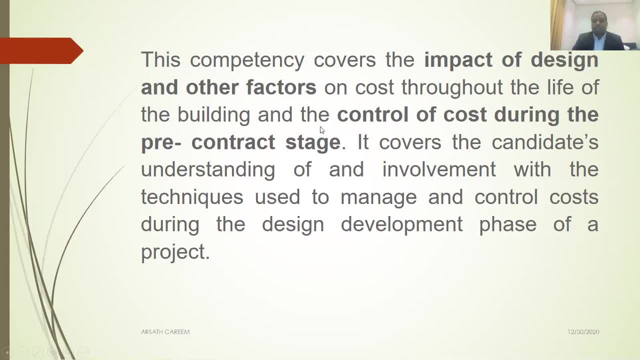 during the pre-contract stage. as you all know, pre-contract stage is very crucial to any projects, from establishing the budget up to tender stage. it's very crucial to play the role in the project 생각이 nating- very crucial to control the cost, because construction is a business, it's all. 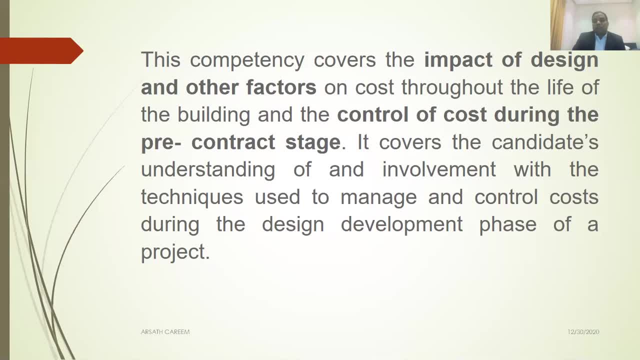 about money. it involves lots of money. so cost is the major factor. cost is the reason you you involve in this business. so you have to, you have to make sure you have to reduce the cost much as possible to increase the profitability of your company. therefore, you have to understand the basic things in next, 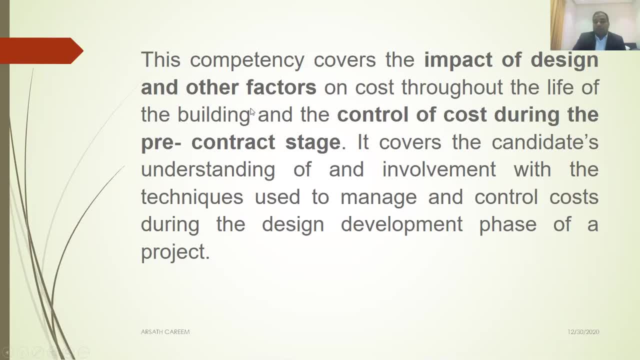 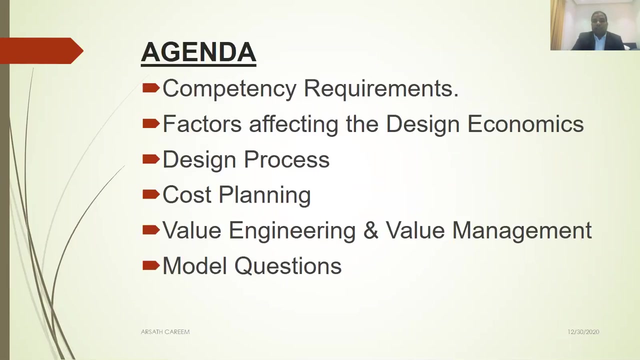 slides you will. you will, I will cover throughout this presentation: first, discover candidate understanding and involvement with the techniques used to manage and control cost during the design development phase of project. we will see what are the design development stages in this contract during this presentation. presentation I will cover following major topics: the competency requirements. 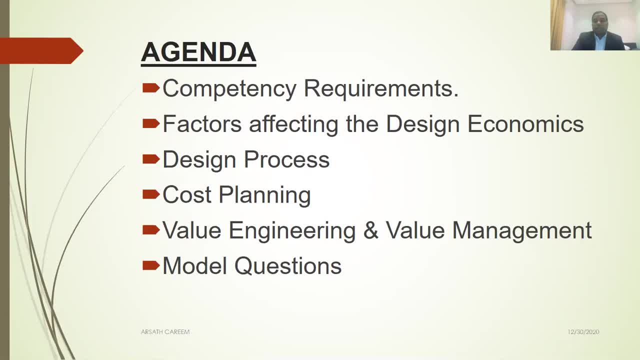 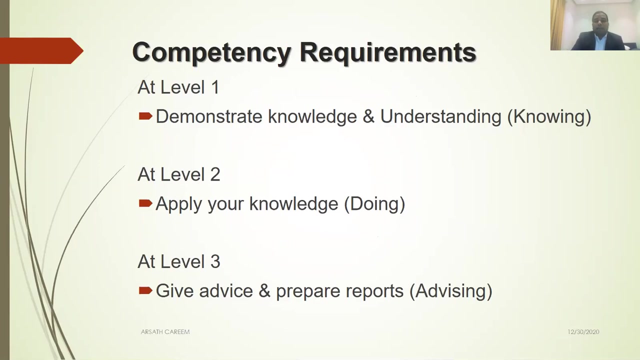 factors affecting the design, economics, design process, cost planning, value engineering and value management. and some moral question in in regards to our ICS interview panel. as we all know the competence requirement at level 1, what RIC is expecting from you? to demonstrate knowledge and understanding. it's all. 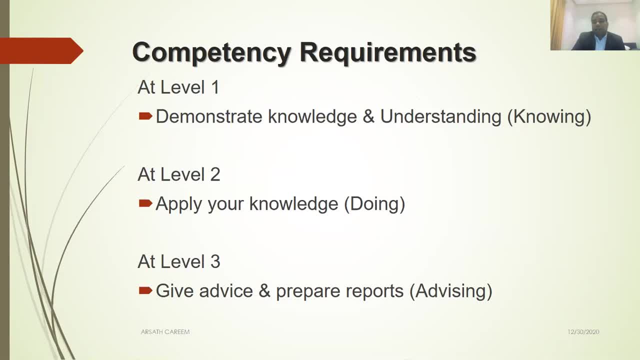 about knowing. normally it's a theoretical part. they will ask a direct question from you: what it is, how it is, what are the factors? you have to understand and demonstrate what it is. at the level 2 you have to apply your knowledge, what you understand, for example, preparing the cost plan, how you 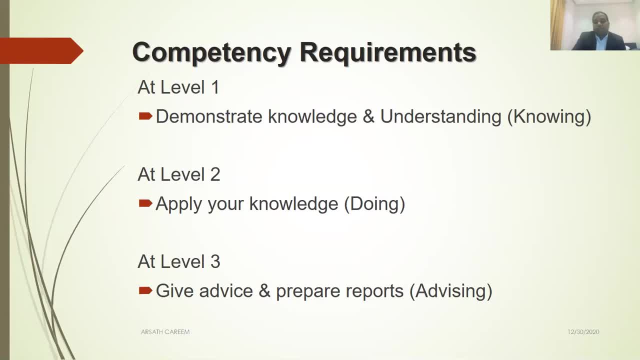 prepare the cost estimate, how you conduct the value engineering. at this level 2 you have you. you should know how to prepare it. at level 3, you should able to know how to advise. also, it's a prepare reports. if you choose this competency as a level 3, you should able to advise. you should able to communicate with your. 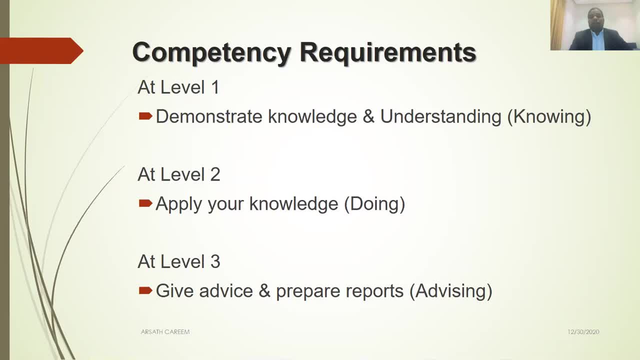 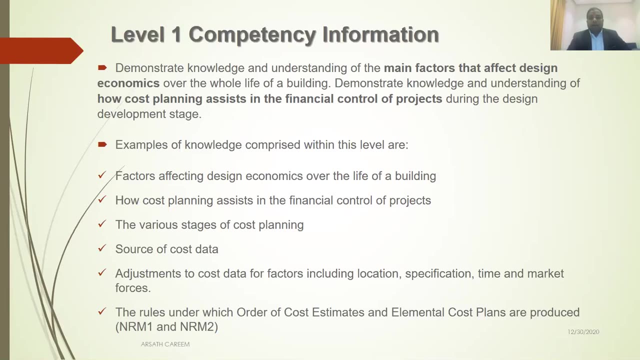 client with the design team advice, prepare reports. so our ICS fine gauge is expected at this level 3. these are- I pick it from RICS pathway guide, which is which are the things you have to. you have to make sure you you are will aware about this before you're going to interview at this level you. 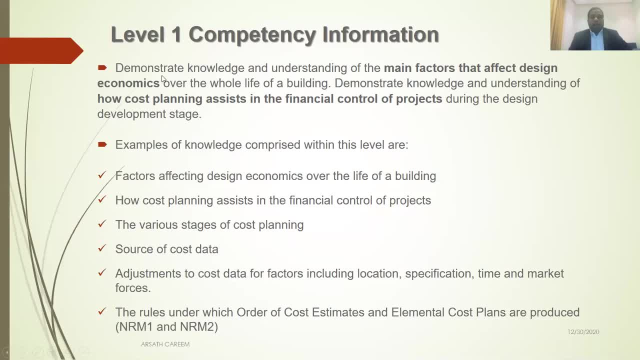 should able to advise, prepare reports. so RICS expecting at this level 3- you are well aware about this- before you going to interview at. this thing should be washable until after. the link is WEB: Wool Geg入 semester two. but you should be able to demonstrate knowledge and understanding the main factors that affected design economics. 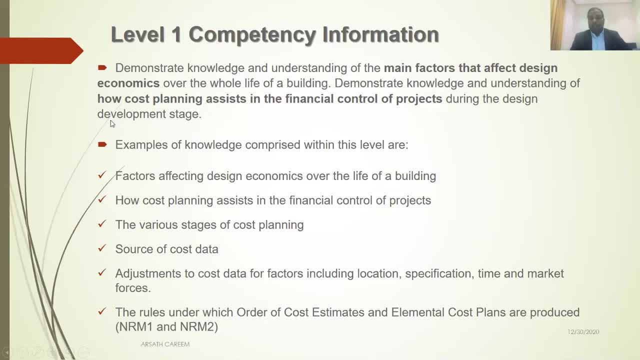 over the whole life of building. in later slides you will know what are the main factors which is affecting the design. also, you should able to demonstrate knowledge, understanding how was planning assets, assets in the financial control of the project during the design development stage. in the later stage, later presentation, you will come to know everything. 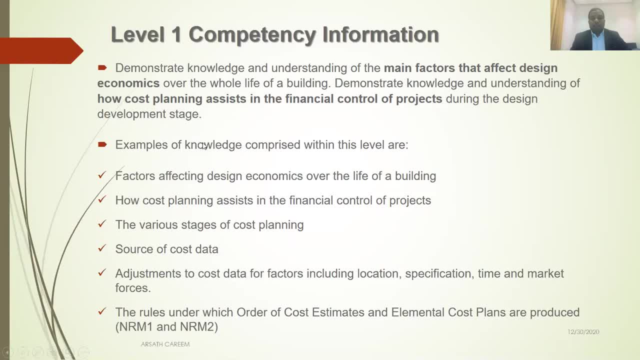 which is included in my presentation. these are the things i pick it from our ics apc pathway guide. once i finish my slides, you will cover all this knowledge. i don't need to read and waste the time, rather i will go directly to them. level 2 competency information. 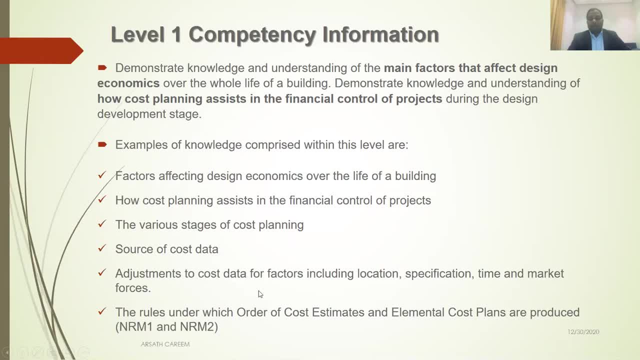 this is you can read in our ics pathway guide as well. also, once you finish this presentation, you will able to understand all the all these things. also the another things you should know. as part of your apc process, you have have to write summary of experience. so while you're writing the summary of experience, 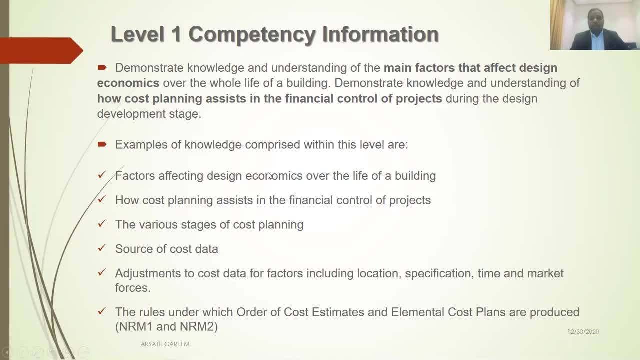 you should able to cover these things you learn from, from your university or undergraduate courses or any cpt you attend, or from your own reading or discussing with your friends. you should able to understand this knowledge. what, what are the factors affecting design economics? how cost planning assists. source of cost data. how you 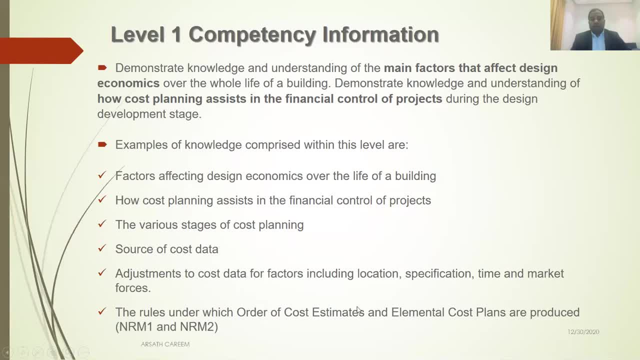 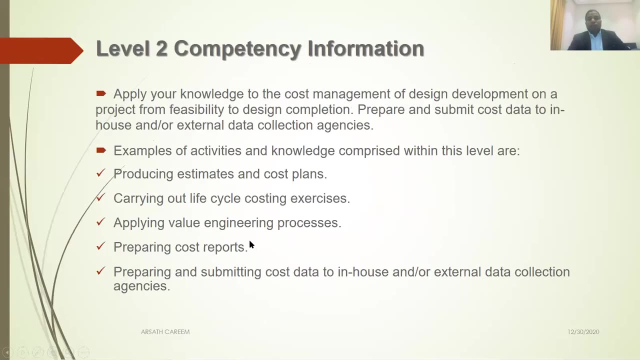 adjust the cost data? what are the rules of order of cost estimate? these things you should able to understand during your studies. so while you're writing summary of experience, try to cover these things on your writing. level two: you should able to produce cost plan and cost estimate. also, you should know how to. 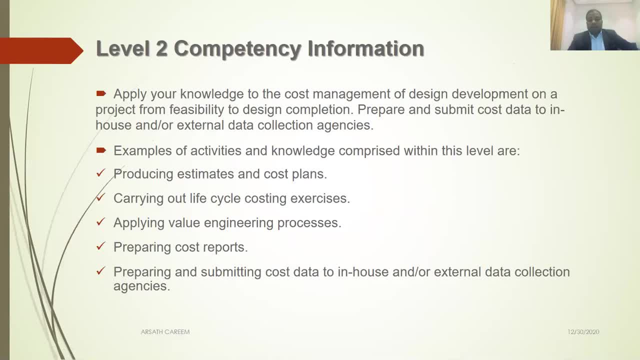 carry out life cycle cost exercises, how you apply value engineering, how to prepare reports, how to submit the cost data. these are the things you have to cover. you should able to know while you working. so, while you writing your summary of experience, you have to say: while i am working this project, i did cost plan in order to control the project. 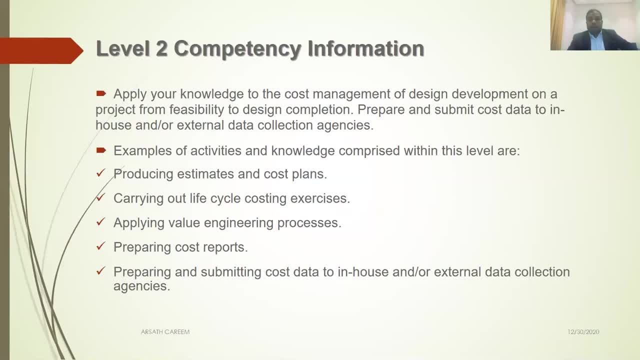 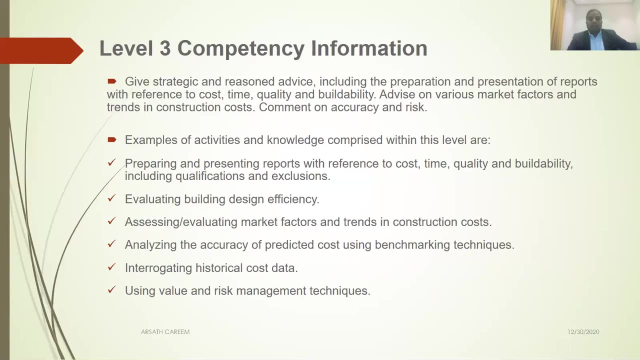 during the pre-contract basis. this kind of wording you have to mention in your writing, like you did, how you did when you did. these are the things you have to include on your summary of experience. level three: you have to able to give strategic and reason advice. 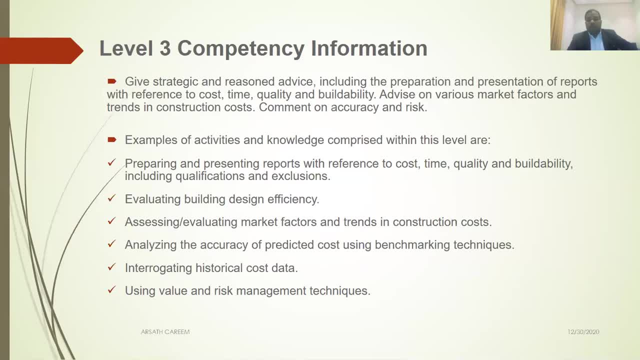 how you can give strategic advice, for example, when your when your project budget more than the client budget, when your cost plan is more than the client budget, how you advise your client. so these are the experience they're looking for: rics interviews on your daily working life. how you 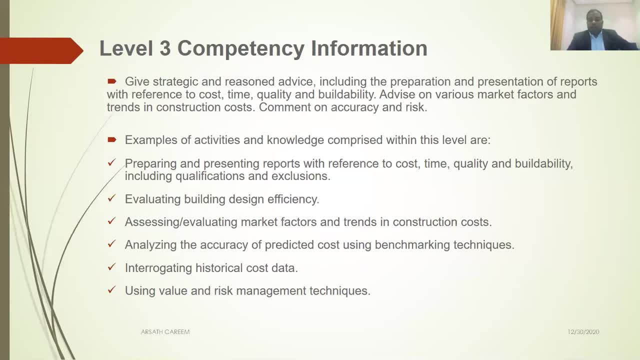 face these kind of circumstances. while you're writing your summary of experience, you have to give evidence for for for which you cover during your working time. so whoever choose level three, whoever working with consultancy, should able to know how to prepare a course plan, how to communicate with your client, how to communicate with your design team, how to use the. 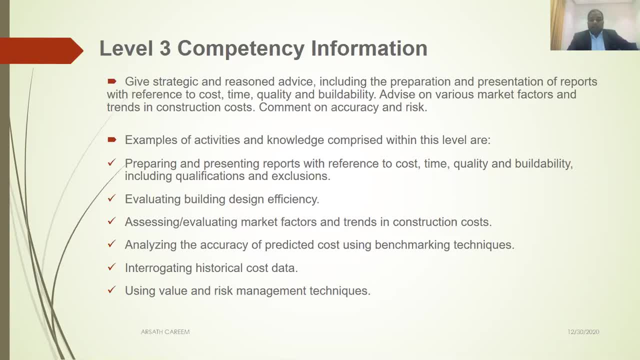 value engineering techniques, how to communicate with your design team, how to use the value engineering techniques when you require to reduce the cost. these are the things you should write, with evidence, with a scenario in your summary of experience. so so far what we discussed, just a pathway guide. 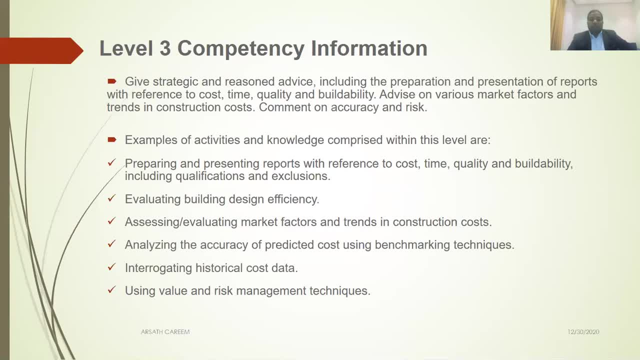 which required you to cover during your summary of experience writing. also, when you go to interview, you should able to demonstrate yourself what it is when you did, how you did, how you advise to your client design team or your project team. next, we are going to discuss about the what are. 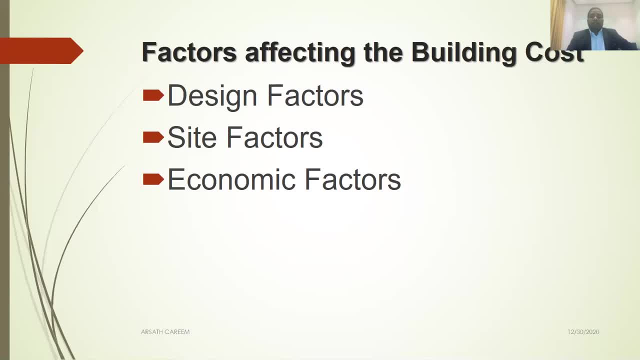 the factors which is affecting the building cost. this is the basic of the design economics. what are the factors affecting building cost? these things you may learn during your undergraduate studies. these are the basic things. i will go through quickly. building cost mainly affects design factors, site factors, economic factors. we will see next slides what i, what it is. 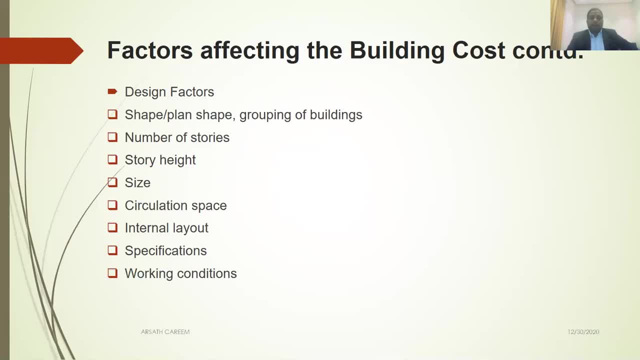 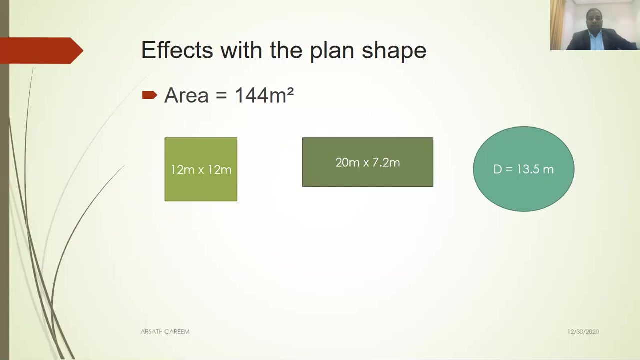 factors affecting the building cost: design factor, for example, shape plan grouping of building. definitely, the shape of the building is the main factor, main element in terms of deciding the cost factor. let's see how it's affect the building cost. for example, on this diagram, you, you have to build the area 140. this is 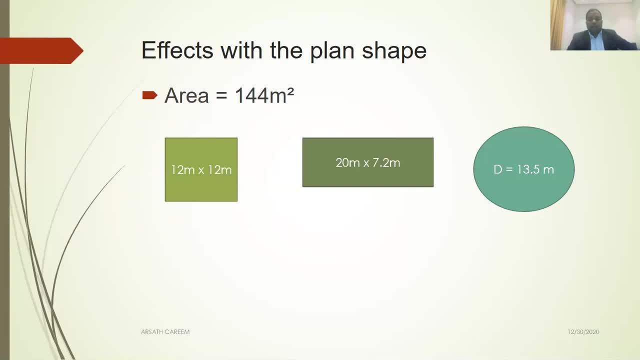 the example how the effects of the plan of with the plant shape, how the shape is affecting the building cost. let's say you have to build 140 meters square small room. you have to you what is your intention. you have to build 144 meters square. options available in terms of shape of the building first, in the easiest way you can make a. 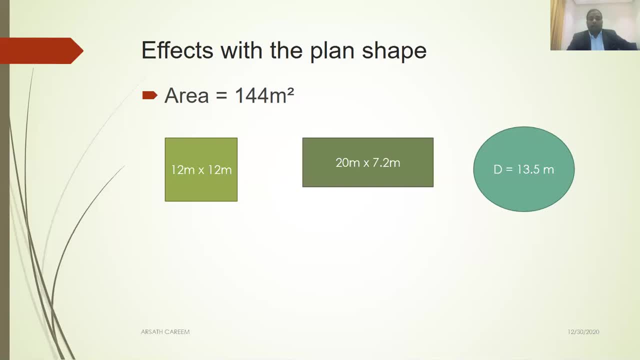 make a 12 meter into 12 meter easily. square shape also. you can make rectangle shape, 20 meter into 7.2 meter also. you can make scar building near to that area, diameter, 13.5 meter. in all three method you can achieve the same area. what you look at, however, this shape will affect. 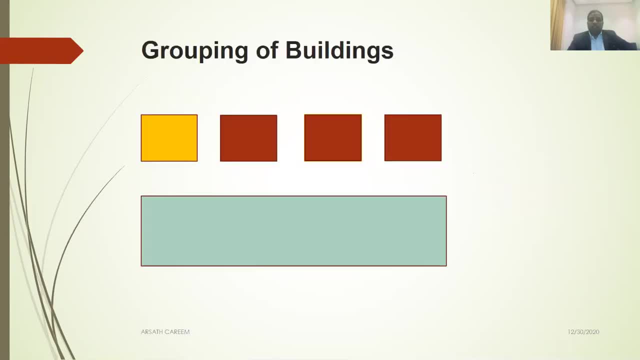 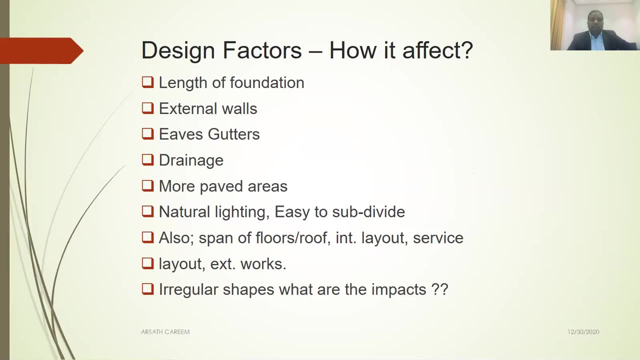 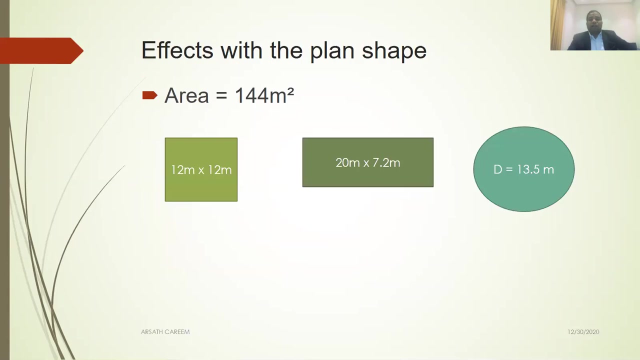 the cost, how you will see here, because because of the shape, the length of the foundation will differ, because of the shape, external walls will differ, if gutters will differ, drainage, paved area, natural lighting, span of floors, layouts- these are the things will affect. also, imagine if you, if you build an irregular shape. 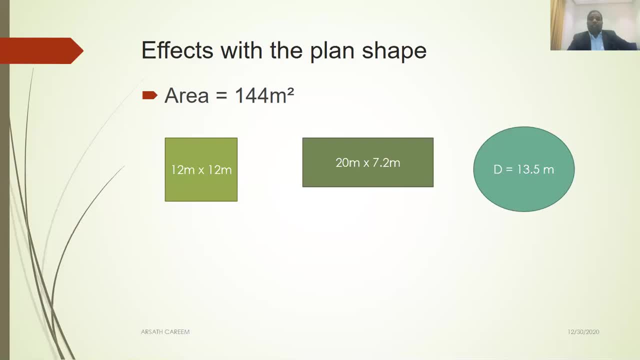 irregular shape is more complicated, normally very costly. for example, if you are living in qatar, there are many buildings which are regular shape. they build for attractive tourist attraction, for example, qatar museum building. if anyone go to konish, you may experience this type of building- the building- not by not considering the cost. what they need is a pride. 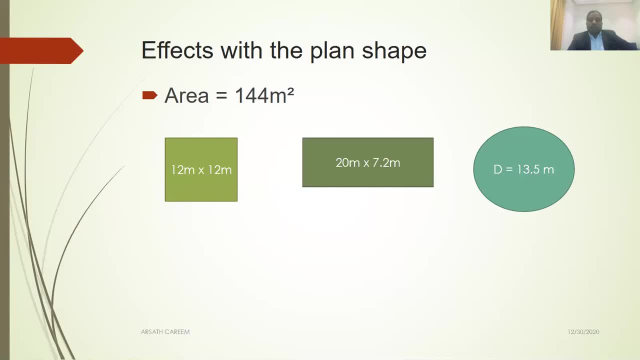 just just to attract the tourists or the people pride purpose. but what we are discussing here is the economy of the building. so economical shape is square shape. why it's? it's easy for natural ventilation. it has less perimeter compared to rectangular when, when it has less perimeter, the length 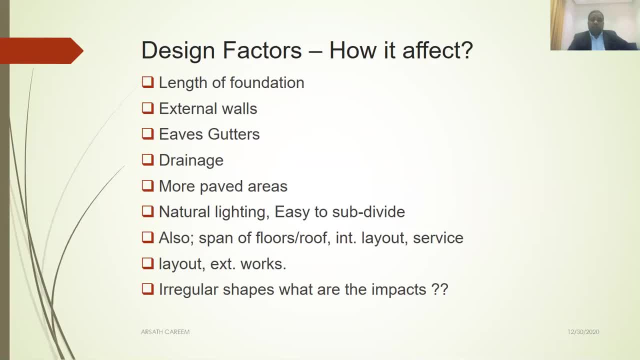 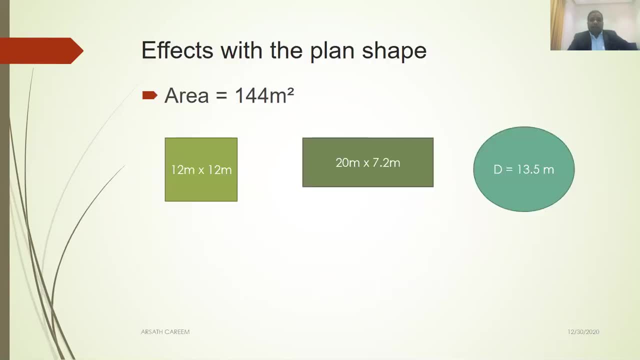 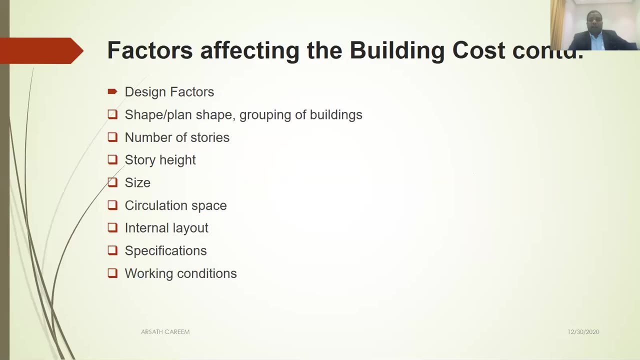 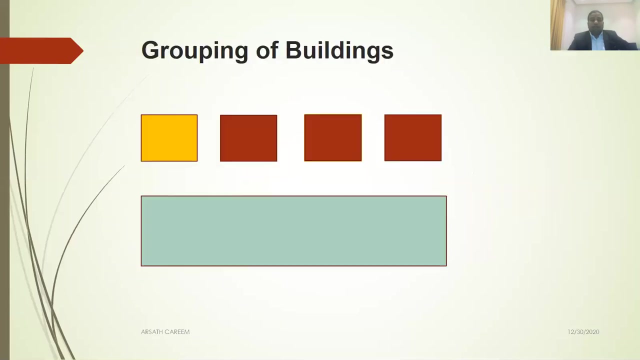 of the foundation will be less, external walls will be less. also, drainage will be less. so this is the reason. design factor- the first one share plan- definitely will- will impact the cost of the building. second, the group of building. this is the group of building you want to build a this much of rectangular, big, let's say, school building. 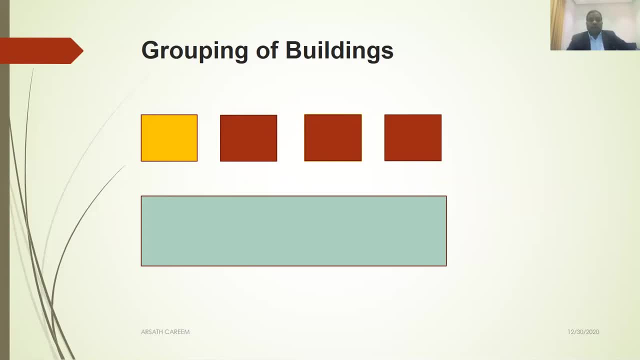 you can make it in one rectangular. also, you can make it same area by small classes. which one is economical? the rectangular one or square one? definitely it's a rectangular. why? because the different, different building will cost more, rather one one building. so these are the factors. the architect basically learn what we learning here. that just for. 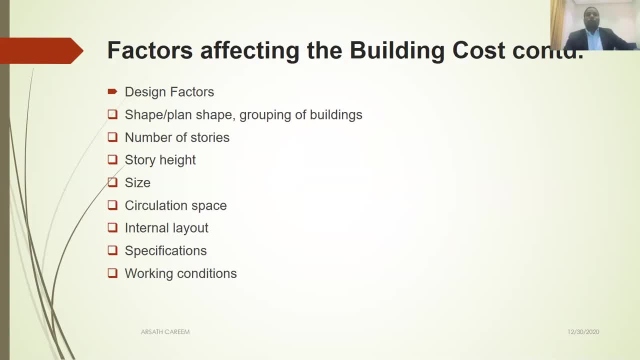 theoretical purpose. as a quantity surveyor you should know these things. also. the number of stories will definitely impact the cost. how, for example, you can't compare with one story building with 10 story building prices because one story usually within that area the cost per meter skirt definitely more compared to 5 or 10 story. because when the stories 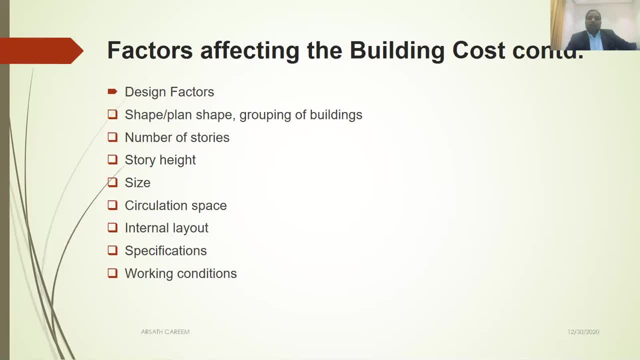 when the area is high there is a chance for less cat. also, story height: you can observe in the building. there are many types of building here. some building story height 3 meter, some are 2.8, some are 3.3, so you can't compare with. 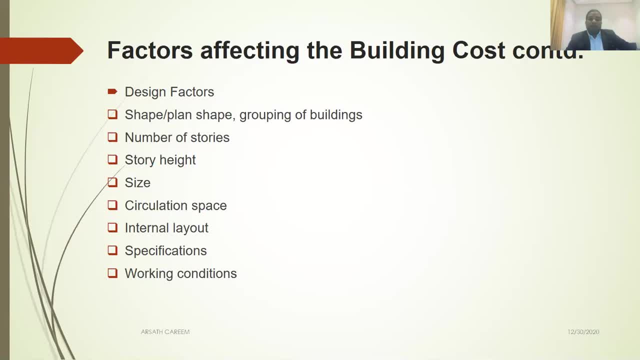 story height. with a different story height, you have to compare with same different same story height. also, size of the building definitely affect the cost. circulation space. what does mean circulation? circulation mean it's a people going through the general spaces which allocated, for example, staircase, lift passage, balcony. these are the. this is called. 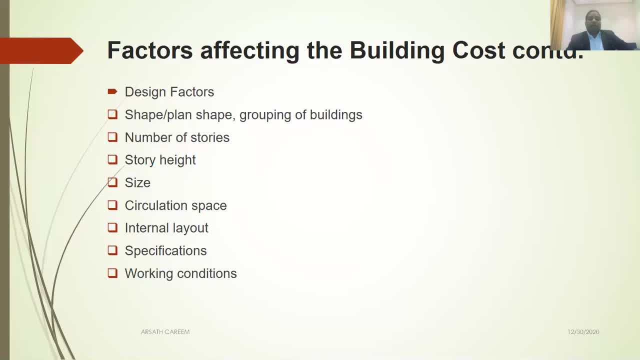 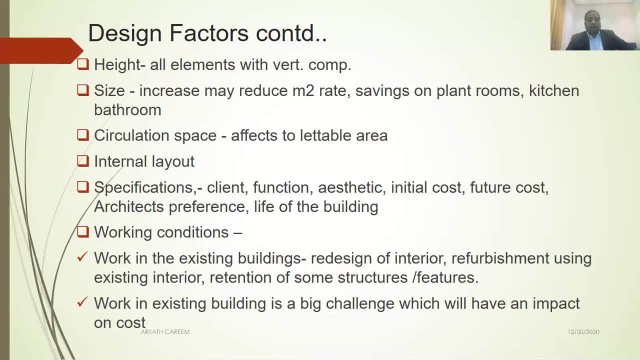 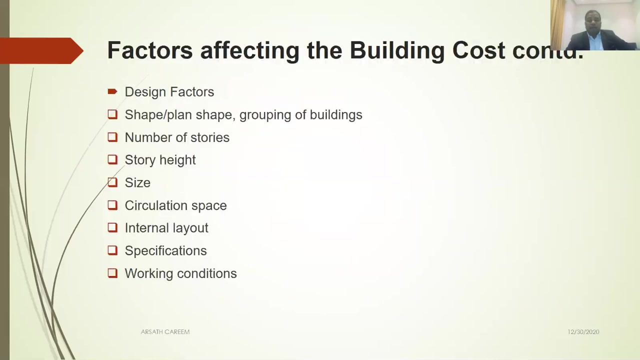 circulation. also, definitely internal layout will affect the cost and specification and working condition. when you check the working condition, working in the existing building different from working in the new building. so these are the main factors, design factors, which is affecting the building cost. these are just the theoretical part. there is nothing you have to think about it, just just. 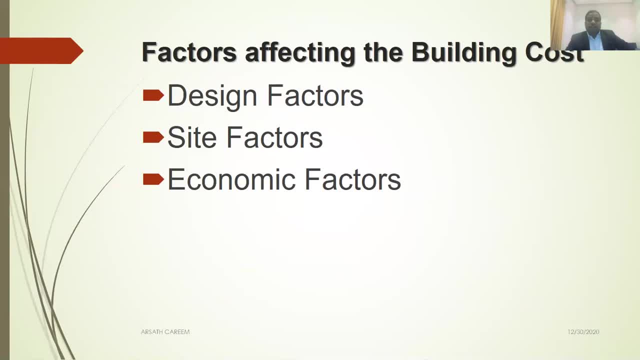 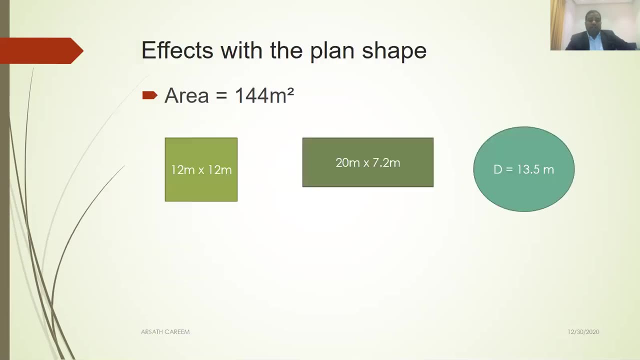 remember for your question. there might be a level one question on this one. just straight forward: what are the factors affecting the design building cost? you can answer directly: design factor, site factor, economic factor. when they ask what are the design factor, you can just list out to remember. i just make it understand by: 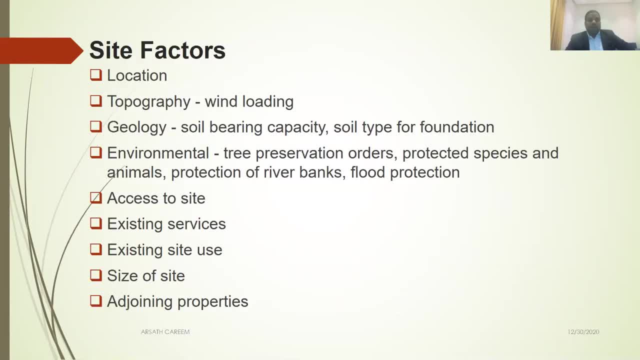 three through this picture. when you take the site factor. design factor, we already discussed. now, when you take the site factor, these are the main things. location, definitely the location is the major factor deciding the cost. for example, if you're building, if you are in sri lanka, if you, the cost of the building differ from capital. 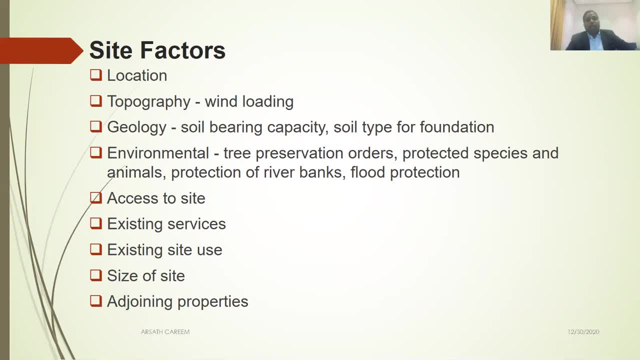 colombo to any other outstation, because mainly it's a transport cost. is the matter also the available labor resources, technology, these are the main things. also topography. topography also main factor deciding the cost, how, when you have a flat land, you you have a less. 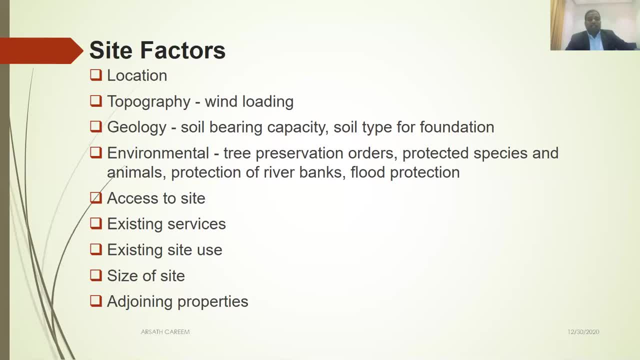 cost, why you can get the natural wind leaves easily. when you have a slope, your cost will be different. you can't compare with flat land building with slope land. so topography is the one of the main factor. also geology. geology, it's about the soil bearing capacity, soil type of foundation especially. there are many. 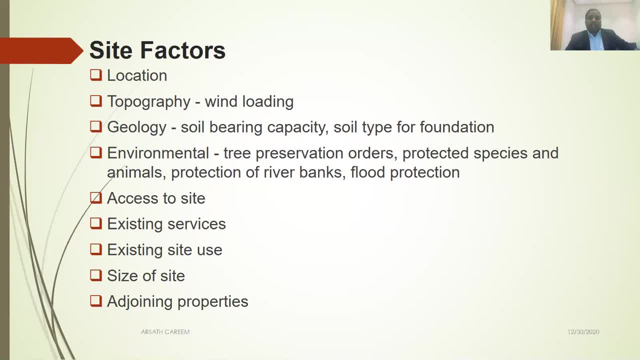 types of soils available. you can learn in the construction technology. depend on the soil type. the cost definitely will be varied. for example, if you want to build in this normal, normal land, sandy land, we compare with the muddy land, the muddy land that you have to improve your soil bearing capacity. you have to do some additional effort to make. 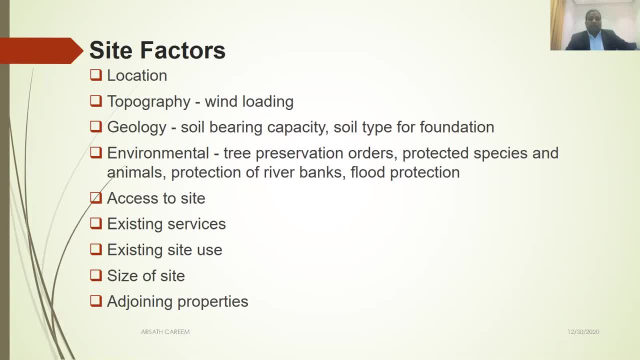 that length increase the bearing capacity. in this case geology, geology, also major factor, also environmental, environmental. for example, if you want to build a building near to riverbank or any flooding area or any near to forest, you have to consider the environmental factor. so in this case also the cost of the building is will be increased, also access to the site. 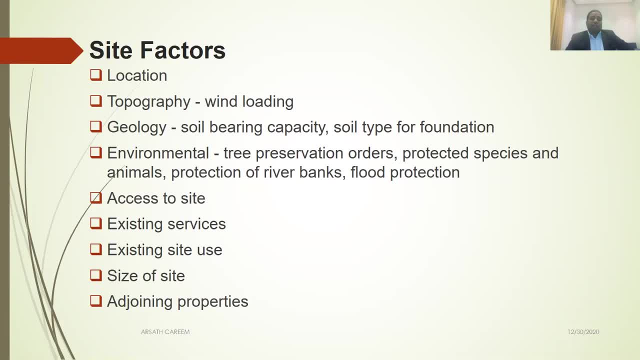 this is also one of the factor. for example, if you want to work in the restricted places, for example, army camp, or in- in perfect example in qatar is a barzan camp i used to work before- you have to get a special passes for that one. so, contractor, the time of the construction was a year. 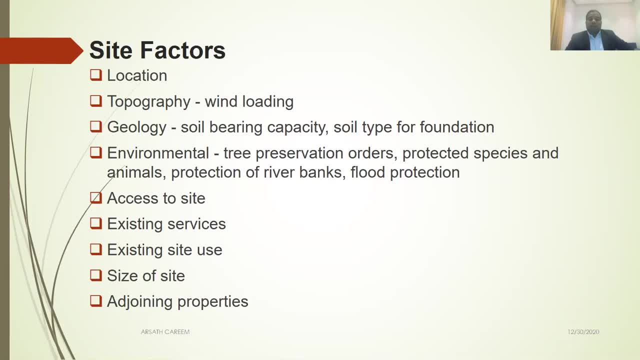 duration may increase because there is a lots of restriction, lot of security issues. this is the reason. access to the site, also one of the major factor. also existing services. for example, if you want to, nowadays in qatar, everywhere there is an underground train, metro train is there. so if you, if you want to build a building near to the near to the metro station, 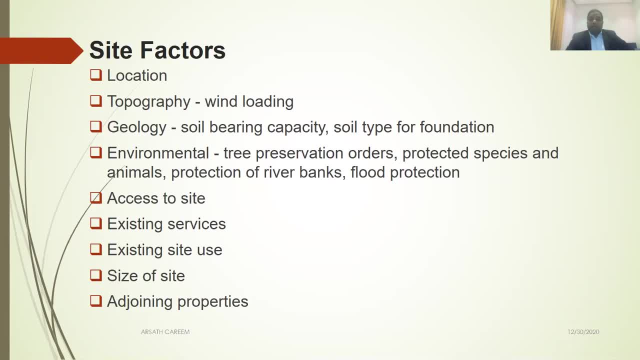 you have to spend additional money to take protection of the all the existing services, drainage line also, the metro line. you have to put additional protection also existing site use, the used site. also another factor: size of site adjoining properties. if you have adjoining properties you have to product them, their properties as well. so this is also one of 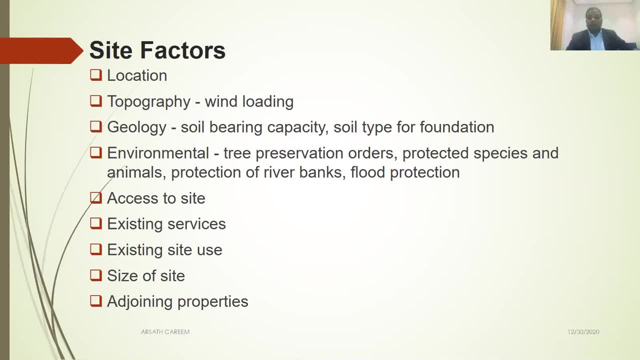 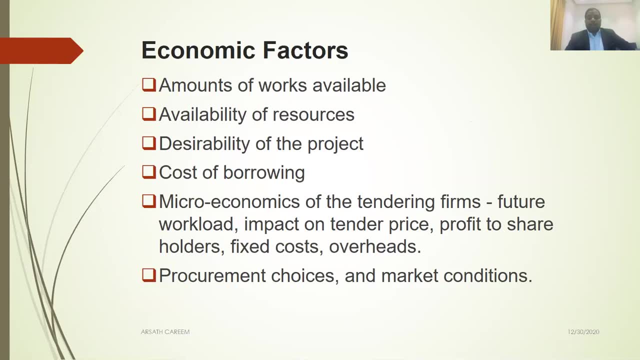 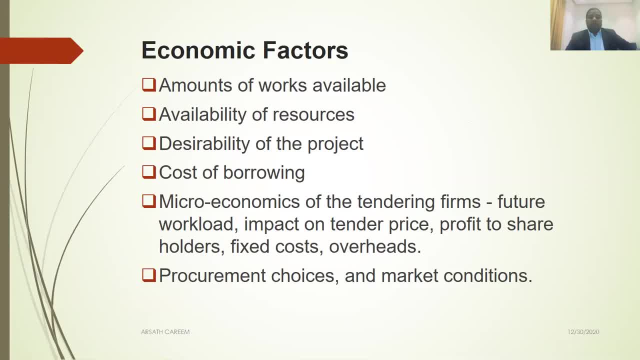 as you all know that if you want to build a small building, if you want to build a big, large quantity, it's a big building. definitely there is an impact on cost per meter, per meter square. when there is a more quantity, there is always chance for a less cost also. 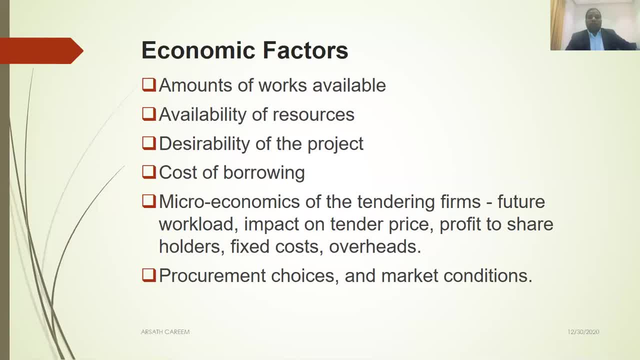 availability of resources. this is the major issue in, especially in qatar- lack of labor resources nowadays due to the covet pandemic, maybe everywhere in the middle east due to travel restriction. when there is a non-availability of resources, definitely the cost will go high. so this is also one of the factors for the cost of building. so this is a desirability of the project. 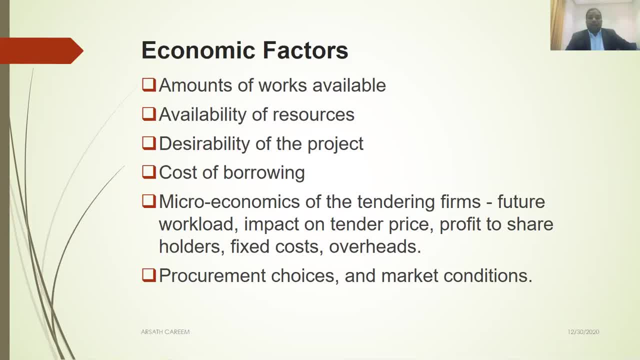 some client they, they won't, they don't care about the cost, just they want to build it. so this the desirability, so this is also one of the factor for the. this building cost. cost of borrowing. this is from the bank. some client get the, so in the construction cost the interest rate also will be added. when you compare with the. 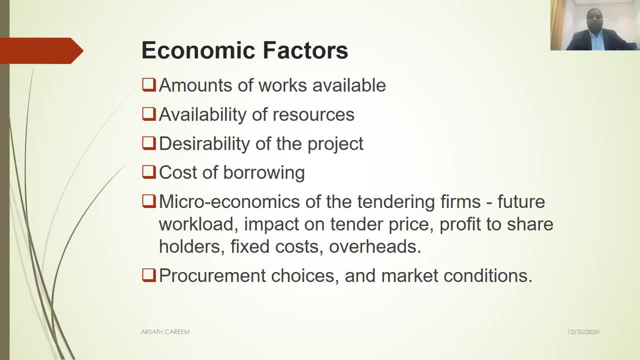 client. he has already money on himself so he can invest easily. so this cost of borrowing also one of the factor microeconomics of the tendering firms. some construction firms depend on the workload impact on the tender price. fixed cost overhead is also deciding the cost of the building. 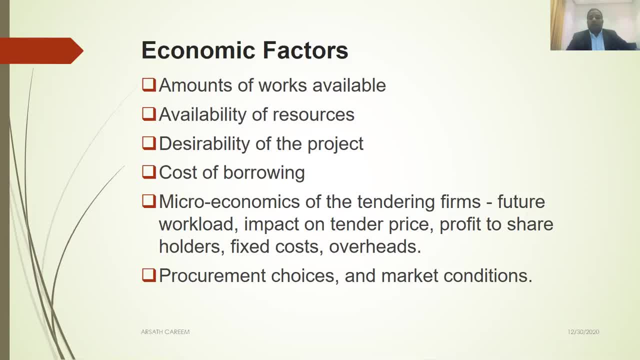 finally, the procurement choices and market condition, also one of the key factor currently the currently due to covet pandemic, the market condition badly affected in terms of traveling and the supply chain especially affected, labor forces especially affected. so these all these all factor which are deciding the cost. 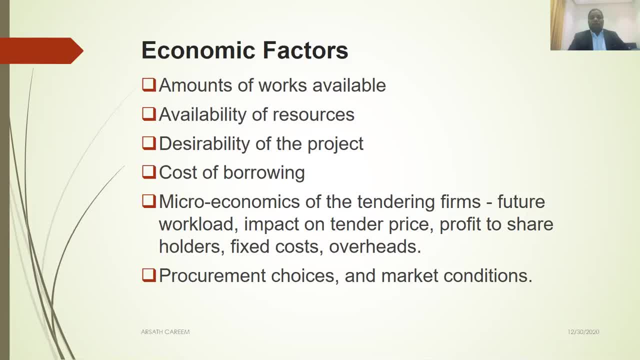 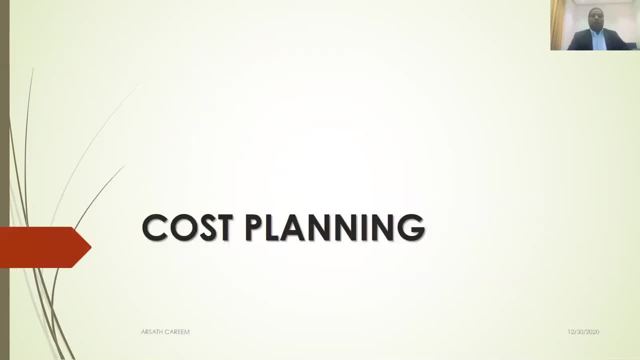 of the building as a quantity surveyor, who who are costing the building, should know these conditions. okay, now we need to finish our first part of this presentation, just just a theoretical part. there won't be a no major question in rics panel, i hope, just a straightforward question. 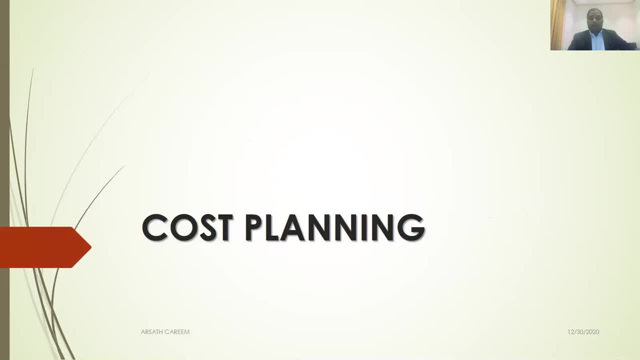 now we are moving to major part of today presentation, which is cost planning, which is the major mechanism, tools to control the cost during the construction process of a building in the pre-contract basis. as you all know, construction is a expensive process. it's consumed a lot of time and cost. 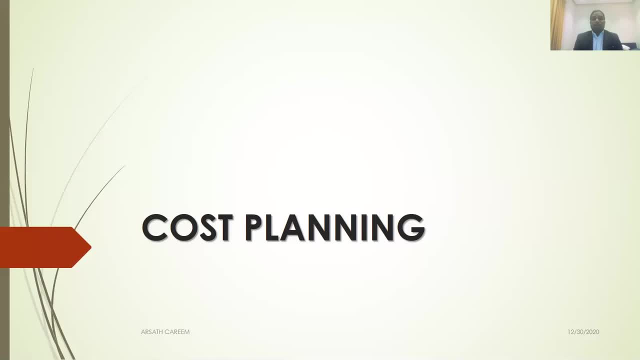 the major part of decision to build is a cost. therefore you have to check the cost first before you go into the project. for example, if you want to buy a phone, what you will do generally first you will check what are the features available, how much is cost any alternative model available to choose the phone. so just for buying phone. 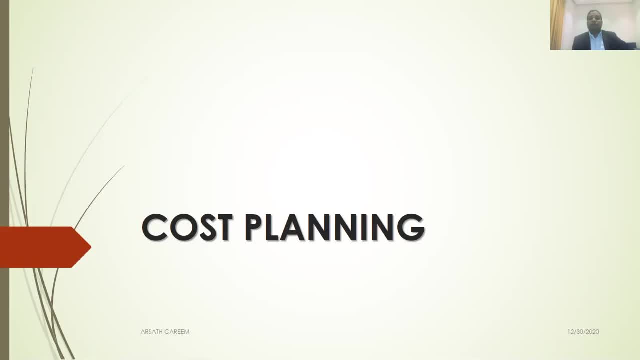 you are. you making many plans, you are planning your cost, you checking the features, think about the construction. it's a long process. it involves a lot of parties, lot of different parties, so you have to think carefully before you into the contract. first course, planning is about forecasting the cost: how much it's going to be. 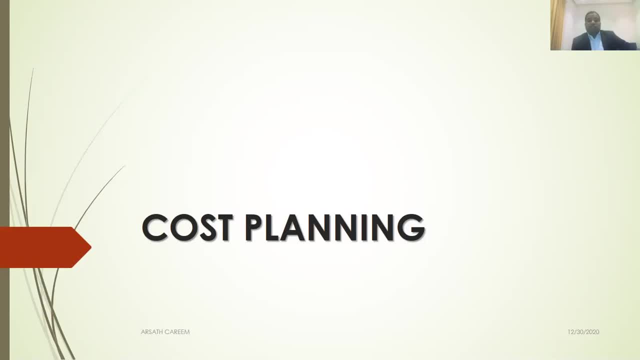 whatever reason, when you enter into the project, it's always is a business decision. what it is, what? what does mean business decision? for example, if a one client want to build a new plant to increase his productivity and compete with his competitor, or one consultant company need to build one head office for his staff to increase his imagination, pride, business opportunities. 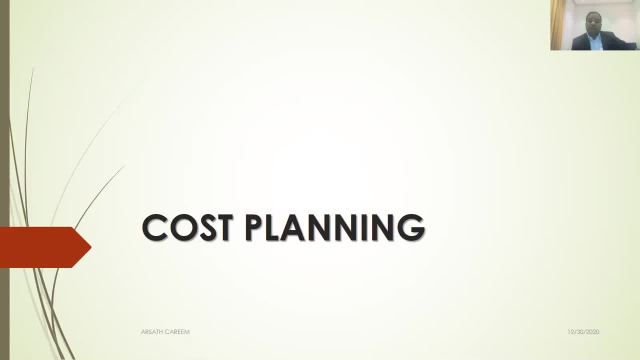 giving a lot of money to the client, comfortable to his staff. also, if you want to build a house, you want to check how much will cost. you want to provide more comfortable for your family, more facilities to a family. also, if a government want to build a highway to reduce the congestion, 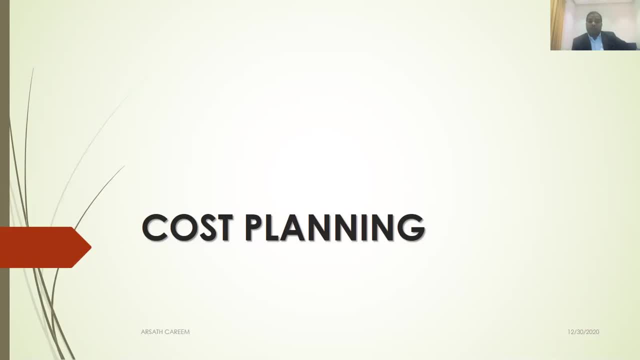 also improve the economy, reduce the maintenance cost. so everything you before you involve, you want to know how much would be cost, because everything is a business decision. you want to. you want to invest lots of money on here. you have to make sure your investment, the profitability you you have a. 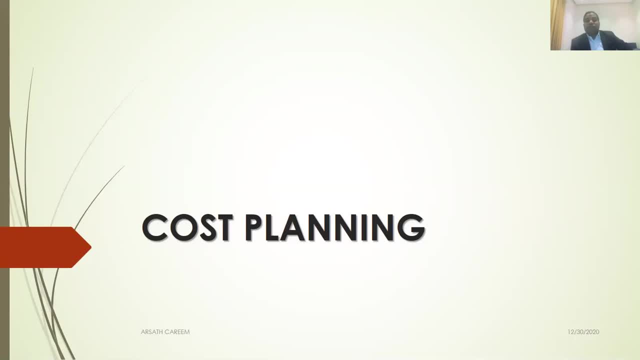 future for yourself, for on this investment. so in construction, we have a tool to identify, before you starting the project, whether it's feasible or not. whether it is, it is more feasible, more profitable, more convenient to your company. so you have to make sure everything depend on money you you have. 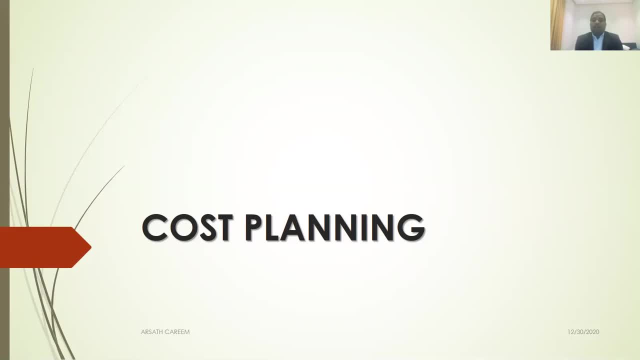 you have some. the money is not easily available on this world, so you have to make sure the money is available with you. so that's that's what reason cost planning take place in contraction in pre contract stage. so we will next slides we will discuss one by one. it's our ICS, a PC. 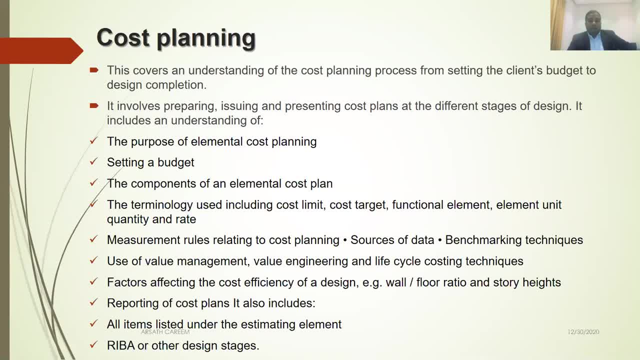 pathway guide listed followings what. these are the things you should know once you, if you want to pass this competency, you should cover about cost planning. following. you have to understand what is cost planning during the contract: pre contract basis up to design completion. it involved preparing, issuing and presenting. was planned at the different stage of design. it includes: 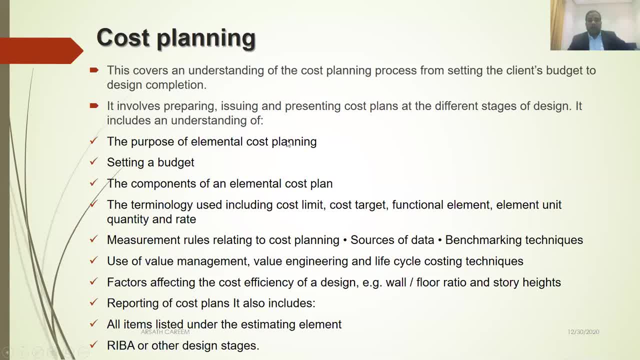 understanding of purpose of elemental cost planning. what purpose you prepare elemental planning? how to setting a budget. the components of elemental cost plan. the terminology used, including cost limit, cost target, functional element, element unit, quantity and rate measurement. rules related to cost planning. source of data: benchmarking technique. 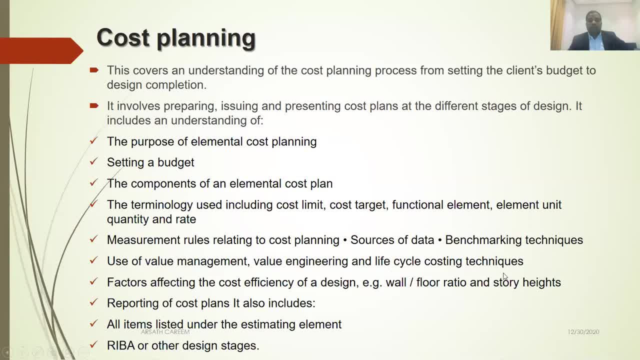 use of value management, value engineering, life cycle, life cycle costing techniques, factors affecting the cost efficiency of design reporting. of course, plan it's also include what are the elements under the costed cost plan and RIBA design stages. so during this presentation I will cover these all topics. 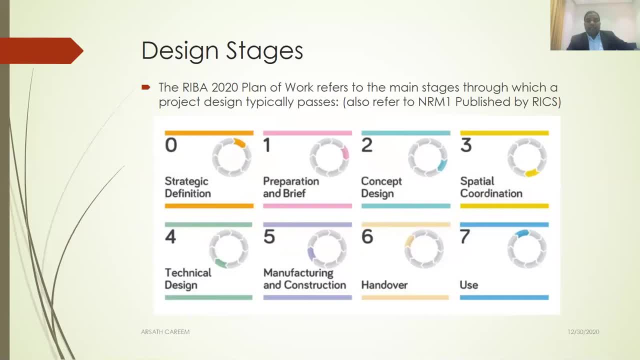 these are the design stages which is defined by RIBA, which is called royal institute British architect. these are the architectural firm, like RICS for quantityуля- this is for architecture architect organization which is providing guidance for architect. so RICS is also coordinating with them to define the 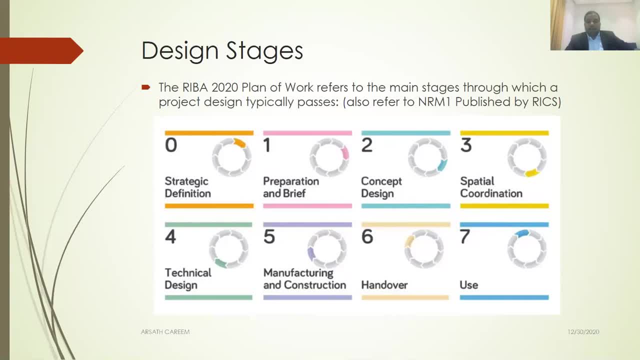 key needs to are then using these services at scale. as the critical note around the TJIC, these design stages- These are recently updated RIBA design stages. For the interview purpose, you have to know what are the stages. These are the eight stages, which are defined by: 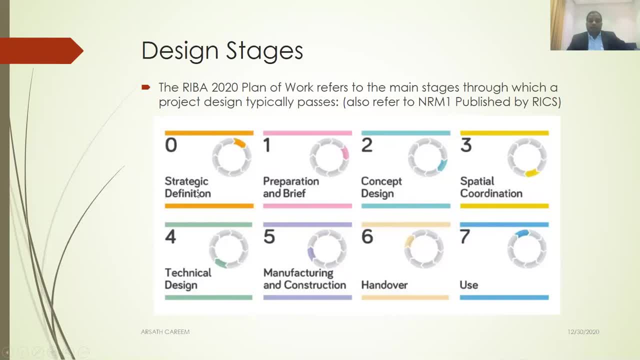 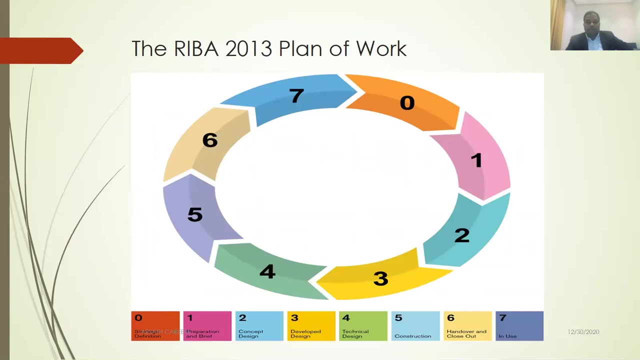 RIBA: Start with strategic definition, preparation and brief concept design, spatial coordination, technical design, manufacturing and construction handover, use Before 2020 introduced. this was their plan of work. They regularly update the plan of work. This is also eight stages. 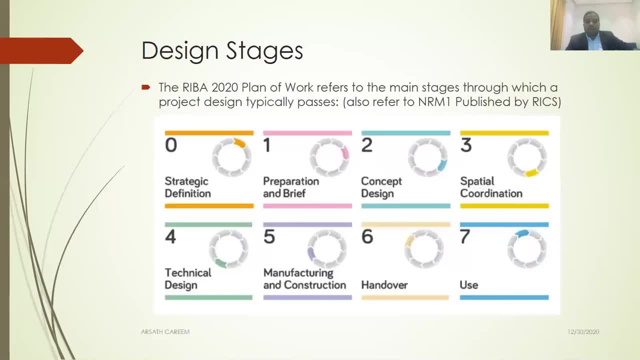 The only changes. number four: technical design, Sorry. number three: develop design. Number five: it's become spatial coordination. So they just updated recently, 2020.. Before going for an interview, better you know the reason. update So the spatial coordination. 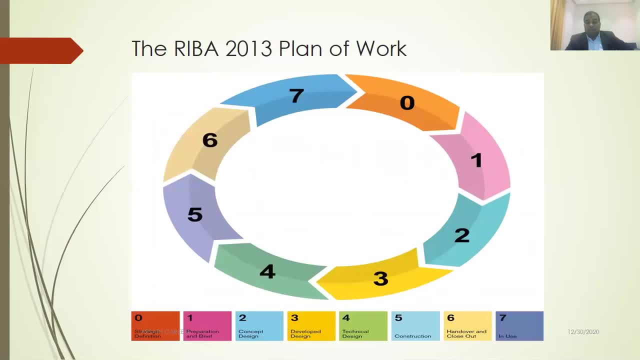 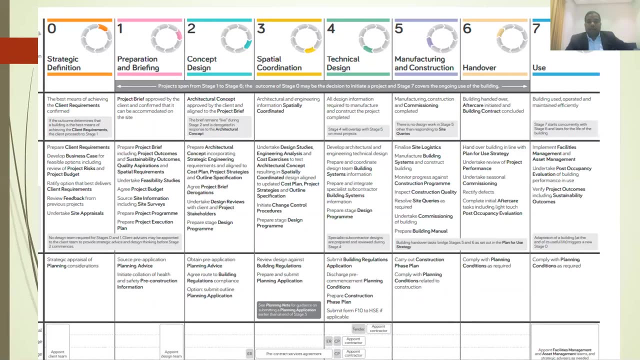 which is replaced with develop design. So every stage, these are the description they have updated in the website. Strategic definition: usually client identifies his requirements, Client requirements, whether he want to build a hotel, he want to build a hospital, he want to build a market, whatever. 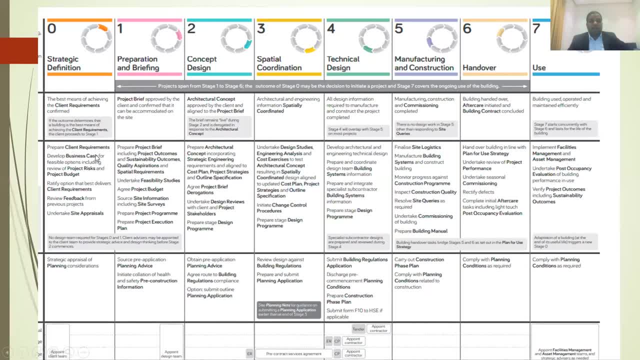 it is. This is the stage he identify his requirements and develop business case for feasible option. At this stage, roughly identify the project budget. It's a quantity severed, i will highlight. i will not go through detail because it's most related to all the professional 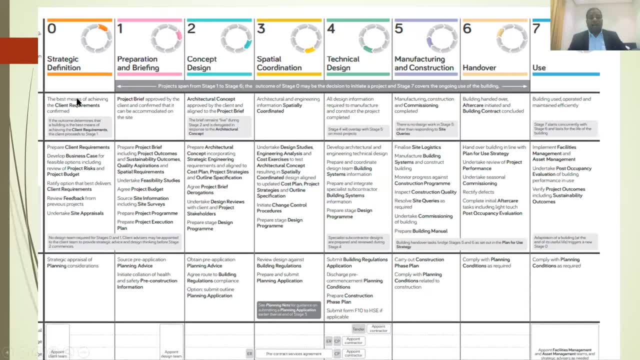 who involved in this process. i i will highlight just what quantity survey need in the zero strategic definition. once cleanse identify what he want to build, the project budget establish or it's a tentative budgeted stage, client say: i want to build within this budget or from his. 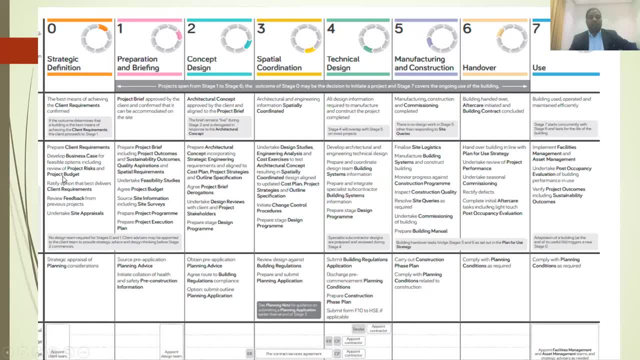 previous project experience. he say: i want to build this much. then preparation brief. from this stage it's developed a preparing brief outcome and project outcome: feasibility study. feasibility study undertake at this stage. whether this project is viable or is a feasible, it's a profitable. they decide at this stage. 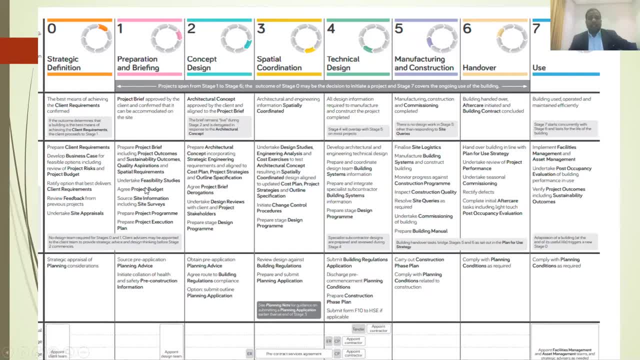 so at this stage they agree on project budget. once project budget agree, they go to concept stage. concept stage: the architect, different discipline architect. they develop the design based on the area, floor area, sketches, plans from that one, the quantity survey, prepare the initial cost plan. in the later stage we will, we will learn, we will discuss how to prepare a cost plan once it's. 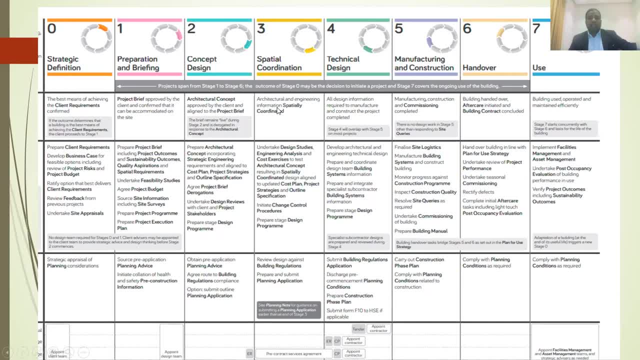 prepared cost plan, then it's, it's moved to a special, special coordination. at this stage also continue the post exercises. let's say, if it is a cost plan one, then at this stage we can say what's the cost plan two? so when the design develop, the cost plan also developed. so we have to compare. 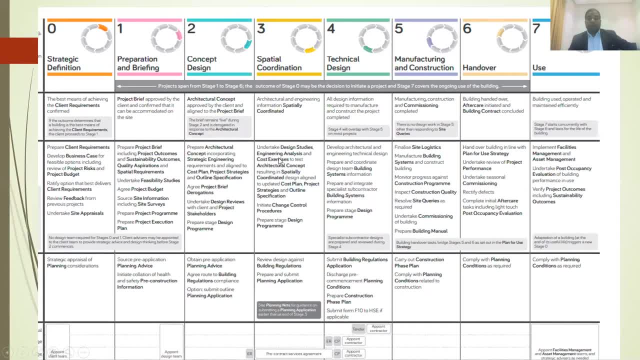 with cost plan. how much? what is the difference from initial budget to cost plan one, to cost plan two? these details, how to prepare a cost plan, uh, how? what are the things we have to look on this we will discuss in later slides. i just going briefly on this stage. then, once is the. 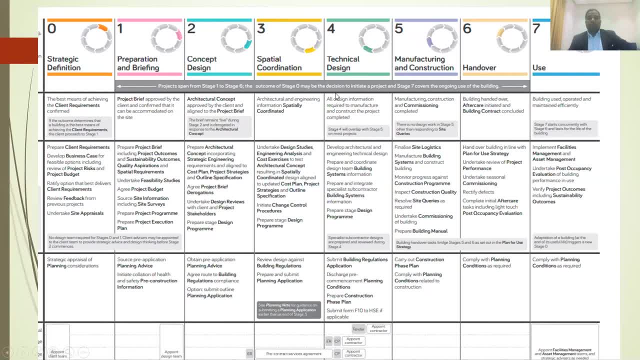 technical design develop. this is the tendering stage. you that all the drawings- construction drawings- completed. then you have to prepare the detail cost estimate. so these are the main stage of the design throughout the pre contract basis. this is defined by RIBA as part of the APC process. 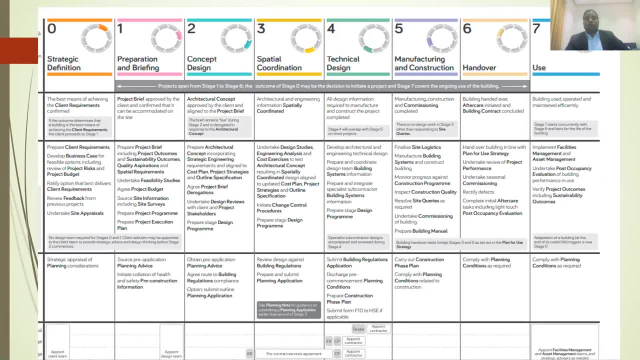 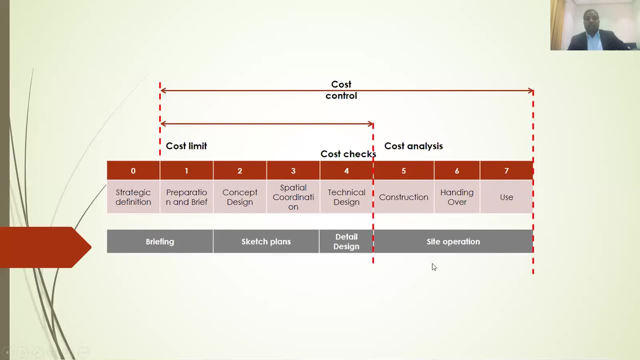 you should know these steps and your role as a quantity server: what should know, what should what, what you doing, how you advise your client. so these are the- I just summarize in perspective of quantity serving. these are the main stages. you have to set the cost limit here and you have 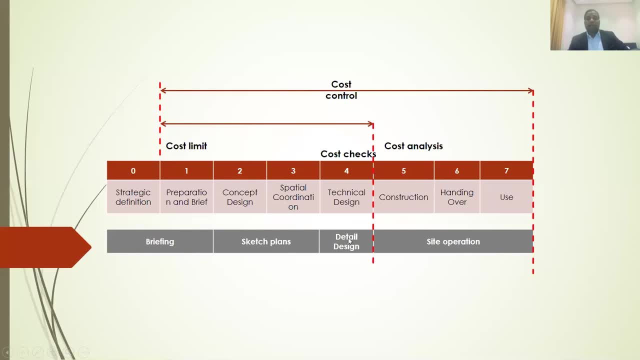 to continually do the cost, check up to technical design, up to tender stage and after the construction, this site operation. you have to analyze the cost, what you prepared before then, this whole process called as a cost control process throughout the life of the building, from preparation to use. so how to prepare these things? how? 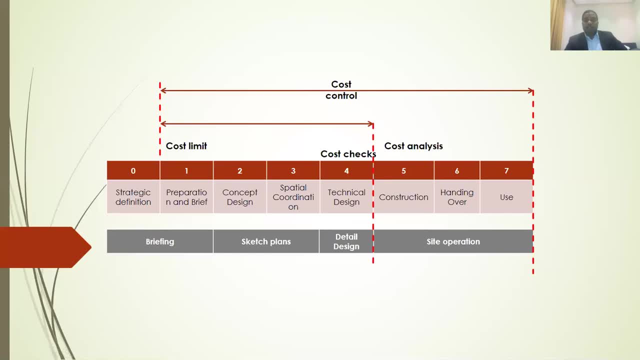 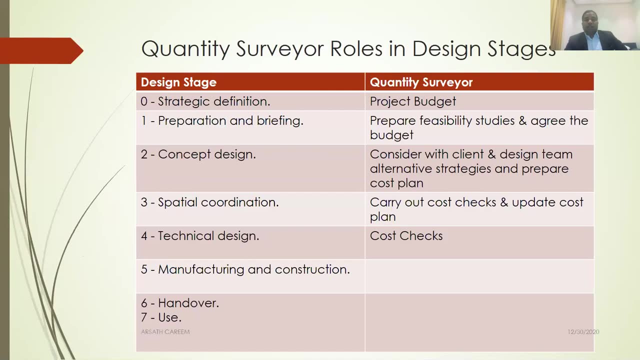 to prepare a cost analysis. how to set the limit, we will discuss in next slides as a quantity server during the design stage. what I discussed, I summarize here. what is your role here, you don't need to worry. what is written here, this is related to all discipline. I just summarized here. 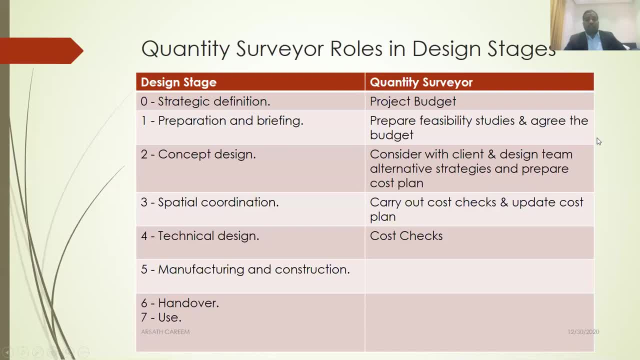 your role as a quantity server. starting definition: you should able to prepare a budget. how to prepare a budget, we will learn it later. preparation and briefing. how to prepare a feasibility study- usually this feasibility study prepared by consultant. however, you have to review and agree with the budget once it's concept design. you have to sit with the client and design team and you have to. 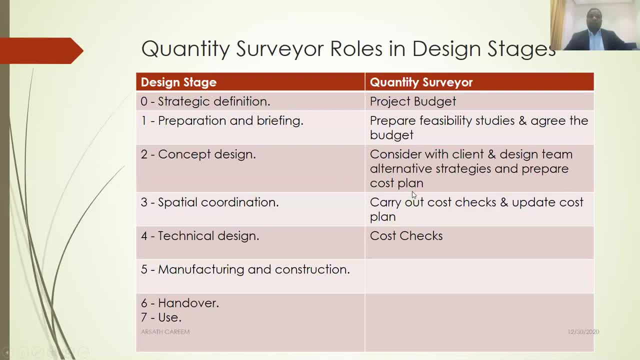 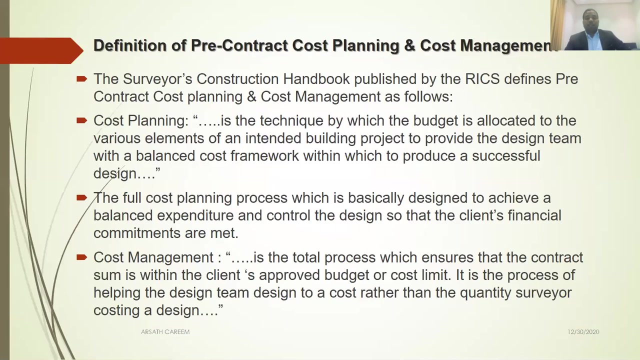 make sure everything is go as planned. then special coordination: you you have to carry out the cost check, update the cost check. and technical design: you have to do the cost check. what is cost check? we will see in the next slides. as per the rics handbooks, the cost planning is defined as a technique by which the total budget 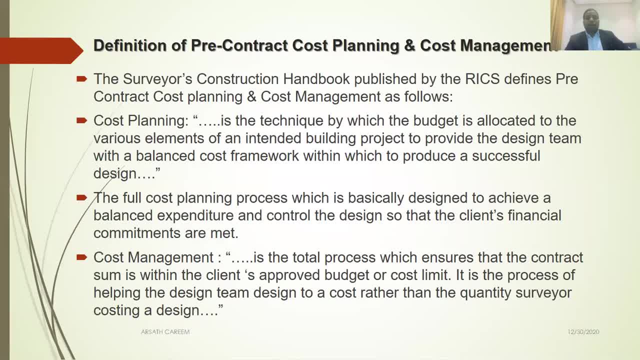 budget is allocated to the various elements of an intended building project to provide the design team with the balanced cost framework within which to produce a successful design cost planning. it's a simple word. you can say the forecasting, the building cost. but rics they define in the handbook is a technique. the budget allocated to the various 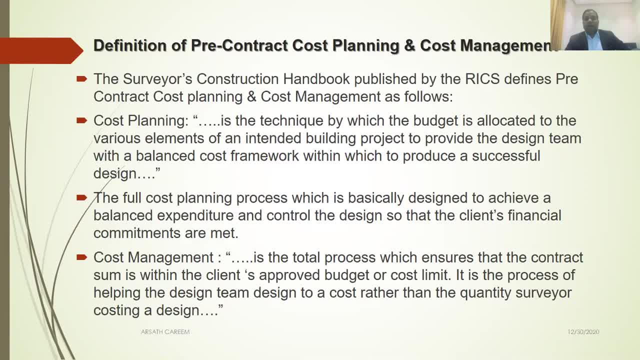 elements of the building. what are the elements you have according to the building function? we have a various elements, for example, substructure, superstructure finishes, mvp works, external work. so the these are the various elements. so the total cost limit allocated to different elements. so that is the planning of the cost. 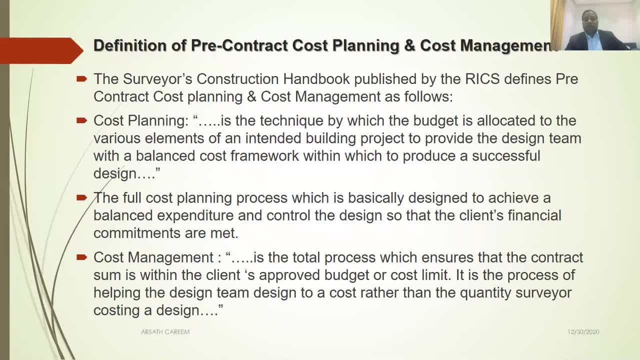 which help to produce a successful design. we will see in next slides detail about the cost planning. this just a definition which is provided by rics, the full cost planning process, which is basically designed to achieve a balanced expenditure and control the design so that the client financial 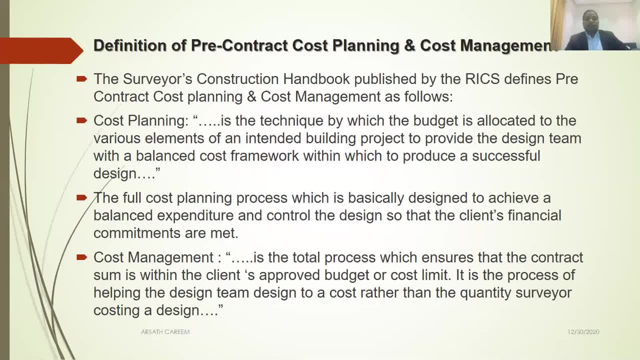 commitments are met. the cost planning used to control the design. how to control the design? because every client, every projects, they have a certain budget allocated. the this process, cost planning is make sure the design doesn't over budgeted. so every, every design process there is a check, cost checking process that will make sure. 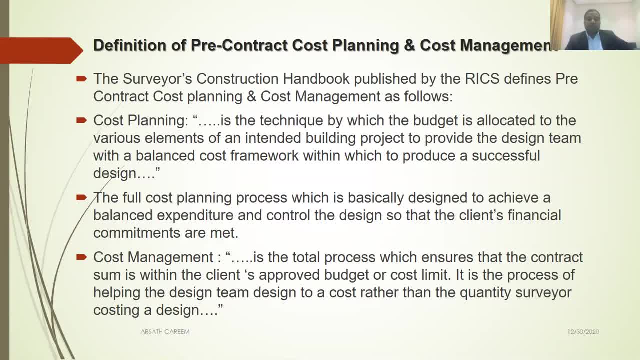 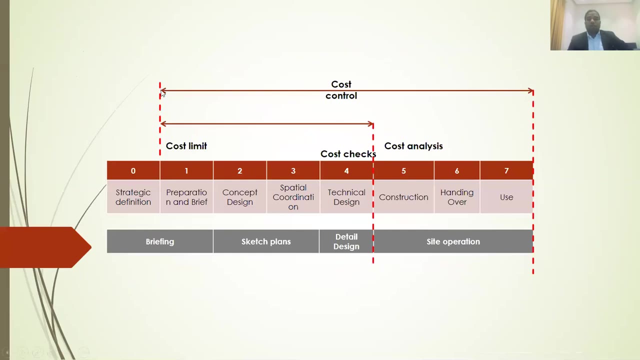 the project budget is within the allocated budget. also, rics handbook defined as a cost management. it is a total process which ensure that the contract sum within the client upward budget or cost limit. the total process which is called cost management. this one, the cost control or cost management from 127, all the process which is called cost. 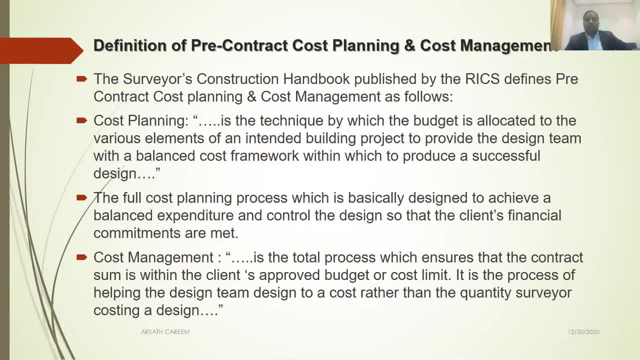 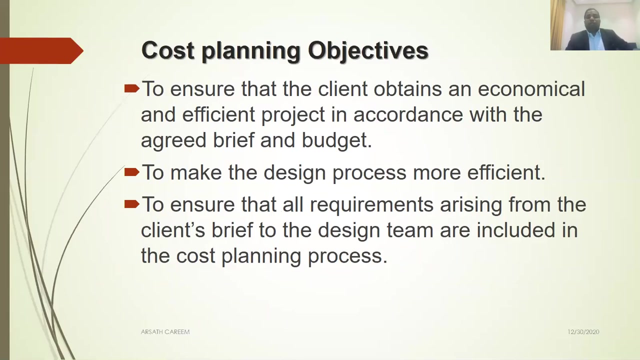 management. the main intention: the contract sum within the client approved budget. this is the the purpose of cost management. the contract sum is within the client approved budget or cost limit. so this is the reason this cost planning, cost management process established. this is the main objectives of the cost planning. these are the three objectives to ensure that the 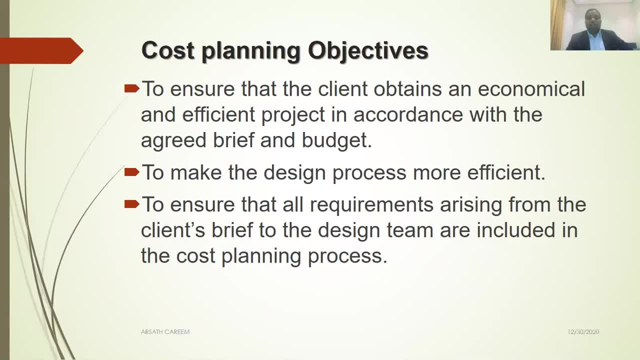 client obtains an economical and efficient project in accordance with the agreed brief and budget. so you, these are the first main objective. whatever it is, economical project, accordance with the agreed budget. this is the main objective. second, to make the design process more efficient. how design process can be more efficient? for example, 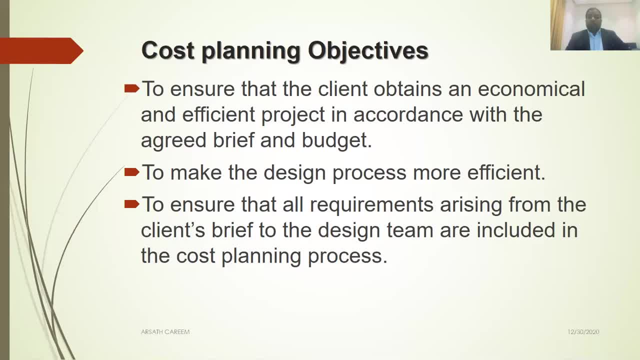 let's assume you don't have a cost planning process. you start the design process from concept design, then move into spatial coordination and technical design. after all design you check the project plan. so the present design and actual project will be different in the long run. the budget: sometimes it will be more than what you plan, sometimes it's a less so toward in order to 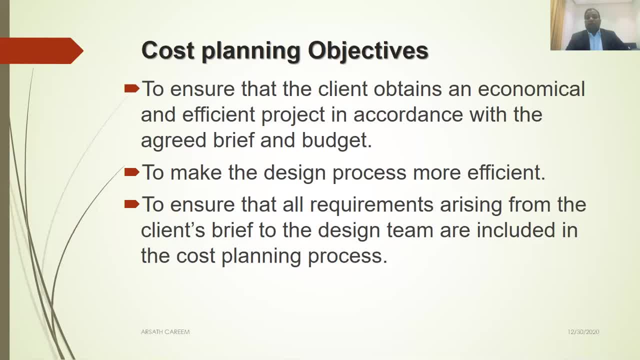 make a design efficient. for example, you don't do cost planning during the design process. what will happen then if that's what you develop during a design process? what will happen so, according to the? so you wasted a lot of about works, for example, consulting office. so this is the general principle. 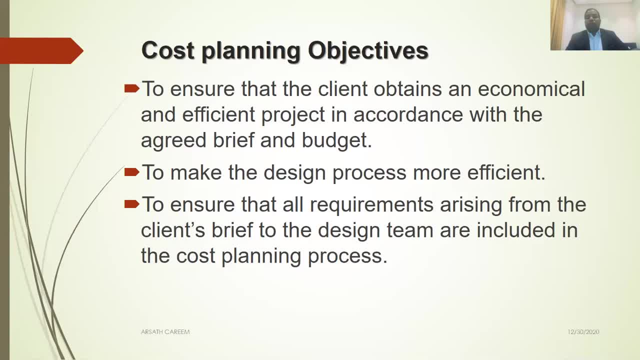 of the cost management in relation to this is where you can automatically use this profit-based concept design you. you didn't check spatial coordination, you didn't check. in the end, when you check, it is more than your budget, so you have to redesign your work within the budget. 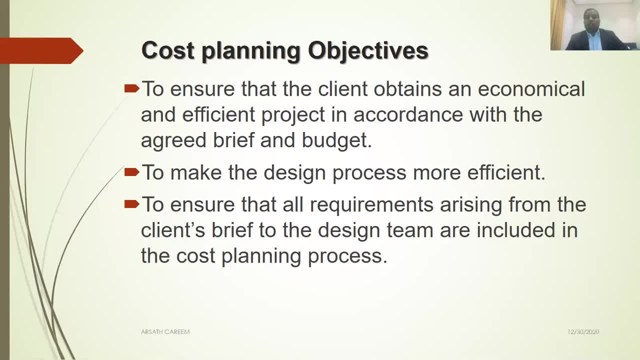 so the old, old worker. rework is about the work. so to make what, what course plan is doing, it make more efficient. so that is one of the key objective. so every stage when you do cost plan, cost check so you will know where is the problem, you can identify which area you have to reduce the cost. 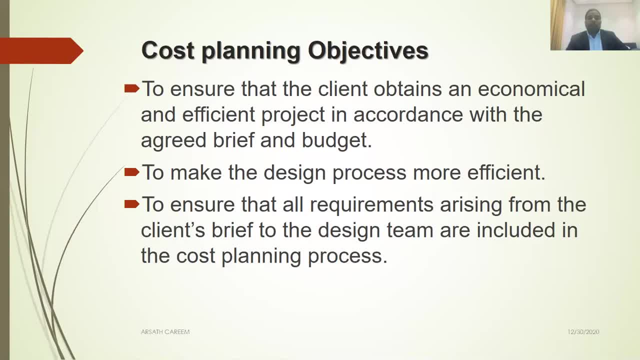 the third one to ensure that all requirements arising from the client brief to the design team are included in the cost planning process. so this is also one of the objective: to make sure every stage, when you check everything, when you do the cost check, when you do all the squabs, are included. 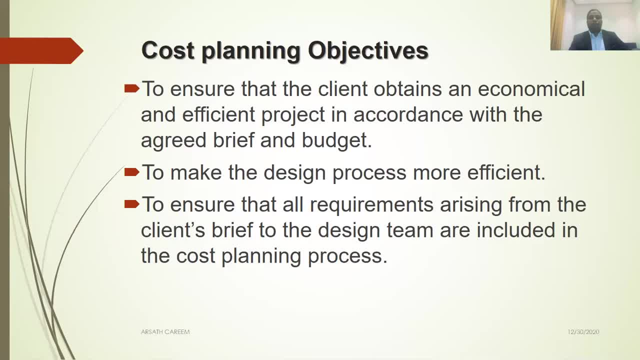 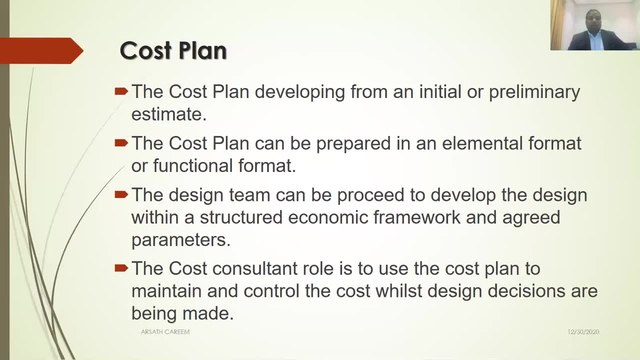 you will not fail to include any of client requirements. so through cost planning you can achieve these three objectives. further, cost plan is developing from initial preliminary estimate. so before cost plan you have to do preliminary estimate. so in construction you will learn later in the slides what are the preliminary. 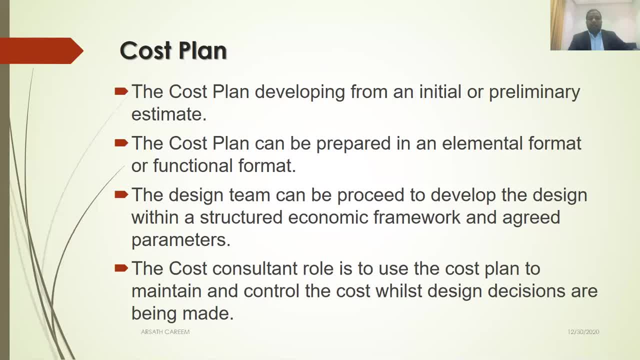 estimate methods available. so, cost plan for the cost plan, for the developing cost plan, you need, you need a preliminary estimate. you should know, as a qs, how to prepare a preliminary estimate. the cost plan can be prepared in element format. this is the standard as recommended by rics. 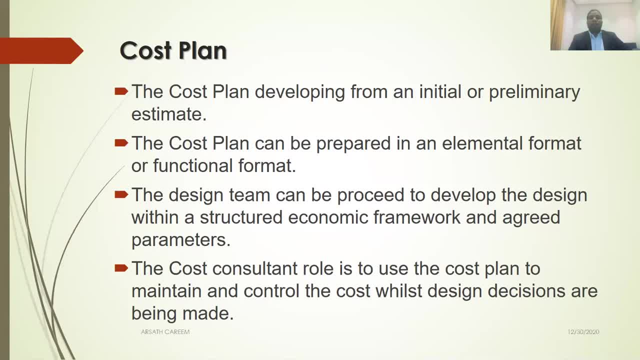 what are the elements? as i discussed before, substructure, superstructure, internal finishes, services, external work- these are the main elements of the building, so you have to use that element to prepare a course plan. the design team can be proceed to develop the design within a structured economic framework and agreed parameters. 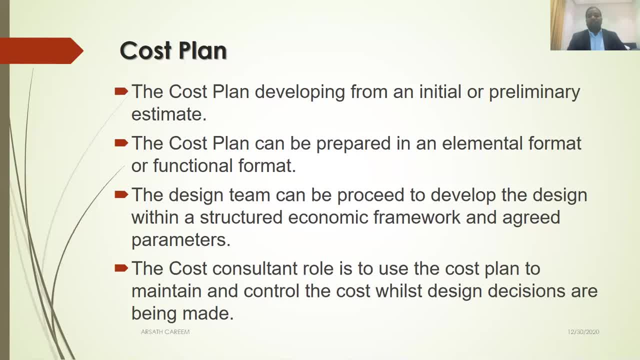 the cost plan of the project should be prepared in an agreement with the cost team, which is helping the design team also. the cost consultant role is to use the cost plan to maintain and control the cost while design decision are being made. so it's a cost consultant as a key was you had to maintain and control the 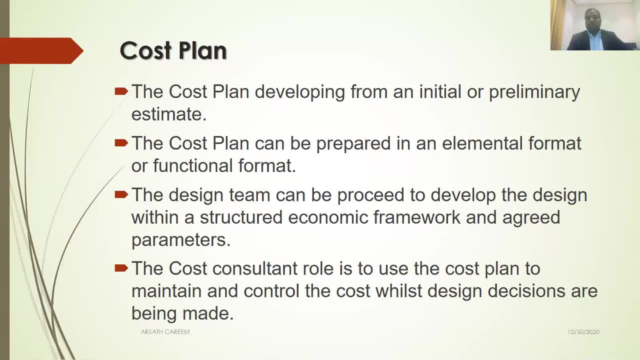 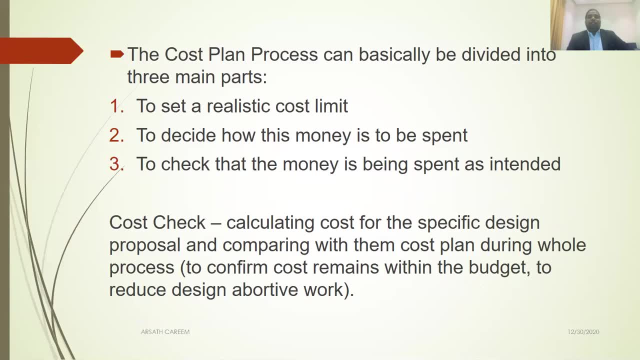 cost. so how we will do we will discuss in next slides. the process basically divided in three main parts. you have to prepare a cost plan. so how you will do that's all about here. it has three steps. first you have to set a realistic cost limit. what does mean realistic cost limit? cost limit mean is a budget first. 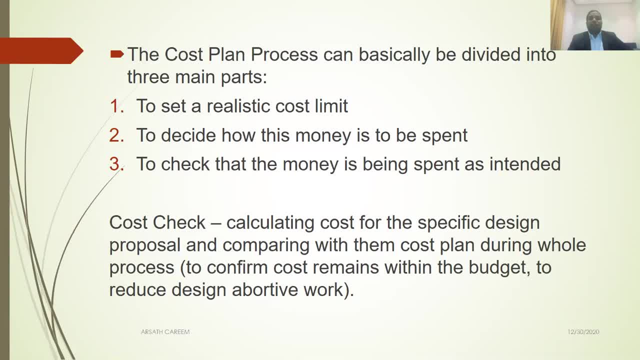 you have to set the realistic budget, rather than just for this one. the question is: does this cost limit mean that is it? so what I will do is I will. QS knowledge is very crucial. the experienced QS. He has to use the right project to decide. 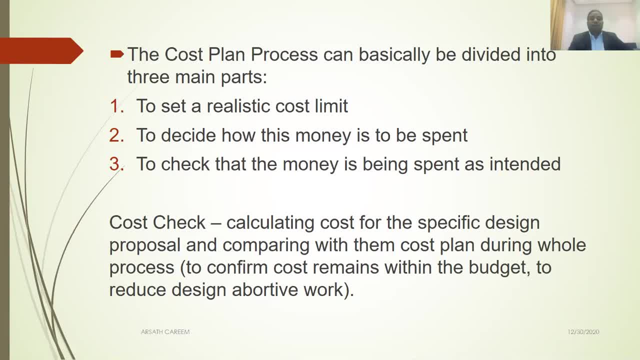 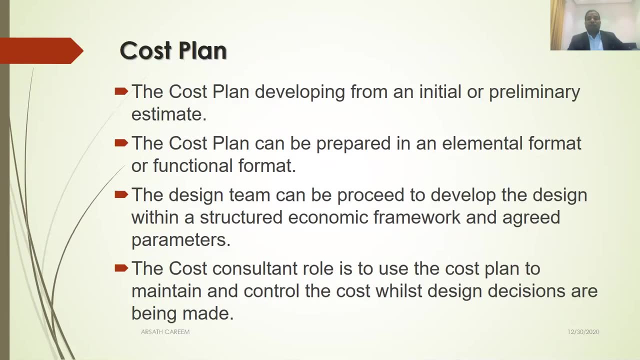 How he will decide, we will see. To decide how this money is to be spent, First you need to set the limit, then you have to decide how this money is spent. It means it's a cost target, As I discussed before. 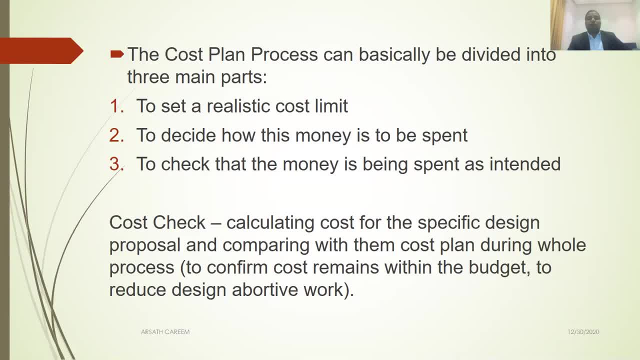 here you are using the elemental format, So you have budget divided, the budget propagation into elemental of the cost. For example, if you want to build a hospital, let's say 100 million, So that is the cost limit From using the preliminary estimate. 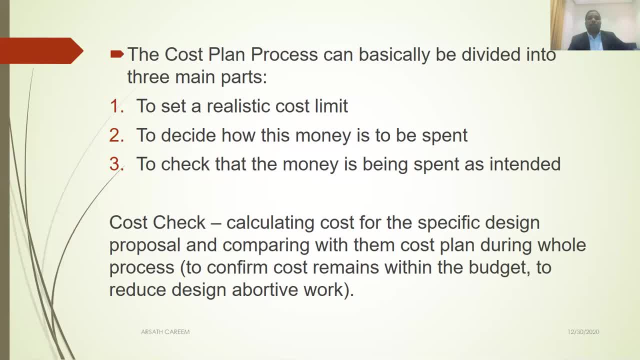 you identify. that is, your. 100 million is your budget. It's a cost limit. Now you have to decide how you are going to spend. For example, what are the main elements? you have? Substructure, superstructure, internal finishes, whatever it is. 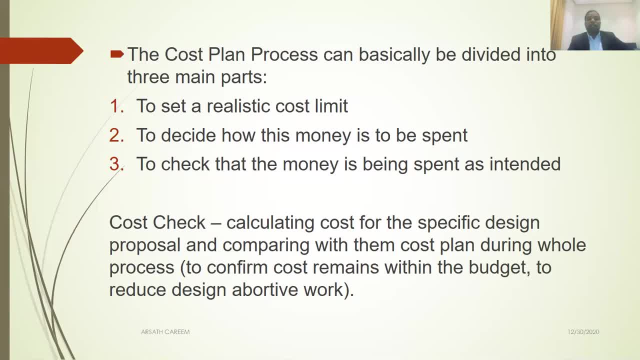 The list out: main structure 506.. Then you have to progression it. that cost 100 million. For example, substructure, you get 150,000, 15% Superstructure, 40% Services, 30% External work, 10%. 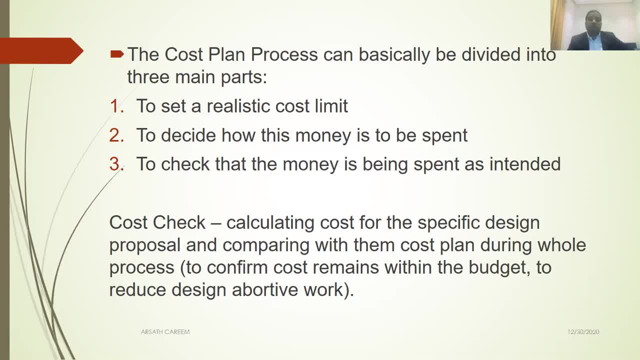 You have to use your experience on similar project. You have to progression it. That's what the second say. You have to decide how this money is going to be spent In the later. I will show one cost plan for you to understand easily. 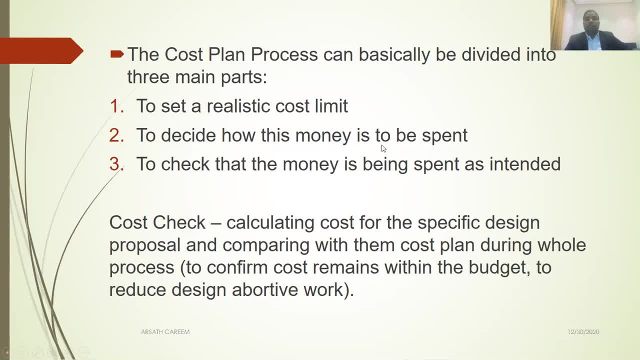 Third one, to check that the money is being spent as intended. This process called cost check. So you allocated each element some money. that is called cost target. So after design, develop, you have to check that one: whether the money is within your limit. 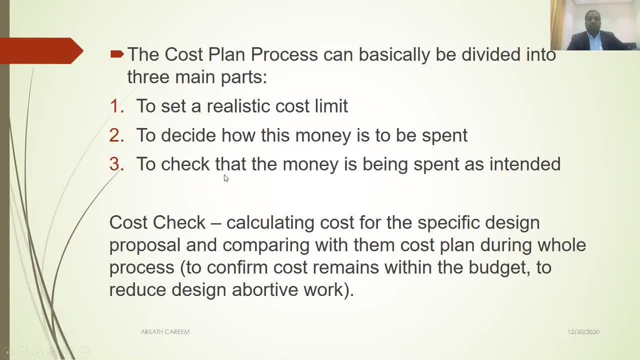 Calc. That's what I define here: cost check. The third process is cost check. This cost limit. Second, one cost target. Third, one cost check. What does mean cost check? Calculating cost for the specific design proposal and comparing with the cost plan during the whole process. 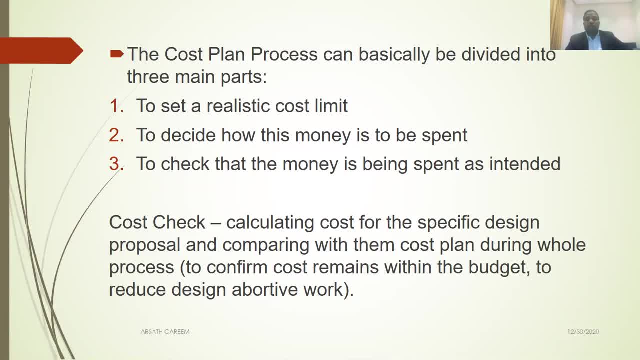 To confirm cost remains within the budget to reduce design about your work. This is the purpose of cost check: Mainly reduce the design about the work After design. you have to reduce the cost check After you full design if you come to know your budget is over. 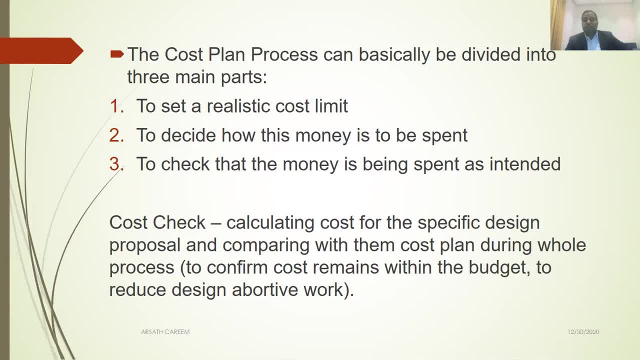 it's long process. You have to come back again. You have to start from the scratch, From every step of the design stage which I discussed earlier. if you do the cost check, you will save lots of time and your design will be more efficient. 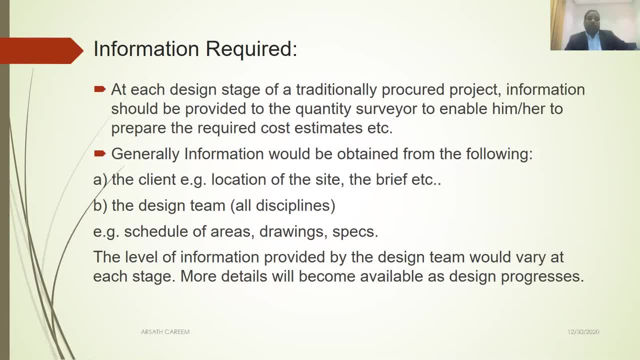 To prepare a cost plan. what are the information required? It's depend on the stage. At each design stage of traditionally procured project, information should be provided to the quantity server to enable him or her to prepare the required cost estimate. Generally following information: 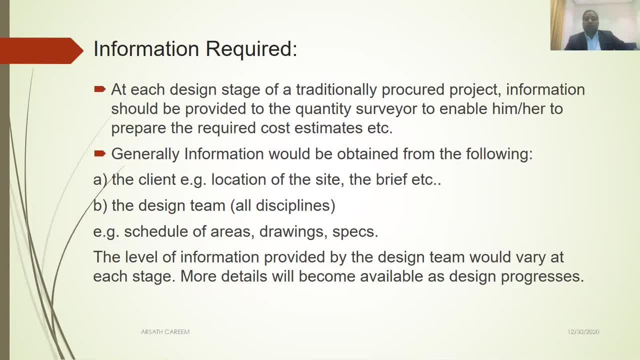 especially the client location site. the brief of the project. the design team schedule. area schedule of areas: ground floor: how much. first floor, how much? how much external work, also drawing specs. The level of information provided by the design team. 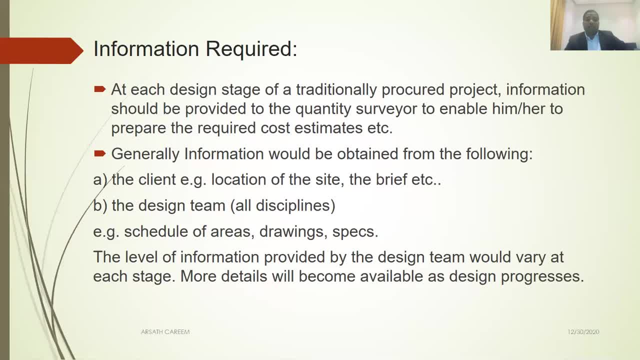 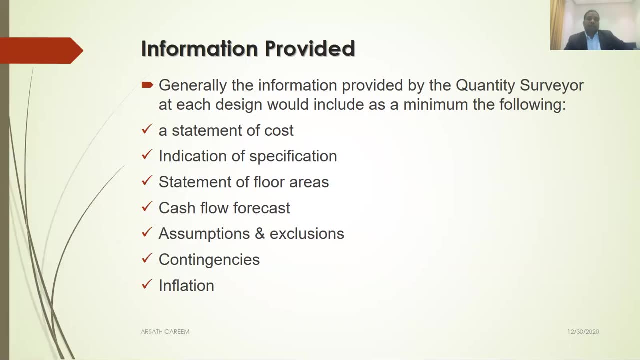 would vary at each stage. More details will become available at design progress. So to prepare an initial cost plan, these are the details you required. Once they provide the details, your job as a quantity server. you have to provide the cost plan. 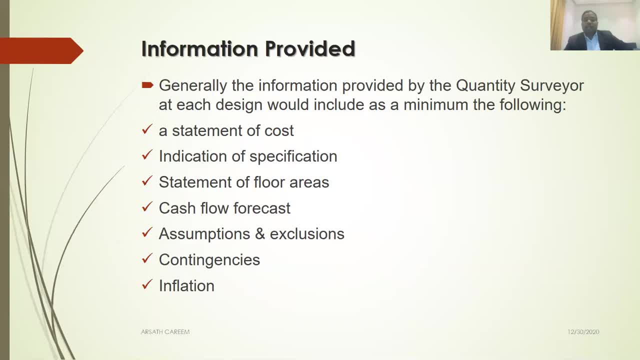 So generally in this slide, discussing when they give the information, client or design team, architect, give. what is your response? You have to provide a statement of a cost, Indication of specification, What level of specification you use. use the general quality or mid-end quality? 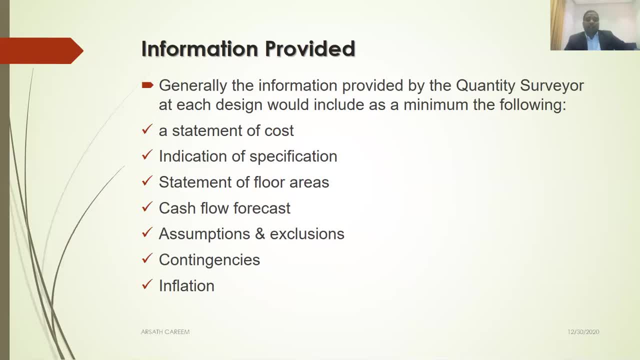 high-end quality statement of floor areas: each floor: how much cash flow forecast? this is very important cash flow forecast. this is one of the main benefits of cost plan cash flow. how? because now you know you need 100 million, for example, to build a hospital, you need 100 million. 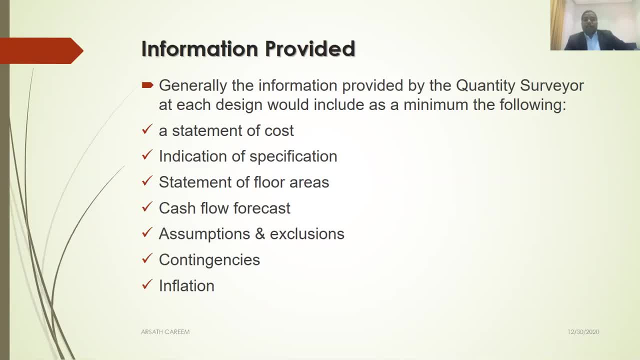 real, you need it. okay, as a client, i want to know when i need, how much i need. so this is very crucial: cash flow. if you don't give this cash flow, the client- for example, he, he, 100 million. sometimes he will get a loan from the bank: 100 million from initial stage. 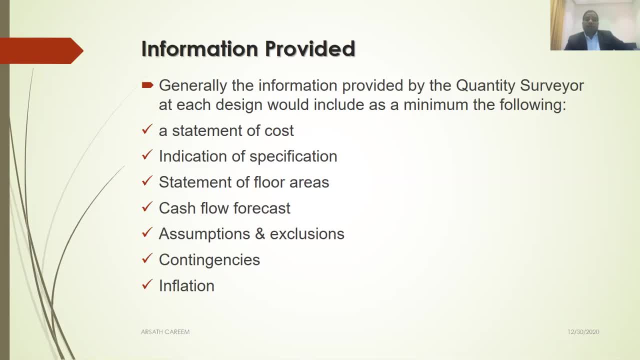 because construction is a progress. it's a long progress. start with every element, one by one. so when you provide the cash flow- for example, one year project you have- you should have a baseline program which month how much you needed. so when you give that information on your cost plan, 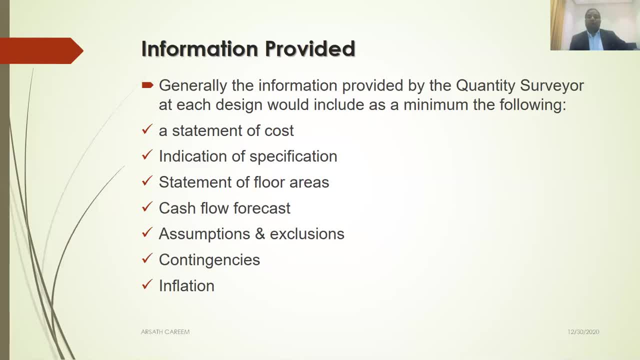 cost report, the client will know his commitment. accordingly, he can decide which month on how much he won, so he can save unnecessary interest. he need to pay for the banks most of the client. without banks is impossible to build a building. this is the current world scenario. whoever we want to build, they definitely 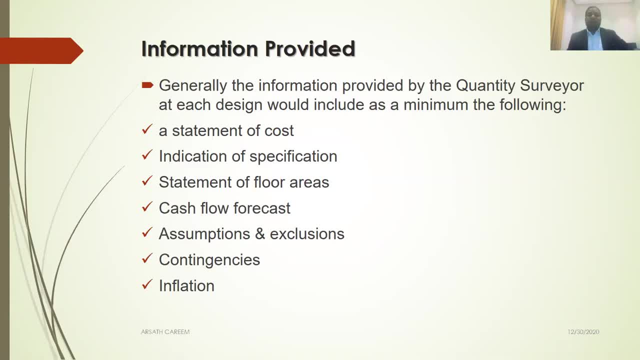 go for a even small loan, even the big client as well. also in the cost plan you have to give assumption exclusion. what are the assumptions? because you are doing the cost plan in early stages or that stage, there is not much available information. as a quantity server, you have to coordinate with the design team. 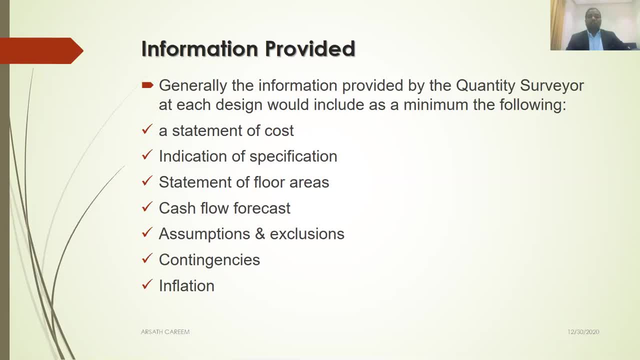 you need to make a lot of assumptions: sometime exclusion, time exclusion as well. sometimes your client doesn't include furniture work, furniture fit out work, sometime from some from the tenant. so depend on the nature of the project. you have to make those decision. those decision should be communicated in the cost report that should go to the client in future. 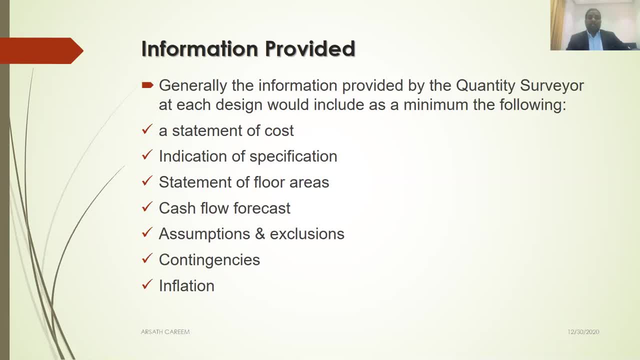 references also contingencies. what is contingencies? it's a unforeseen work, so normally in the cost plan we in general we allow. it's a trend, not compulsory, depend on the nature. sometime yellow 10 percentage- it is not a standard in my experience. usually we allow for contingencies, for example, design. 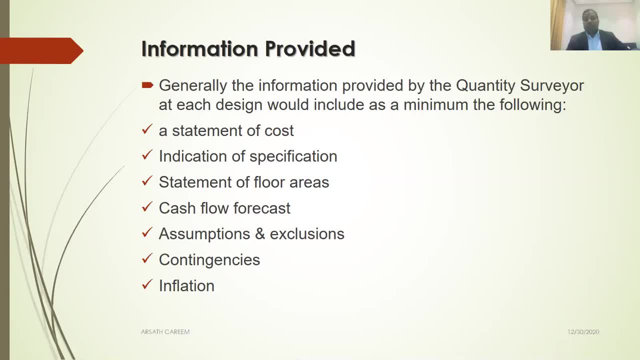 development risk. design development risk, sometime client changes risk, sometime unknown risk. we allow in case to avoid any additional budget required later stage. it is a risk risk elimination, risk management, including the contingents and inflation. you should know the current trend of the market condition. so inflation: you have to say in the cost report whether you consider the. 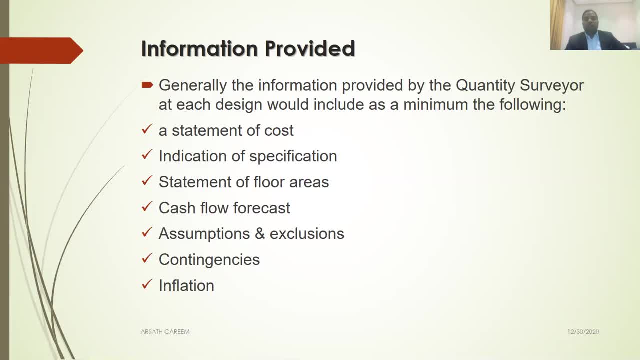 inflation, because you will do the cost plan this year. maybe you construct in next year. when you do costing here next year, maybe the major difference the cost may be the inflation will be high. the project prices will go high. that time you can met your budget. what do you? 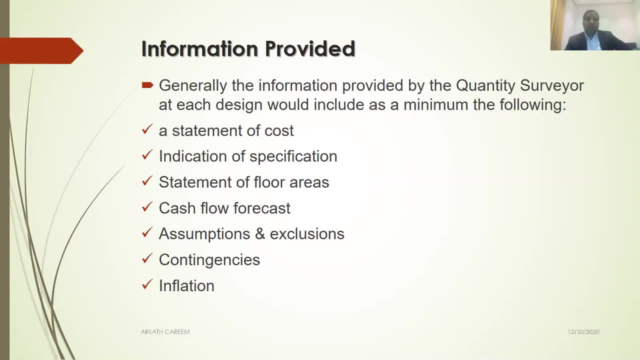 prepare. so you have to consider inflation as well. so when you give the when, when the client give this information as a quantity survey, you should prepare a cost plan according following, not limited to, but these are the main things you have to include. later stage, later slide, I will show you. 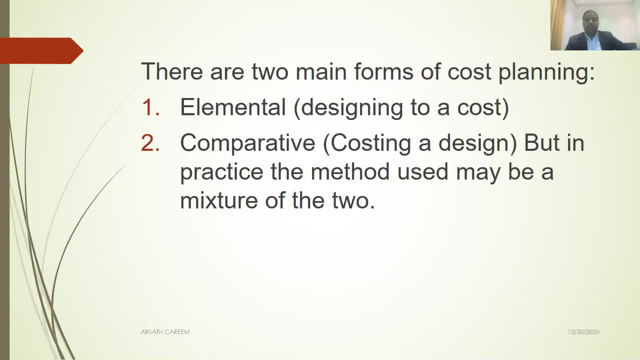 one cost plan for your reference generally. there are two things that you are going to be talking about today are two types of cost plan: one we called elemental and other one comparative. what does mean elemental? elemental is a designing to a cost, that the cost divided into the element of some. 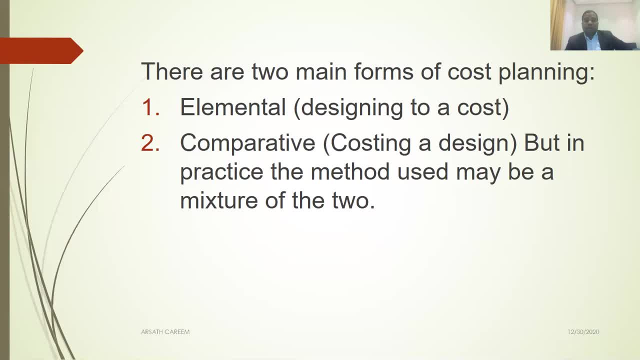 building. now that is the cost target as an architect. when, when you prepare an, the architect, that target, his aim should be the maximum budget. what you provided, for example, the same same scenario which we taken before: 100 million hospital project- we allocated substructure 15 percentage, 100 million, so 15 million that is the cost for architect. 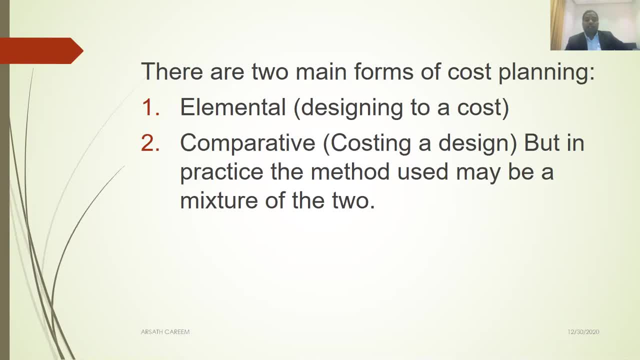 he need to make sure he designed that structural part, substructure part, within that one. that is called designing to a cost. is he always the structural engineer should aim to finish his design within that cost. that is the best practice. also, there is another cost planning method is comparative. this is called costing a design. this is just 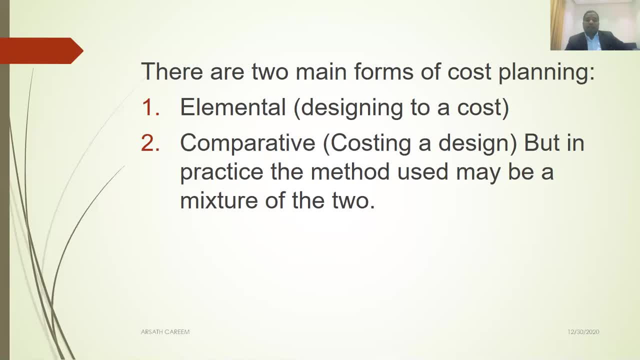 a costing a design. they normally the architect doesn't care about anything. he has a budget 100 million. what he do substructure, okay he, he designed a draft foundation. also, he designed a footing foundation for that particular building land. then the quantity server: what you need to. 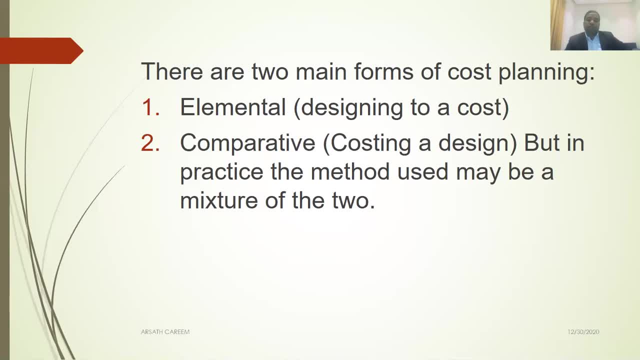 do you have to costing a design, you, you, you costing the footing, also, you costing the r rosetta. so you compare it which is better, so you compare it which is better. then you decide- this is called comparative, the first one designing to a cost, second, one costing a design. 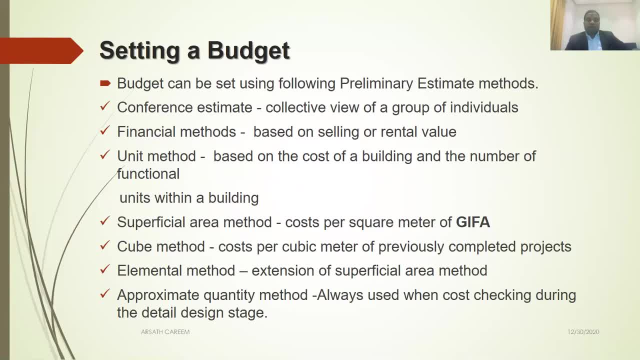 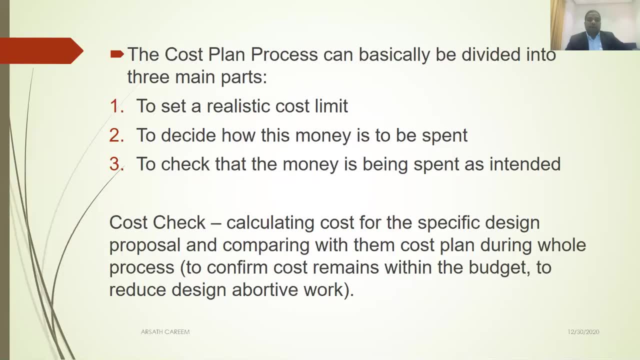 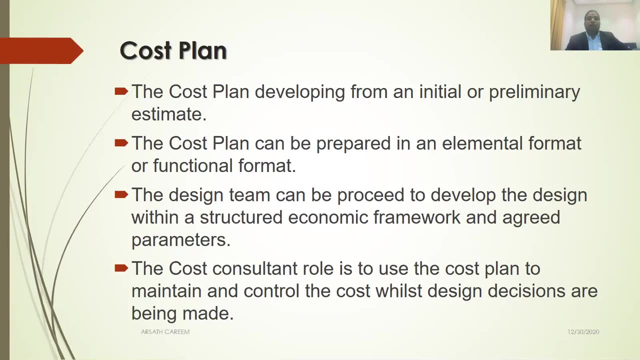 now we talked a lot about the course plan, but in the initial slide course plan i said cost to prepare a course plan, the first para. what was the cost plan, the first para. what does say the cost plan developing from an initial or preliminary estimate? so we learn about cost plan before cost plan. we have one activity need to know, that is: 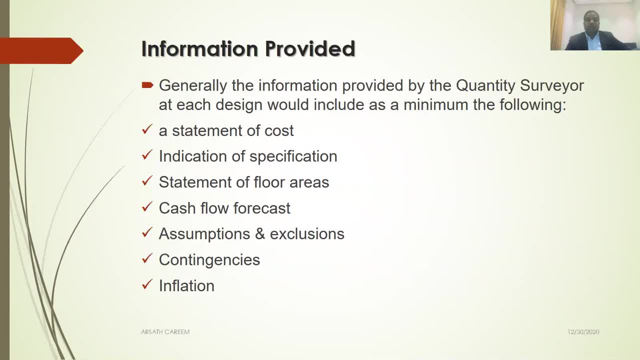 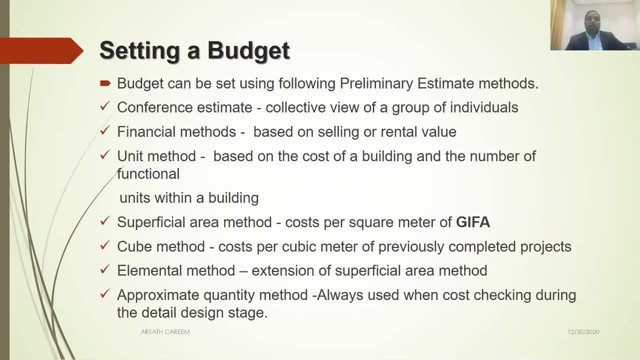 preliminary estimate, so cost plan take into place in second stage before that one. as a quantity server, you should know how to to the preliminary estimate or order of magnitude cost estimate. it is called order, so we will see how to prepare it. setting a budget. budget can be set using following: 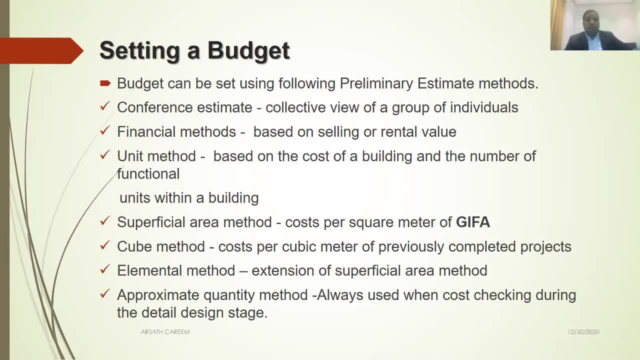 preliminary estimate methods in industry. there is two, four, six, seven methods available. it's a quantity server. you should know each and everything but you. you may use mostly superficial area method or elemental method, however better to know. maybe you have learned this one your undergraduate studies as well. just to make all. 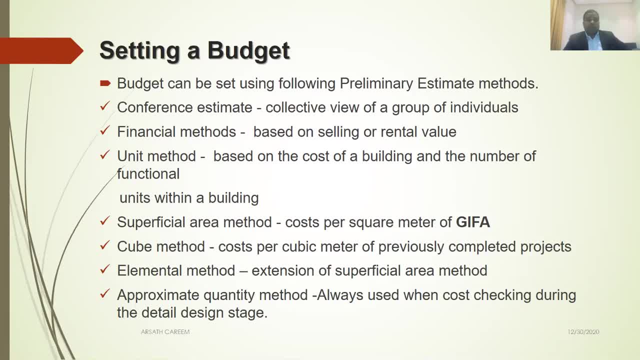 inclusive i. i have included in this chapter first one conference estimate. this is this. this estimate just about collective view of a group of individual, for example some high level people in the company, for example ceo mds. they have enough experience, they are decision maker, so they don't want any assistance in the early design. brief stage definition. 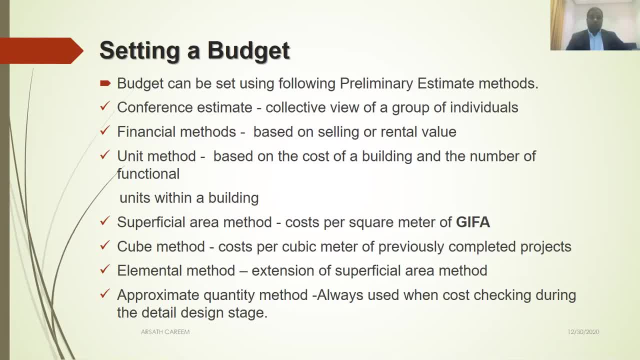 they, they need to set the budget, okay. so what they need to do is they need to come together and they, they get together and they discuss, for example, if they want to more shopping mall. the same the owner of the building that he built many malls throughout the 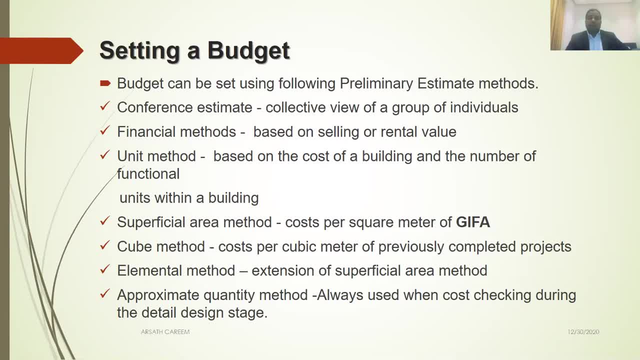 country. let's say: perfect example: lulu owner, you all know, especially in middle east. so lulu owner, he, he has, he has company ceo managing directors. so they all get together. they're just discussing: we okay, how much will be cost, because they want to build similar building when you. 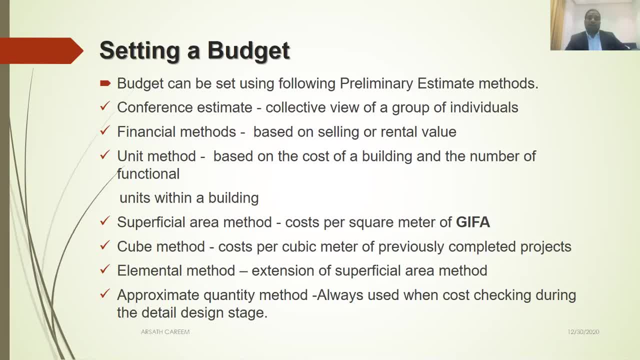 go to this, the shopping mall. they all are very similar to each other, so they can easily decide how much per cost. let's say, 10,000 per meter square in Qatar. we want about including all interior fit out, or we want to build this 10,000 meter square and this much, of course. then they decide. this is also. 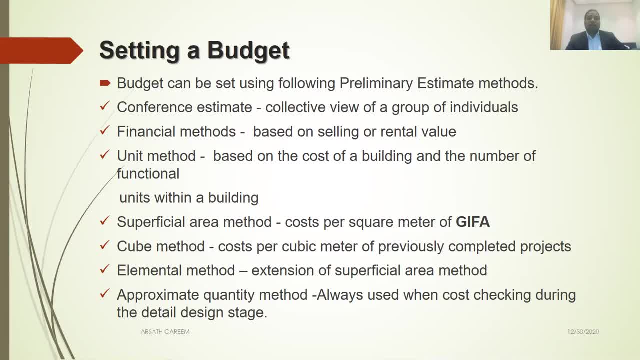 one of the way to set the preliminary estimate. it's not depend on the historical data or previous project. this through the experience. this is also- you can deny this kind of X, maybe this more correct because they, they are well experienced, they already delivered for that cost. so this is one of the method. 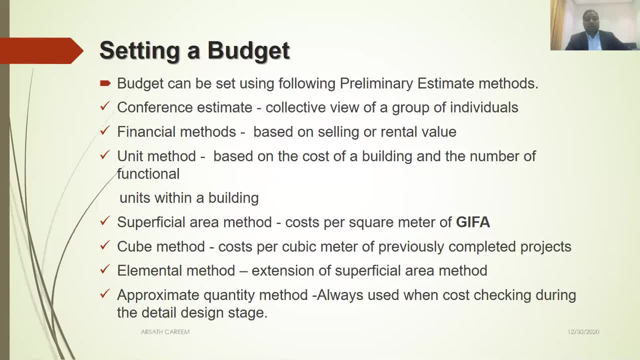 second one: financial method. this is mainly based on selling or rental value. you selling and rental value, for example, financial method. let's say you want to build apartment, okay, the selling value is currently in you. you are checking the market currently, let's say, in Rupee, Sri Lanka, which I know for the apartments. 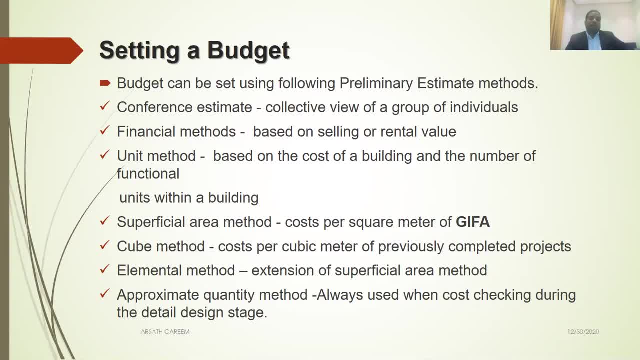 15,000 per meter, skip per square feet. okay, now you want to build 10,000, so you will incur one hundred and fifteen million cost. so one hundred and fifteen million cost, so you adding some profit for you. let's say five million, so two hundred million is your budget. simply, this is. 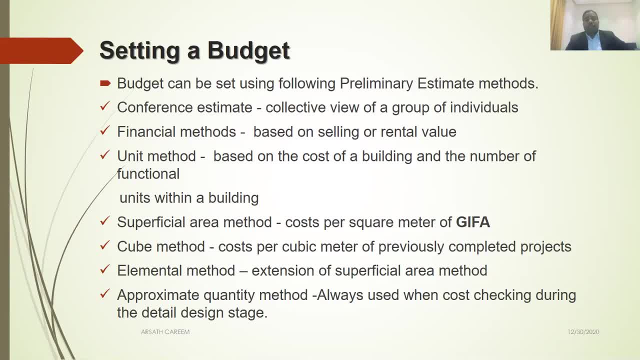 from all from from based on the selling a rental value. this is also one of the method. third, one unit method based on the cost of building and the number of functional you need within the building. this method generally use for the number of units for a hospital: 100-bed hospital, 500-bed hospital, one bed. how? 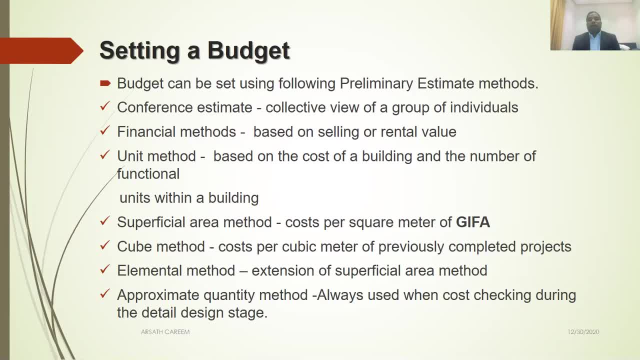 much, usually total building cost divided by number of beds for the hospital, for example, school, for example mosque, car park. these buildings usually we can easily measure through unit hotels, thousand, thousand hotel rooms per rooms per number. so, whichever the building, the functional, decided by the numbers, we can easily total cost divided by the numbers, then you will get the 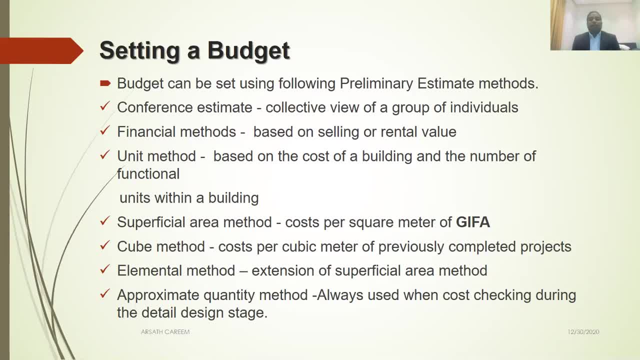 unit method, also a superficial area method. this is post-pass adolescence of gross internal floor area. what is gross internal floor area as perまり's definition can see the definition face of the external wall, excluding the staircase lift passage. so all the usable areas we can count as a gross internal floor area. this is the per meter square. 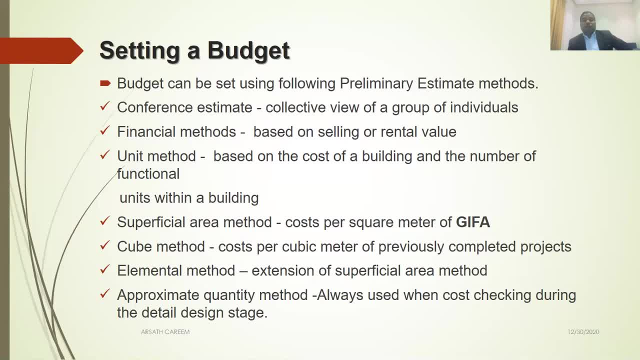 area. for example, if, if one building cost 500 million and your area 10,000, your 500 million divided by 10,000, you will get cost per square meter. next, one cube method: usually this cost per cubic meter of previously completed project. this, currently this method is not not in practice. previously, long time ago, this 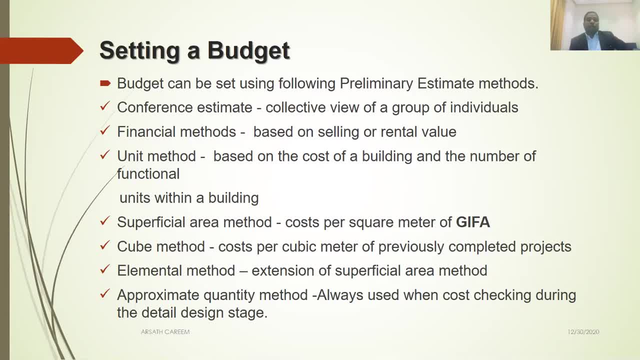 widely used. next, one elemental method. this is very similar to extension of superficial area methods. same method, however, is it's the cost break into the element of the building which I discussed earlier. the final one, approximate quantity method, always used when cost checking during the detailed design stage. this is normally used, not 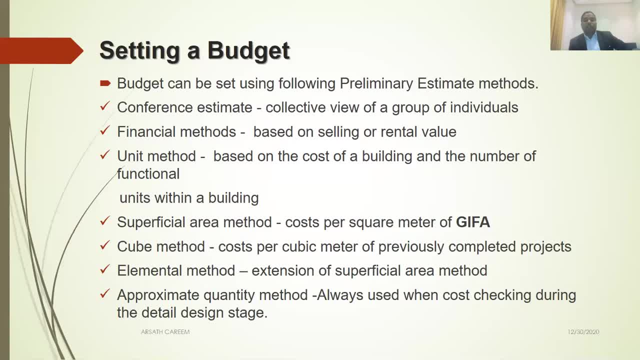 often used in the pre contract concept stage, but widely used in the later design stage. when there is a quantity you can, when you able to measure the quantity, this method can be used. so this is the explanation for setting a budget. so once you set the budget, it's become a cost limit, so the cost plan process start. 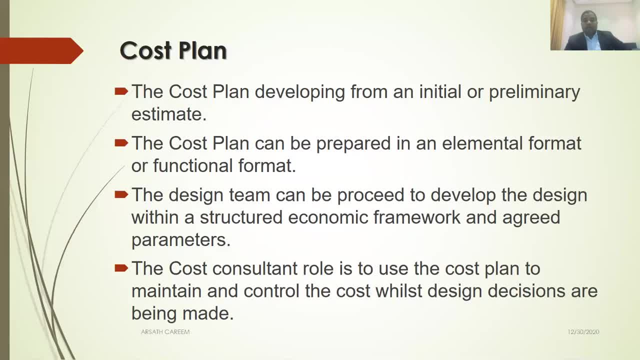 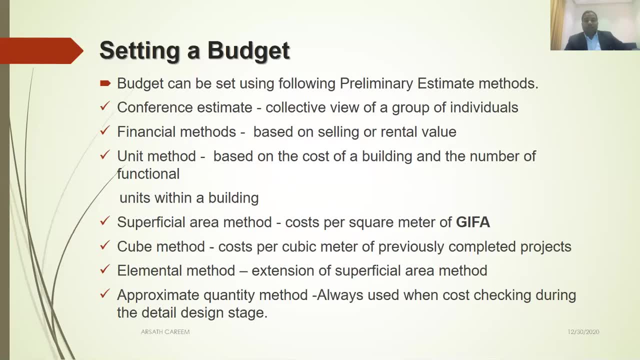 so what we discuss here, the first stage of cost plan, it is developed from the preliminary estimate. what we discuss: how to prepare a preliminary estimate. once you prepare a preliminary estimate, it is your budget then that budget converted in inverse budget, converted into cost plan, into the element, then your, your aim should be: you have to make sure. 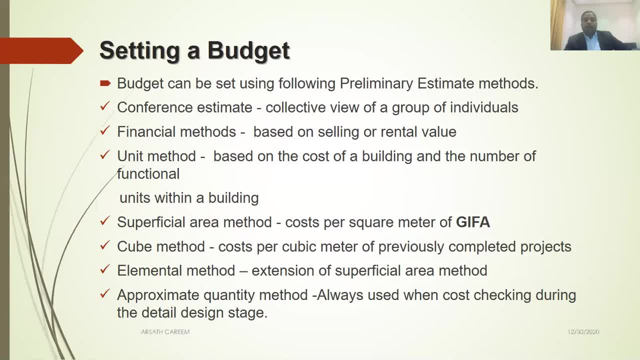 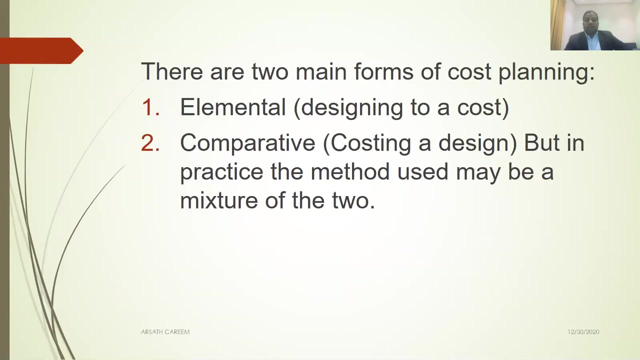 design within that cost target of each element. that is your main responsibility. okay, elemental method: now we talk about two types of course planning. now let's look further about the elemental method of course plan, two types, what we discuss before cosplan. there is a process: preliminary estimate. we discuss here now two types of cost planning that we 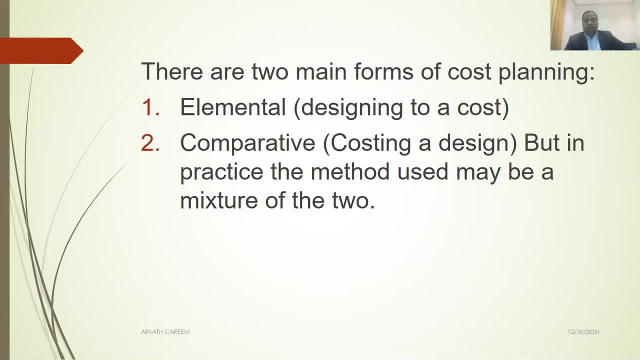 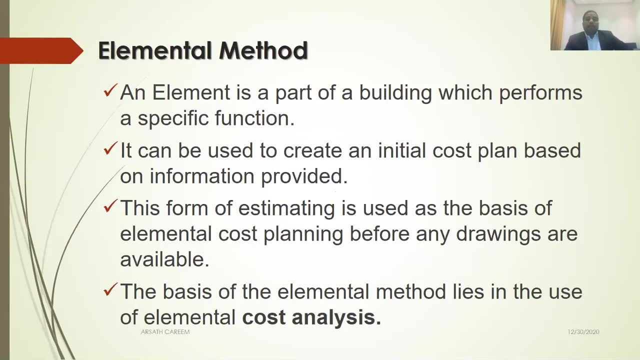 cost plan. what is? i already discussed? what is elemental? comparative detail of that slide will go here. elemental method: an element is part of building which performs specific function: substructure: it's one function. it's carrying the load transferring to the superstructure, provide, providing aesthetic appearance. wall partition, ceilings, aesthetic services. 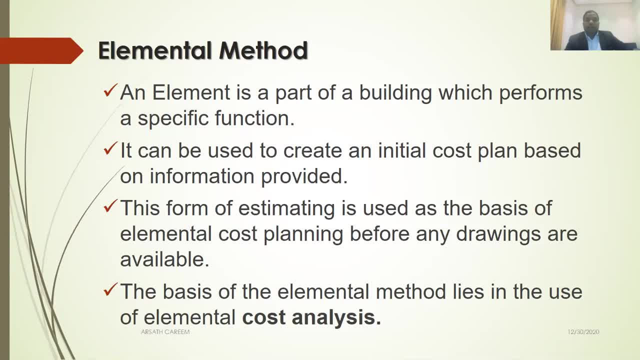 mvp services, external development. everything has a specific function. so elemental method, which performs specific function based on the function, it can be used to create an initial course plan based on information provided. this form of estimating is used as the basis of elemental cost planning before any drawings. 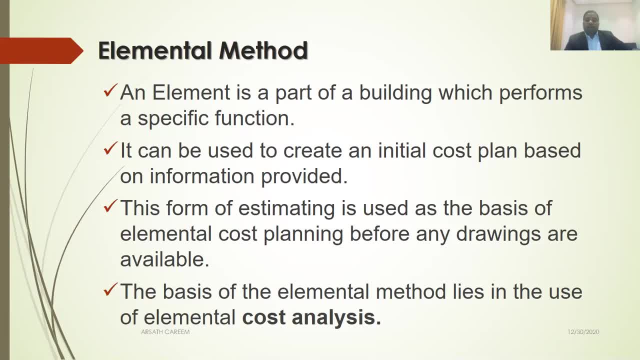 available for? okay, any drawings available. the assessor rics, as he will start the question, that normally the level one only. they will ask directly. level two and three, most of the question indirectly. so they will ask your client looking your course plan when you don't have any drawing available, what kind of advice you will provide. 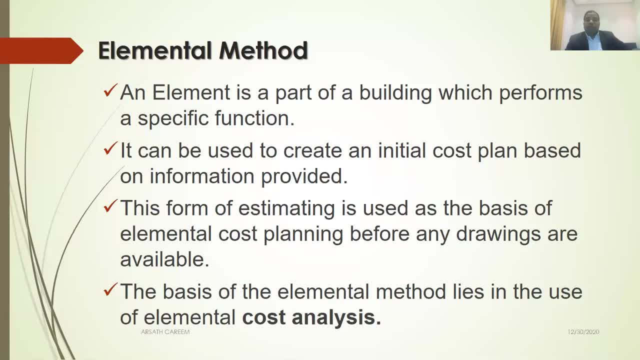 this kind of question they may ask. so you, you should know, when there is a drawing available, what mechanism you have. you have to control the cost, to to know the cost. So your answer should be structured way. The basis of elemental method lies in the use of elemental cost. 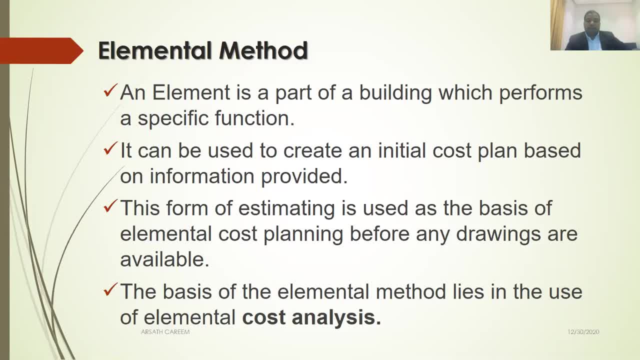 analysis. Now another Chapter coming is cost analysis. So elemental cost plan mainly depend on cost analysis. So now we want to know what is cost analysis. Once this type of cost planning finish, we will discuss what is cost analysis, Elements of building this. I already discussed this one. 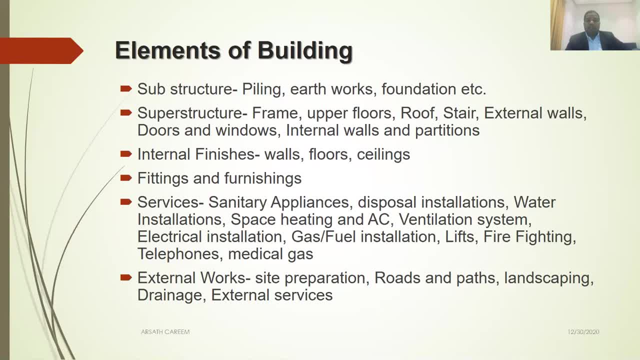 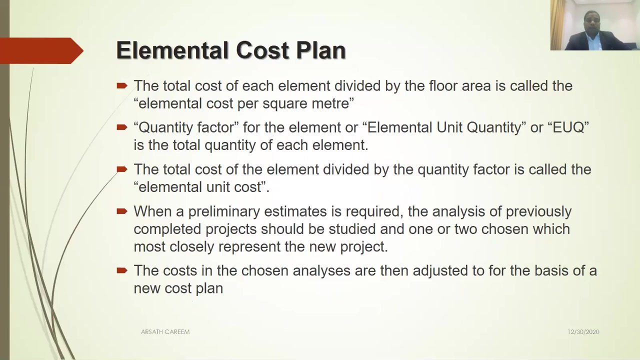 verbally. what is substructure? superstructure? internal finishes, fittings and furnishing services, external work- These are the category defined by RICS. These are the main elements of the building. So elemental cost plan, what it's all about, we, we. the total cost of each element divided by the floor area is called the. 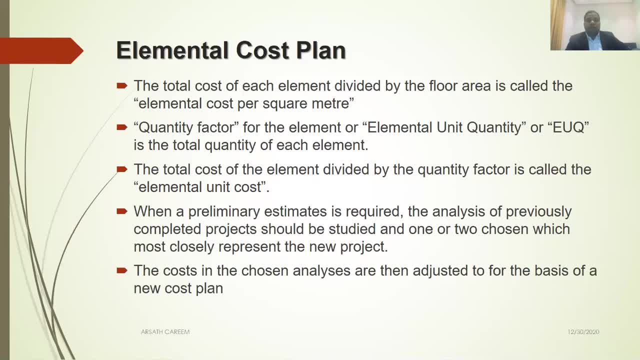 elemental cost per square meter. Total cost divided by the floor area: gross internal floor area. quantity factor for the element: elemental unit quantity is the total quantity of each element. The total cost of the element divided by the quantity factor is called the elemental unit cost. So these: 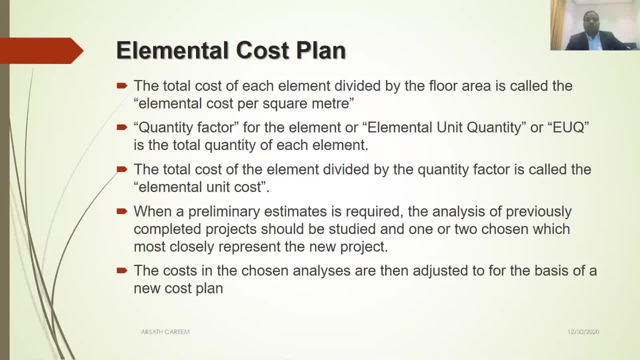 are the definition. What is elemental unit cost? Total quantity. total cost divided by the quantity, you will get the elemental unit cost. When a preliminary estimate is required, the analysis of previously Completed projects should be studied and one or two chosen which most closely represent the new project. When you choose the 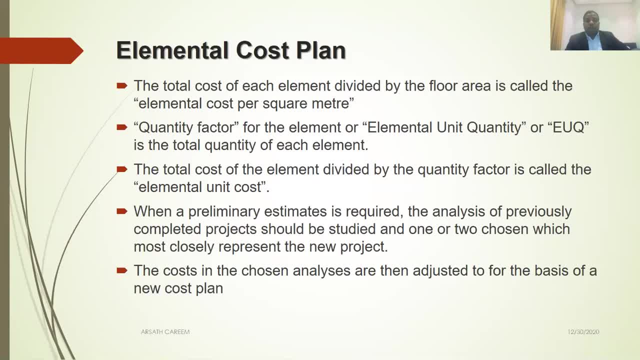 project. for a cost plan, you have to carefully choose Previous completed project And should be studied, and one or two chosen which mostly closely represent the new project. So it's very important to choose similar project. For example, if you want to build a hospital, you have to. 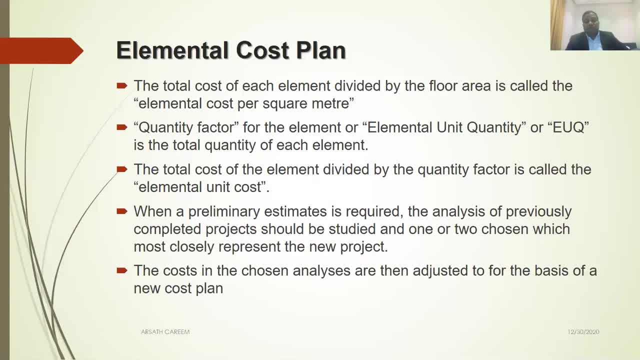 choose previously completed hospital project should be related to same function. Some hospital have basic function, Some have, for example, operation theater, So you you should choose which you have operation project: operation theater- cost information- That's what that para mean. The cost is. 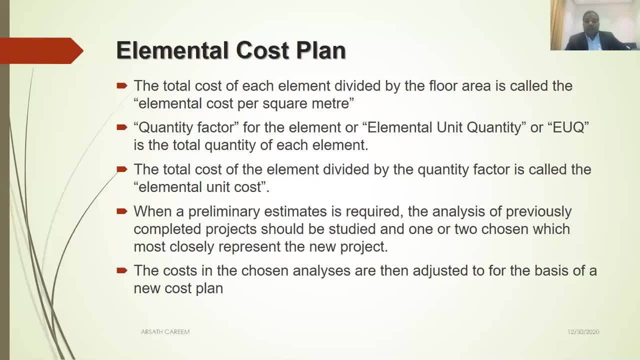 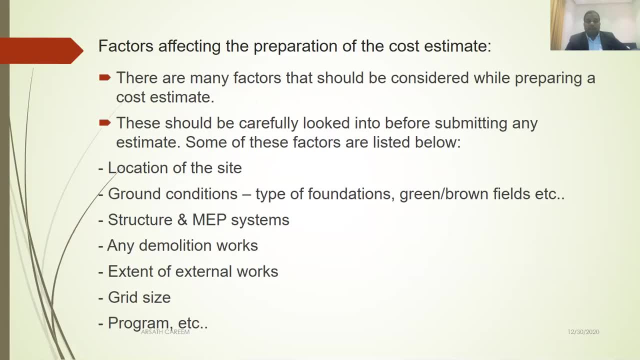 related to the cost of the cost of the hospital. So those are the basic aspects of the cost plan. So how you're going to adjust- we will see next slides- how you are going to adjust Factors affecting the preparation of cost estimate or cost plan. 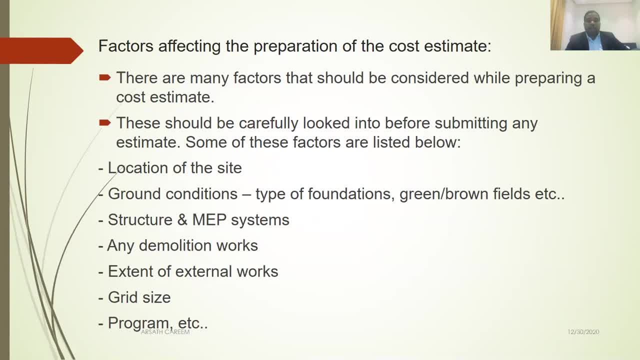 There are many factors that should be considered while preparing a cost estimate. This should be carefully looked into before submitting any estimate. Some of these factors are listed below. While you're preparing a cost estimate- preliminary cost estimate- you have to consider following factors, For example: 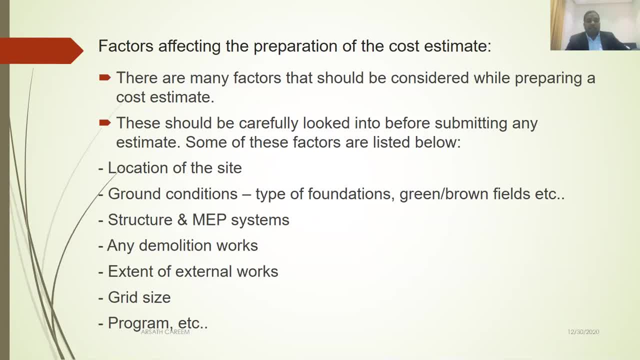 location of the site, ground condition, structure, MEP system. what kind of structure they use? what kind of MEP services they use? any demolition work is there? extent of external works, great size program. So, while we preparing a preliminary estimate, you have to. 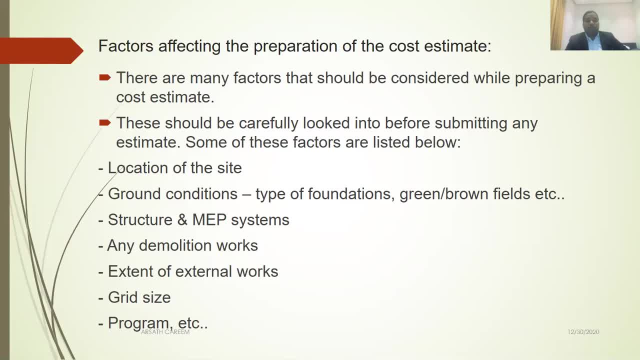 make sure you have to give adjustment How you are going. these are the theoretical, Too easy to understand. I have prepared one case studies in below slides. So just theoretical purpose for time being. just, you should know, you have to, you know to consider this factor. For example, if you 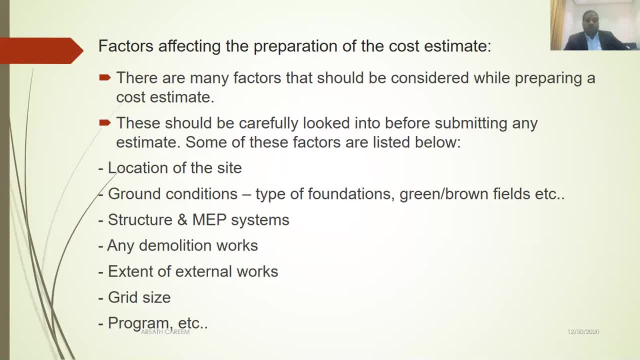 want to build one mosque in Doha and out of Doha. there is a lot of lag. Most definitely there will be a different due to location factor, due to transport factor, due to available labor, of labor resources, Using the technology in the area. These are the main. 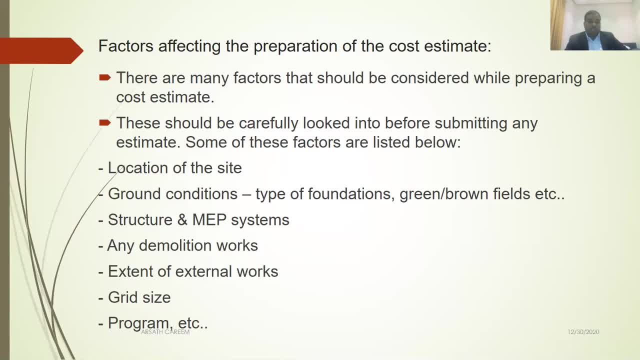 factors which we already discussed in the first, first chapter, factors affecting the design. So those factors affecting here as well, same same. So I don't need to go one by one. You should know what are these, how we are going to adjust as a quantity. 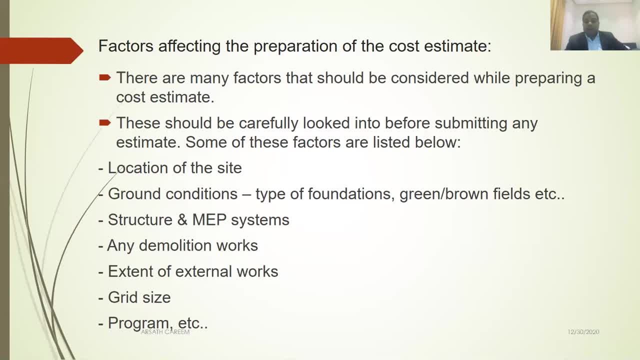 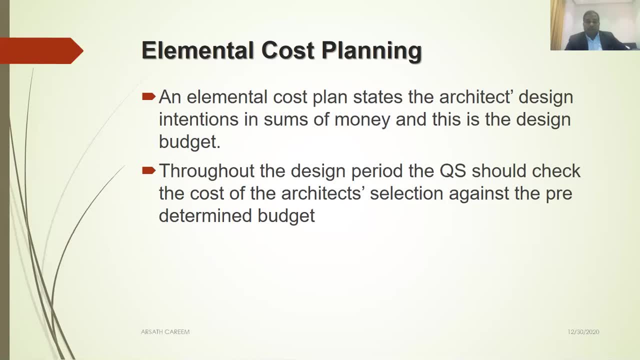 I will give you in below slides with the one case study. This is further to elemental cost planning. Elemental cost plans state that architect design intention in sums of money and this is the design budget Throughout the design period. the QS should check the cost of the architect selection against the predetermined budget. 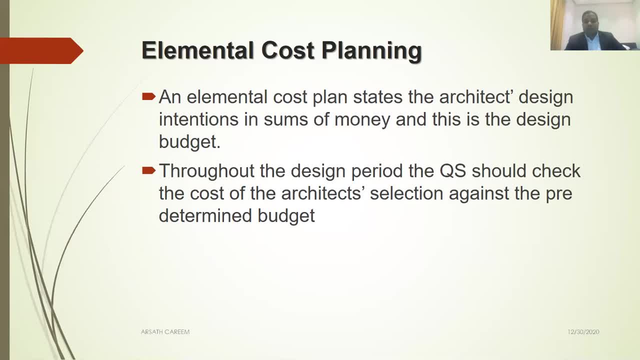 This we already discussed during the elemental cost planning. the QS should check the budget Against the architect design regularly and identify the difference deviants, and you have to communicate with your project team and you have to take any action required. For example, if you dissolve a budget, you can redesign or you can change the material specification. 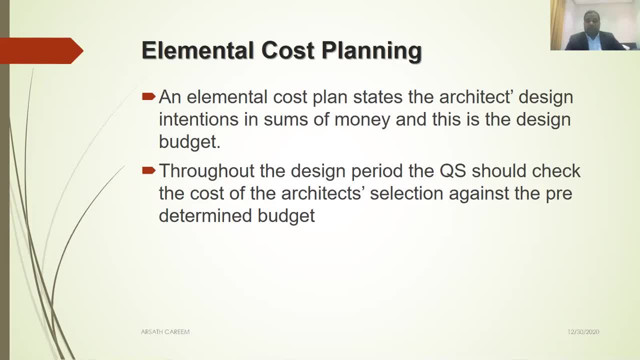 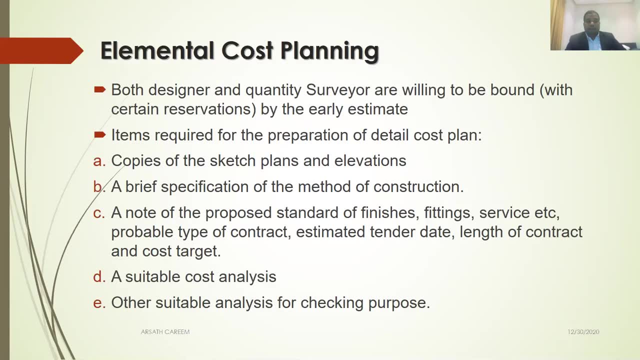 or you can conduct a value engineering. There are other mechanisms available. that is also will be discussed later slides. Thank you. To prepare an elemental force planning, the following details: you need copies of sketch plan, alleviation brief. specification of the method of construction and not of the proposed standard. 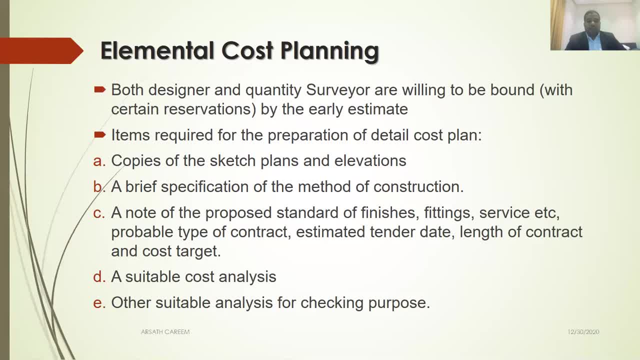 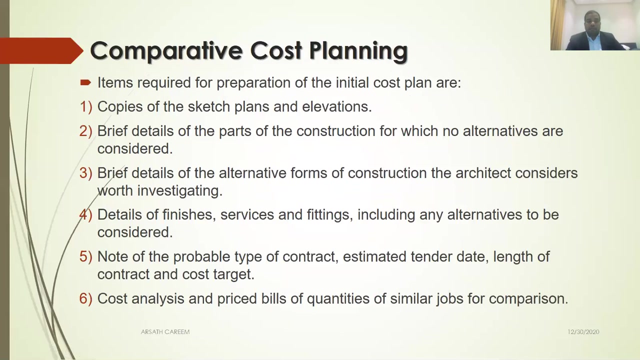 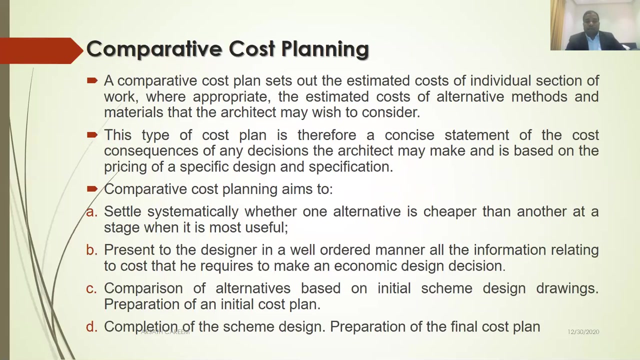 finishes, fitting services, Type of contract, estimated tender date, length of contract and target cost. Also suitable cost analysis- other suite of learners analysis for checking purpose. so what is cost analysis? it will come at the chapter. first we learn about the elemental cost planning. now we will briefly look about the 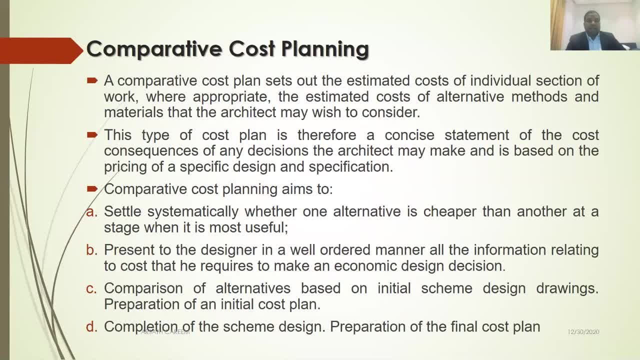 comparative cost planning. as I said earlier, comparative it's a design alternative design option available. for example, if you want to for a building, if you want to build HV system, you have option package unit. you can design a split unit. what you do, designer will design both and QS will. 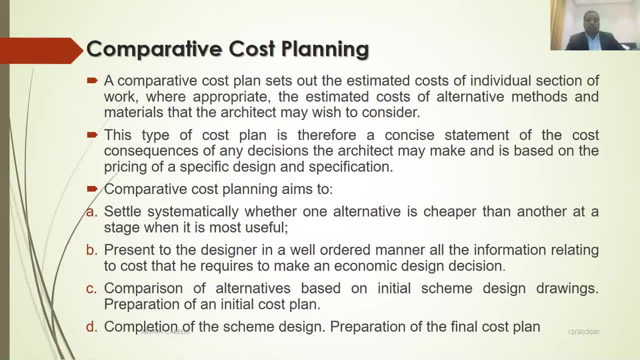 cost, both system package unit and the split unit, and compare the cost which is feasible. they will put it that is called comparative cost plan. other one elemental cost planning is a costing, a design. that is different process. this one another process. both are cost planning. comparative cost plan sets out. 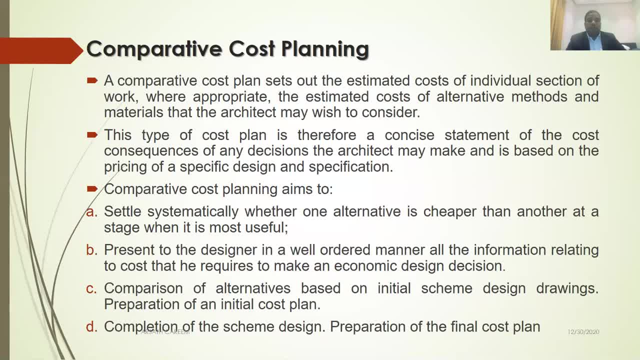 the estimated cost of individual section of the work. we are appropriate the estimate cost of alternative methods. that's what I called alternative methods, for example, like package unit, split unit you can use like a stack-case area- finalmente, я spell a little better. this steel door also for this lab, for the structural 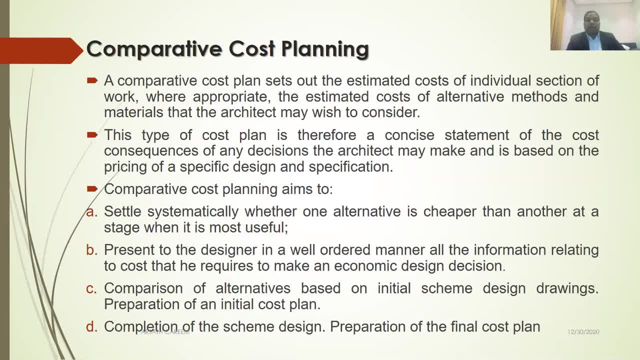 part you can design bit flat slab. all you can slap and beam. some other concept will be planned site like a stack case, area of ну I rated moon door o pirated steel door. also for the slip, for the structural part, you can design be flood slab or you can slap and beam some othercu. 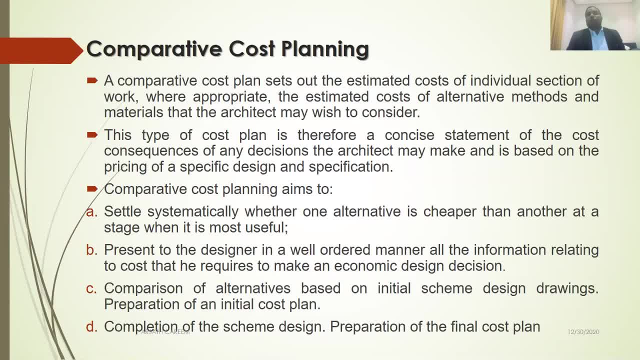 a question, if you have any comment, you might say: shape like patch. so we have a matter of administration. so you have a 1992, this laminated west, Кстати not technically- between US and China, various countries, Spanish and techniques available. so designer what he will do, he will design both, whatever the available methods. 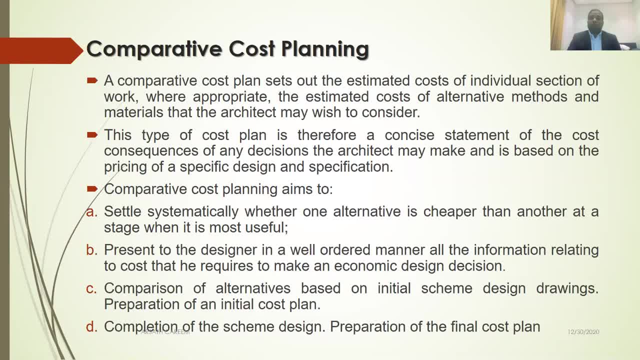 and he will give it to you to quantities. what you need to do, you have to price both of them. then you compare the price and the team will decide which system to be implemented. so this type of plan is therefore a concise statement of the consequences of any decision. 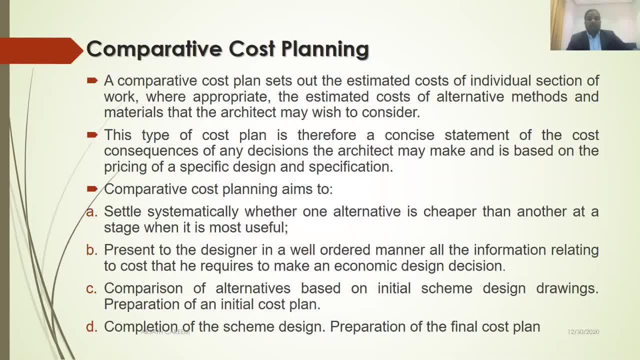 the architect may make and is based on the pricing of specific design and specification. so it's all about specific design and specification. the comparative cosplan aims is settled systematically whether one alternative is cheaper than another at a state when it is most useful. that's why i explained before. 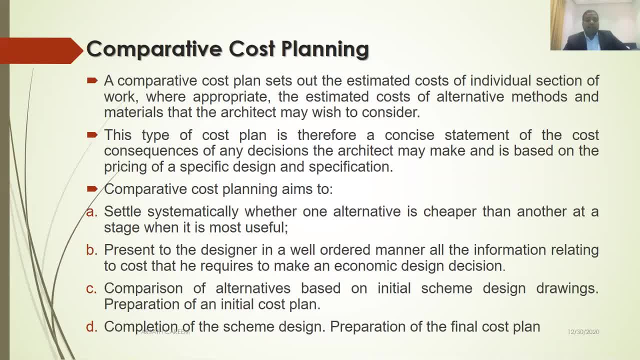 one alternative is cheaper than another at a stage when it is more usable, present to the designer, in a well-ordered manner, all the information related with the cost that he requires to make an economic design decision. so you prepare a cost and give to all alternatives with the cost details to make the decision. comparison of alternatives based on initial. 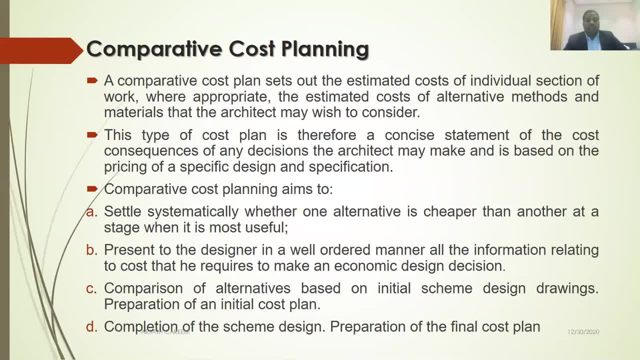 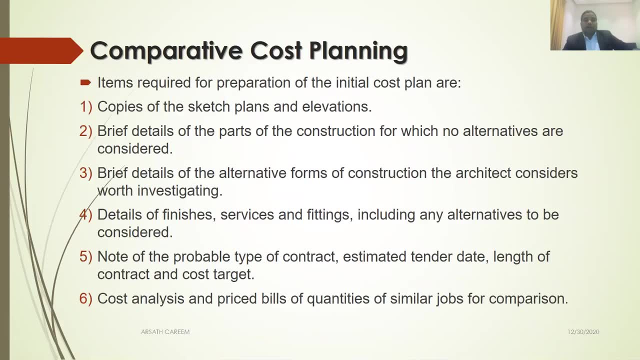 scheme design drawings. preparation of initial cost plan. completion of the scheme design. preparation of the final cost plan. so after all comparison, you have to prepare a cost plan including all the details. the followings are required to prepare a comparative cost plan. it's most of them similar. 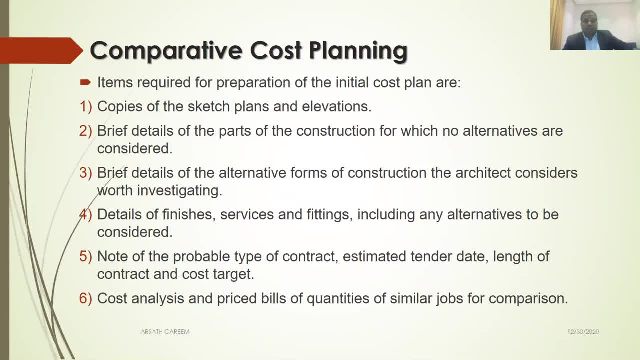 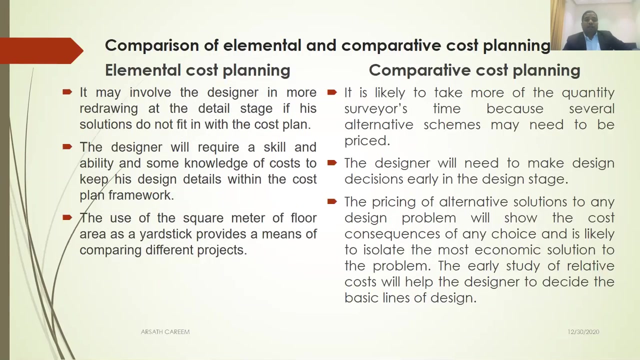 to elemental cost plan here. additionally, you need alternative condition number four- details of initial services and fittings, including any alternatives to be considered. this is one of the things additionally needed. when we compare to elemental cost plan, other older, similar to elemental cost plan, what information required sometime for part of level one? you you have a question. 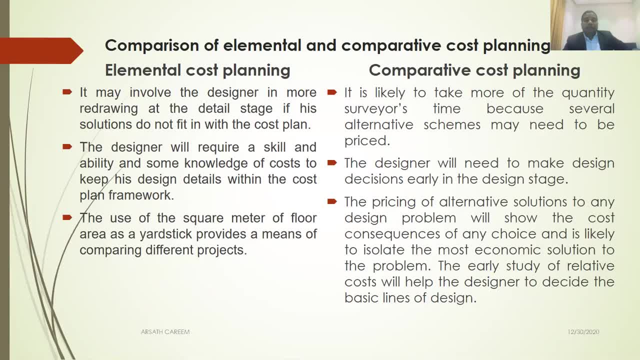 comparison of elemental and comparative cost planning. what is the difference? you may have a question. this is a level one question. these days very rarely ask direct question, however, just for theoretically better you know what is the difference. so just for reading purpose. i don't already discuss deeply, no need to go details, you can read and 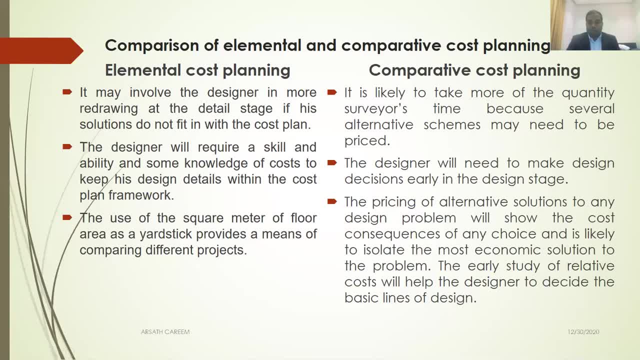 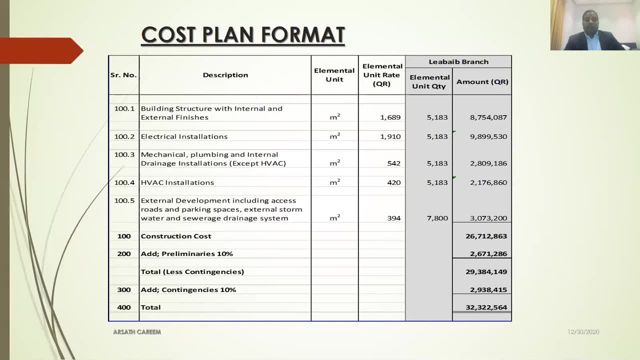 understand. so finally, we, theoretically, we studied what is course plan, what is the purpose, what are the steps process, what type of course plan. so far, we have discussed last half an hour about the course plan. now, after all, theoretical, this is the course plan format: how you produce. 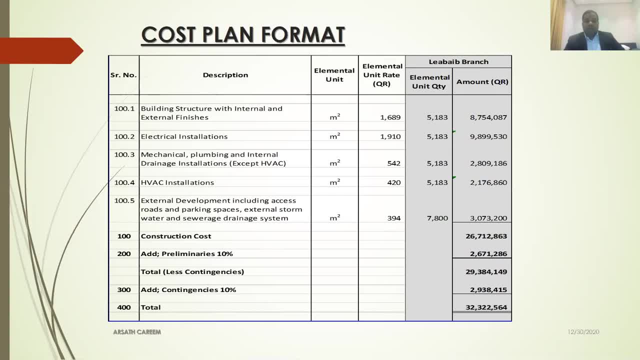 one of the- i just picked it from one of project which i prepared and i will explain it here. so our course plan is the course plan from one project to another project and uh, if, if it is going to be based on this, uh, we need to reduce its number of elements. to add the number of elements we have, for example, for elementals to add the number of elements. for elementals to add the number of elements. so here, building structure, internal, external finishes, rather than putting substructure superstructure internal finishes, i covered it within one item to reduce the number of elements. for elemental unit rate. elemental unit quantity amount. 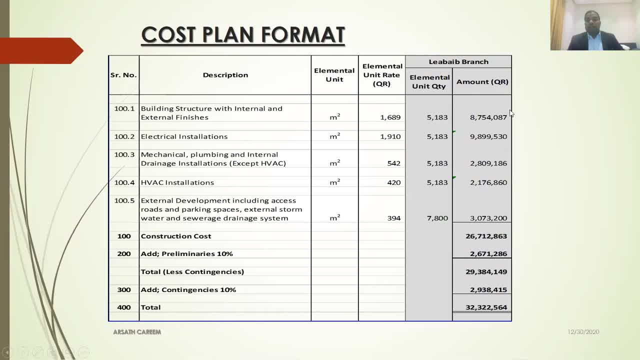 this is. this is my target cost for each item. let's say, I prepare this course plan for concept stage. okay, this amount, 8.7 million- this is the cost plan for this element. so designer architect is his aim should be: you need to design, you need to design the project within this budget. this is the. 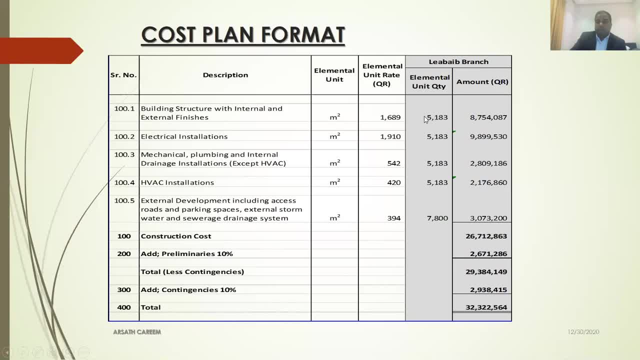 elemental unit quantity mean total area of the building and the elemental unit rate thousand six hundred eighty nine, which which this rate we derive from preliminary estimate, preliminary estimate which is we discussed before. this is the project budget and this is the project budget, and this is the project budget. 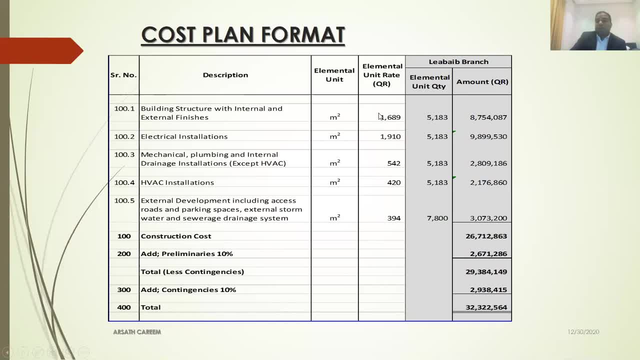 investment estimate. cost per meter squared. okay, superficial method. I use superficial method. this is the elemental unit rate for my project for these items. how I get this rate? okay, you say elemental from preliminary estimate. from preliminary estimate you can get a only the cost limit of budget. but how you get this rate using previous 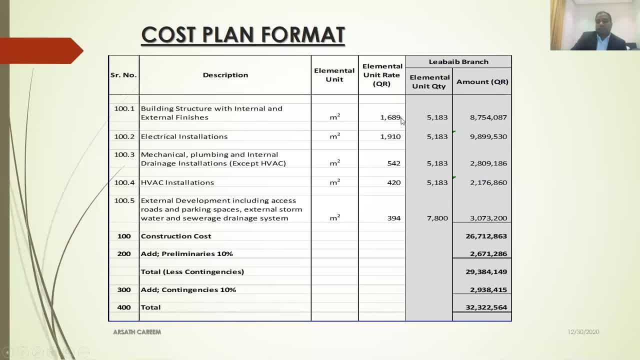 completed project cost analysis. so, in order to prepare a cost plan, you should know how to prepare a preliminary estimate in addition to that one, how to do cost analysis. so one one area increasing, you want to know how to do cost analysis. from cost analysis I derive this rate cost. when you say cost, 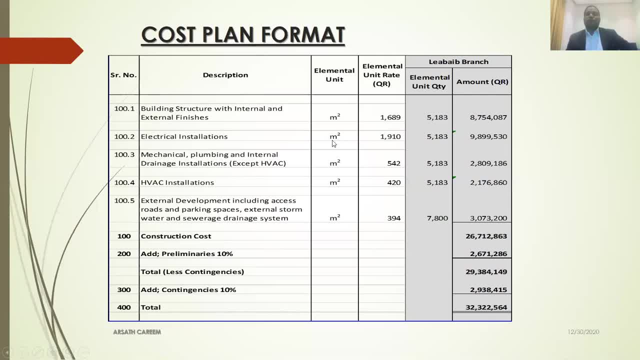 analysis is examination of cost of each function of the building from previous completed similar projects. it's very important you have to do cost analysis for similar projects and you need to do some adjustment based on the factors, for example, location, time factor, risk assessment, contingencies we will discuss later so accordingly, my construction cost I prepared for this particular project: 26 million for the concept stage and my preliminaries 10 percentage. then I added contingencies: 10 percent for design development, 5 percentage for any variation during the construction stage, 3 percentage and client reserve money: 2 percentage for safeguard. for this project my budget was 36 million. 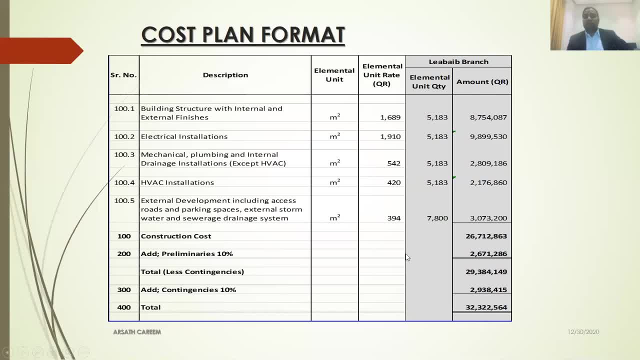 however, my cost plan after the concept stage was 32 million, point 3, so still within there cost cost limit or budget. so when it's reached more than 36, only we have to explore, find alternatives. so this is one of the cost plan format. second, once you 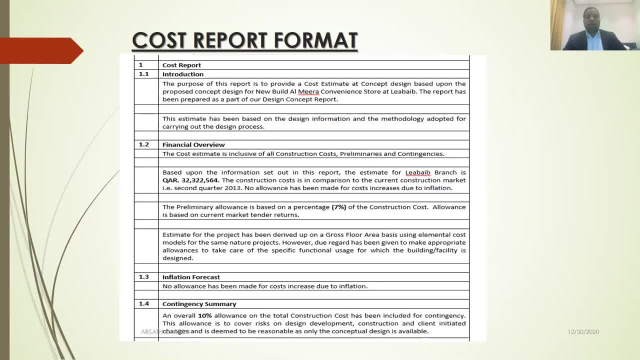 prepare a cost plan. you have to submit a cost, remote cost report to your client. it's a quantity server. it is your main duty. you have to prepare a cost plan for Pour out your cost- both the costанс price and the budget, in one investment. 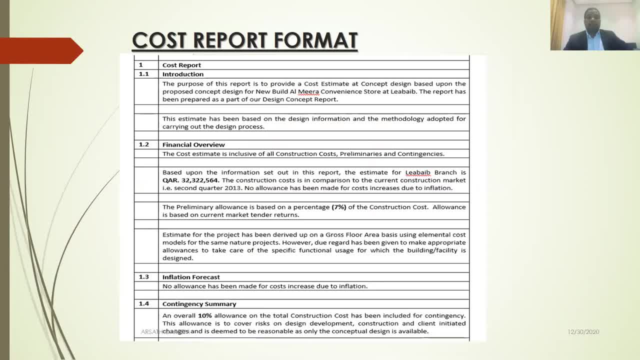 return for this project content, you have to submit the previous project as Aurora Como. these are obviously cost reports. usually cost is above that page so that you can move forward according to the pharmacy mulher will be required. you need to before completion. to make a cost report for project is needed. 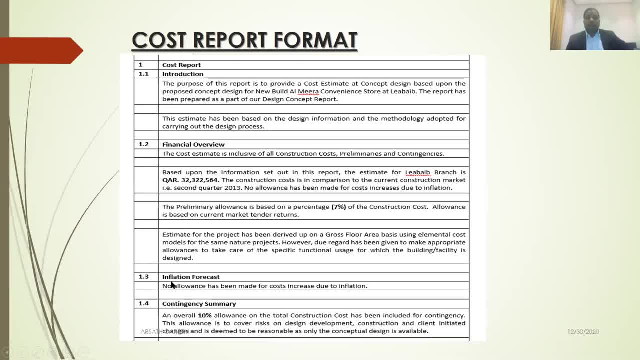 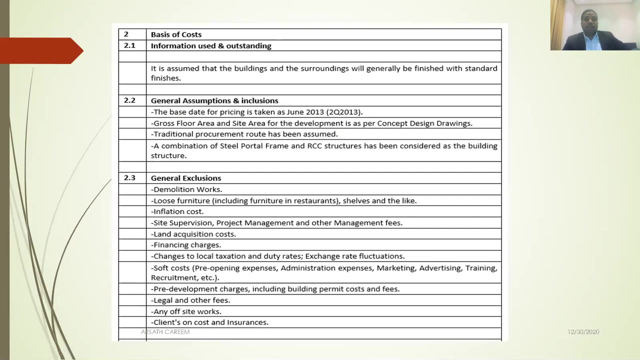 and I include any inflation forecast. we here, we haven't had any inflation, so here no allowance has been made for cost increase due to inflation. also contingent summary. so how much percentage? this is the cost report format for the basis of cost information used and outstanding. it is assumed that the buildings and the 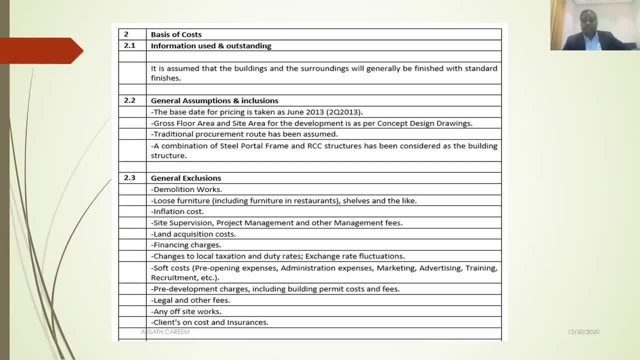 surroundings will generally be finished with standard finishes. so during in our cost we are considering standard finishes. any assumptions, inclusion, any exclusion. these are the things mainly you must include on your cost for cost plan format, cost report format for the cost plan, especially assumption: which which period pricing you have taken. 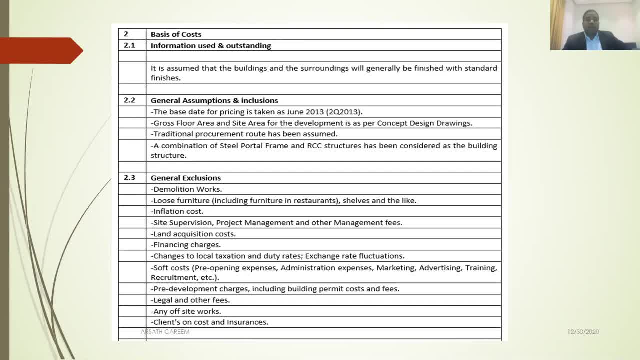 which stage of drawings you have considered, what procurement route you consider, what structure you considered? here we considered a combination of steel portal frame and RCC structures, also a general exclusion. what is excluded? for example, any demolition work, use furniture, inflation cost, site supervision, financial charges, soft cost, pre development charges, legal other fee. whatever you considered, you have to. 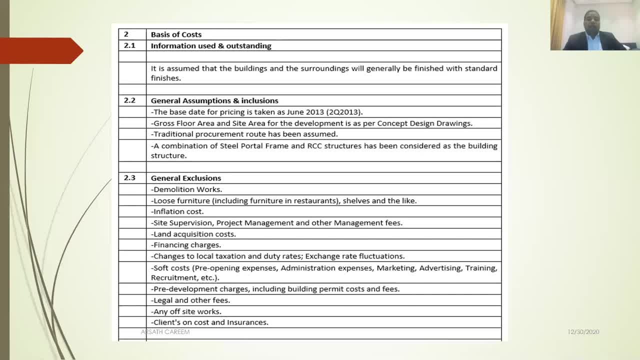 communicate with your client. clearly this is very important. also, this is level 3: what RICS expecting from you. so first report this there. level 3: competency: how to prepare cos. they will ask if you write any a summary experience. when you write you a cost plan, cost report, they will definitely they will ask question from what you did, how you did. 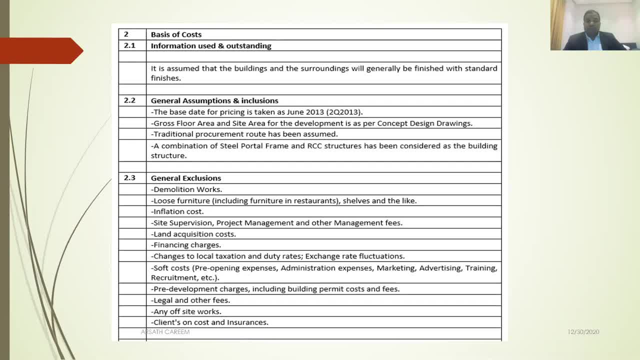 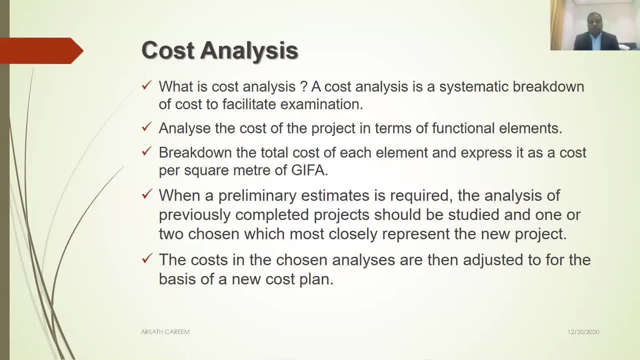 how you give your advice in abnormal situations. so we so far we have learned about the cost plan. to prepare a cost plan we need preliminary estimate. i have already discussed another one we need to prepare cost plan is cost analysis. this is also one of the main contents of this course planning. 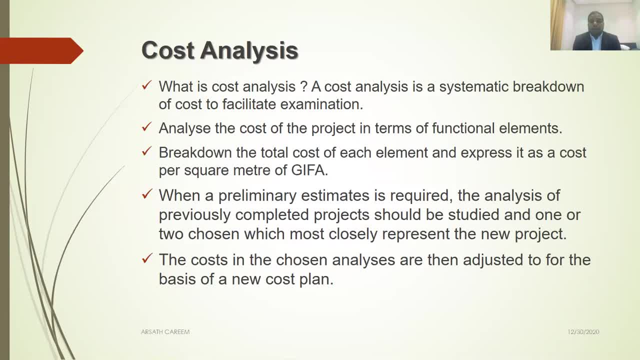 actually what is cost analysis? it is simply, it's a systematic breakdown of cost to facilitate examination. simply say it's a post-mortem of the completed project cost or tendered project. when you finish a project or when you tendered awarded project, you can take that cost into breakdown and you can analyze. 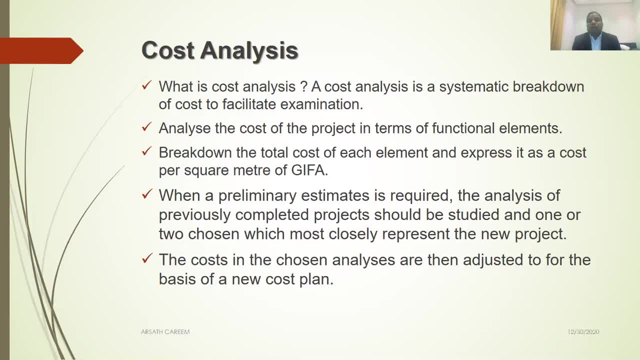 you can do analysis: how much will cost per meter square for each element? it's the same exercise for elemental, just you have to analyze, analysis for the completed project, analyze, analyze the cost of the project in terms of functional elements, break down the total cost of each element and 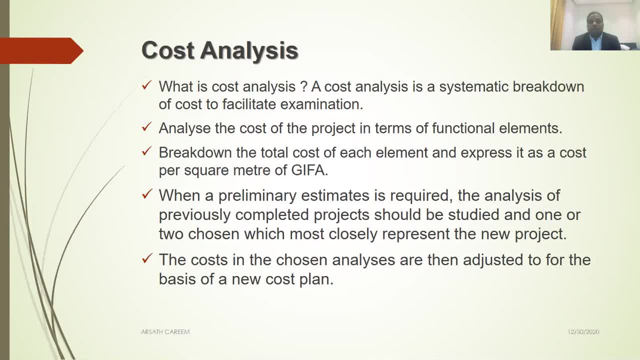 applied field reporting. each element fits in an essential level for the future project parameters to be analyzed and the analysis of the completed project will compare as a cost per square meter of cross internal flow radian. when a preliminary estimate is required, the analysis of previously completed project should be studied and 102 chosen which most closely represent the new. 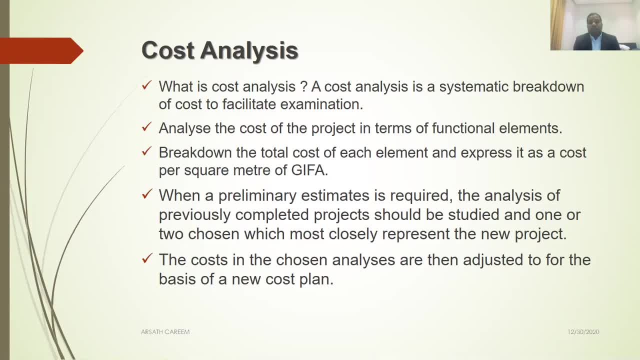 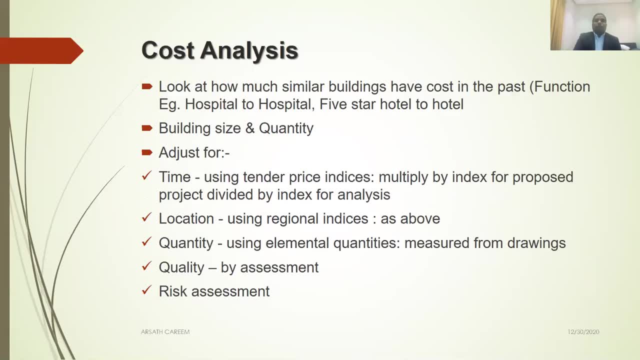 project. the cost in the chosen analysis are adjusted for the basis of new host plan. for the new cost plan. how you will adjust it, You have to consider similar buildings for the cost analysis, For example, based on the function hospital to hospital. 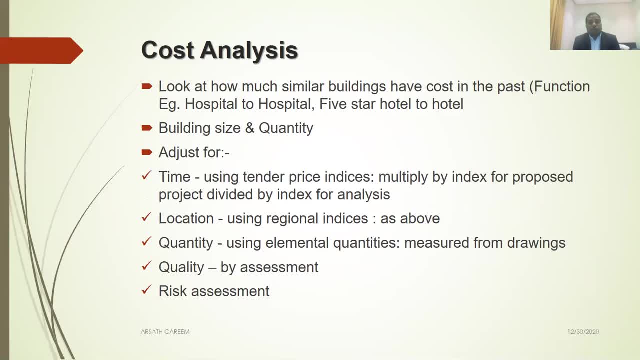 five-star hotel to five-star hotel, mosque to mosque, also school to school. Similarly, if you want to do analysis, you have to choose similar buildings. also size and quantity. You can't compare with 100 meters squared with 10,000 meters squared. 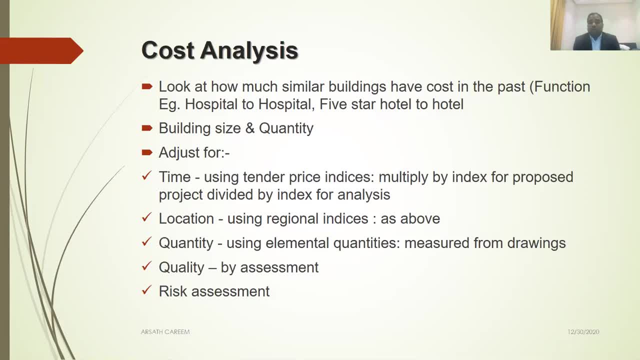 because, depending on the quantity, cost always will impact. While you're choosing for cost analysis, you have to choose similar building size and quantity. After you've chosen, you have to choose the building size and quantity. You have to adjust for time, location, quantity, quality and risk assessment. 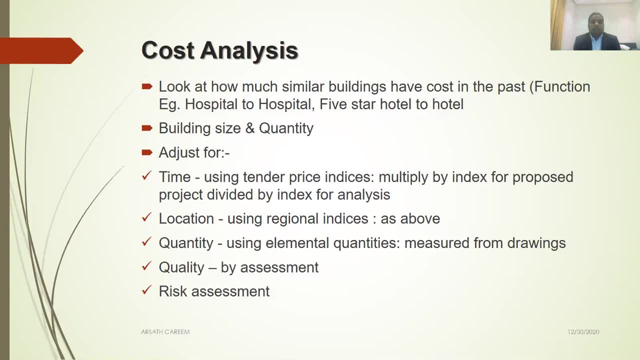 Time is very important because you take a project in order to analysis in 2008.. If you want to build in 2022, definitely there will be an impact on the price due to time difference. How are you going to adjust? Sometimes the location may be different, as I discussed before. 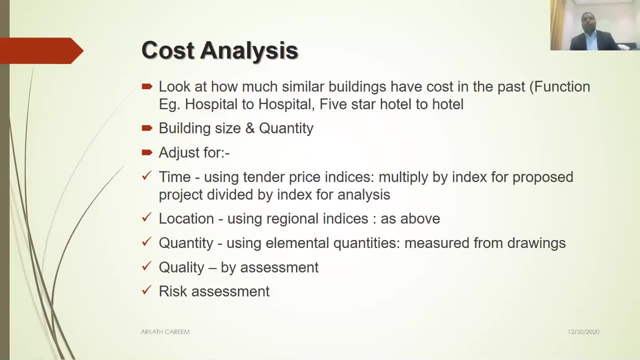 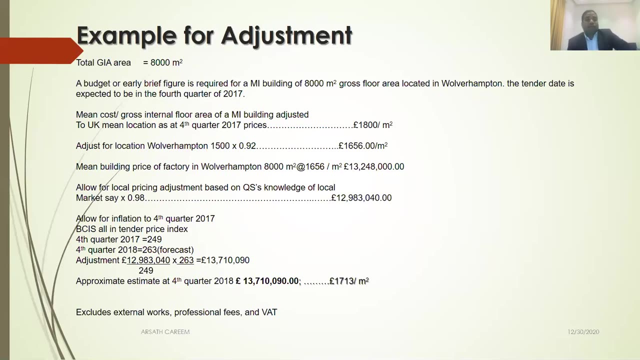 Quantity, also quality, also risk assessment, These factors you have to consider. To make you understand, I have taken one exercise for you. Example of adjustment. Let's say this example. I directly pick it from my University assignment, which is very suitable to illustrate the situation. 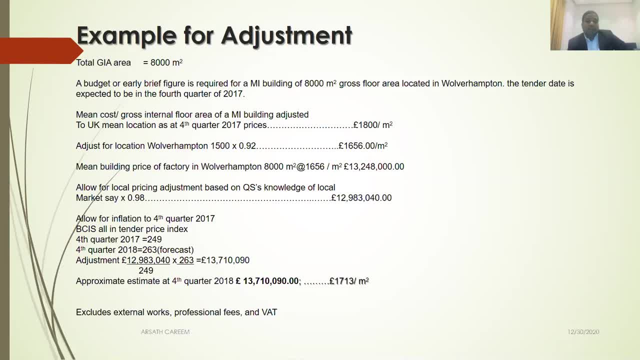 For example, my university building has one Millennium City building, one in one place. Usually my university have another location. They want to build the same building in another area. So the task is a quantity survey for me. I want to tell how much will it cost for the same building in another location in another period. 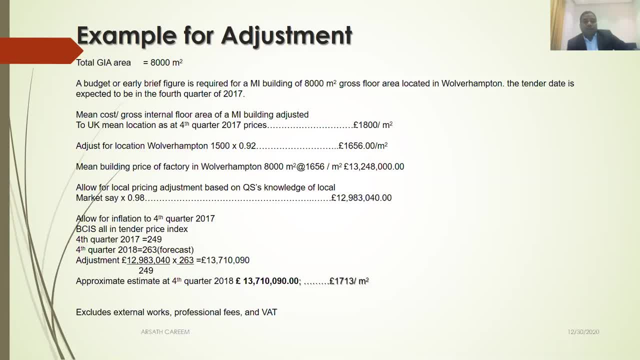 So the data available: total internal floor area: 8,000 meters square. So you want a tender date is 2017.. This adjustment can be made, especially in UK because they have a proper cost database, especially in UK Because they have a proper cost database. 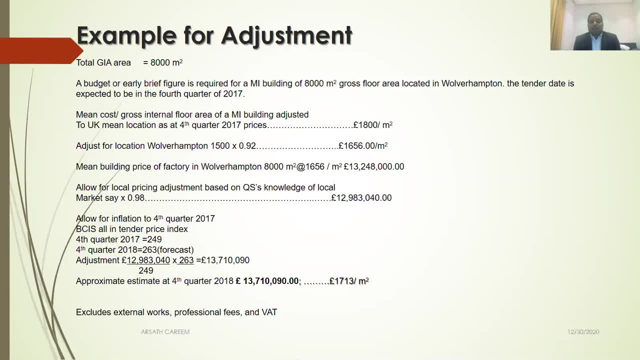 especially that is called BCIS, Building Cost Information Services. They regularly update every quarter about the cost information. Unfortunately, this information not available, especially other part of the world. only this costs data available on developed countries For the study purpose. we should know how these factors affecting the price 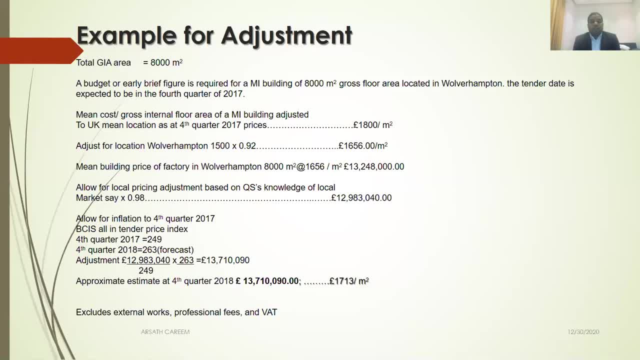 We should know what, how it's influenced the cost of the building. So the case is you have to build 8,000 meters square in fourth quarter of 2017.. For the for this cost, you have to open your BCIS price index. 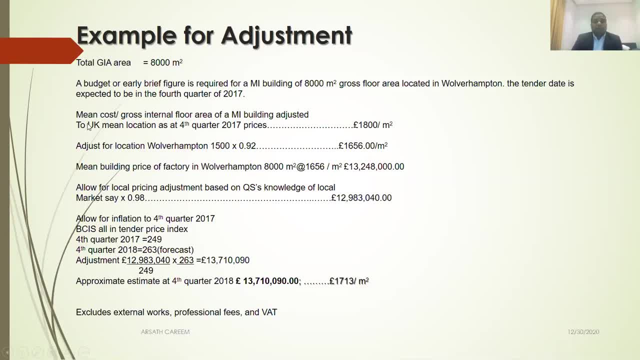 It show here for the UK, all over UK, and the mean mean for this this period, fourth quarter of 2017, prices: $1,800 per square meter. So you have to take that 1,800 per meter square. So this is why, throughout the UK now, 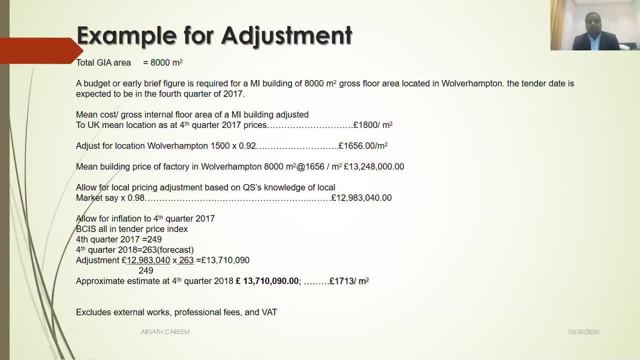 you want to build this building in Wolverhampton, the place called Wolverhampton, So you have to take that 1,800 per meter square. you have to take that 1,800 per meter square, per meter scared as a mean cost. and there is a location factor for. Wolverhampton: 0.92. unfortunately there is a error here. that is not thousand five hundred eighty thousand eight hundred thousand eight hundred. you have to adjust for location factor 0.92, which is thousand six hundred and fifty six per meter square. so total cost for eight thousand meters got around thirteen. 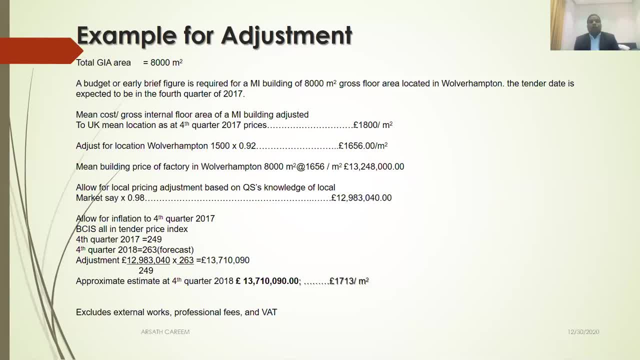 point two million now as a key was experienced. key was normally sometime. you have to adjust for local markets condition by identifying the risk and this one for. for that purpose I have multiplied by 0.98. I feel this is little high, so therefore I use you. see my local knowledge to adjust this cost. now you need to find out if you want to build this in fourth quarter of 2018, how much will be. if I want to build in fourth quarter 2017: 12.9. if I want to build in 2018, definitely there will be a. 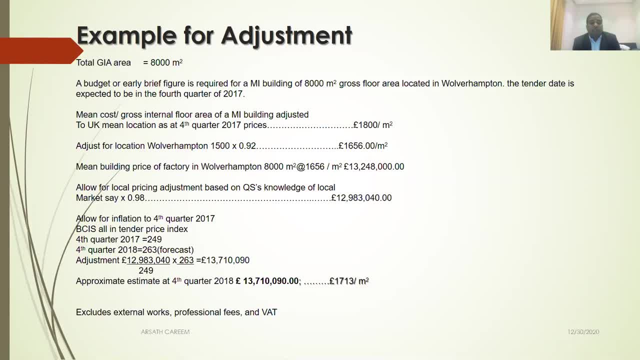 inflation, there will be a change. so now the price index coming to effect so that you can get, is that the record now? the average was 2008 oractually not 해- 0.43 $6. they regularly updated the fourth quarter price index: 249 for fourth. 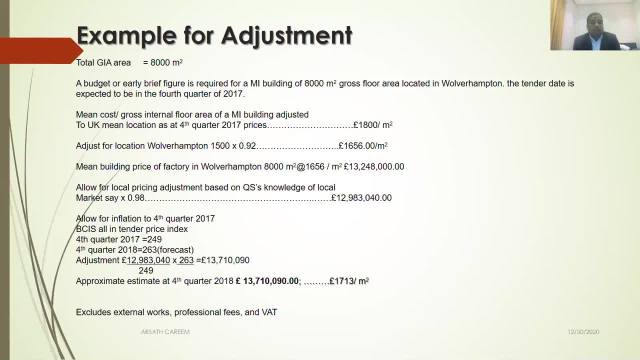 quarter of 2018. they followed authority 263. now you have to do small adjustment. previous sum 12.983, so you will reach 13.7 million if you want to build in one year after. so in this example, you are adjusting for location, you are applying your knowledge, you are you. 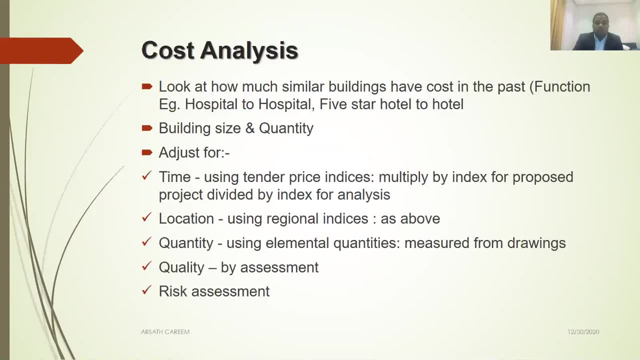 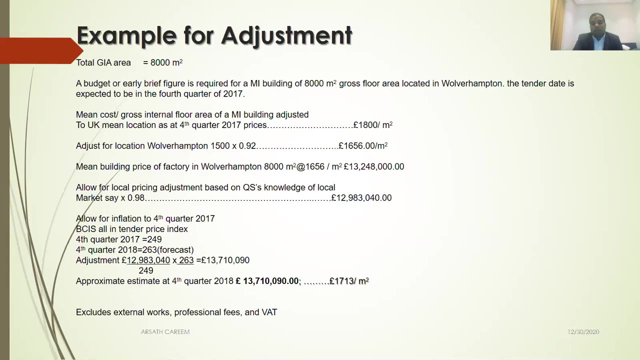 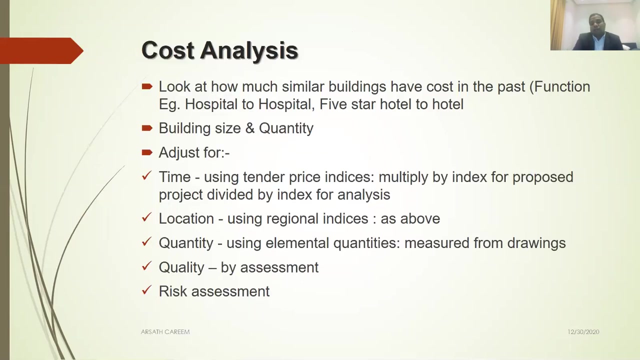 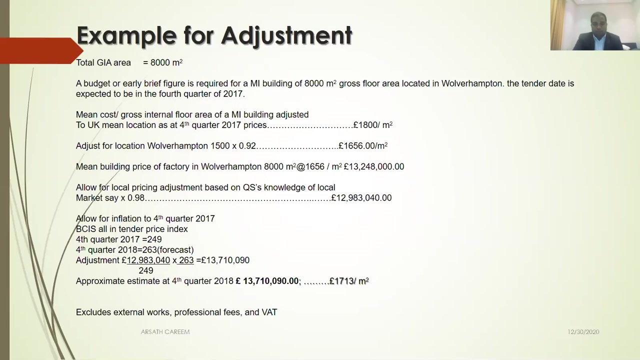 are adjusting for time. so one example: you are adjusting for all three of the cost. so what you learn here, and just for time, location, quantity, quality, risk assessment- it's a quantity server on that. on that example, i did three adjustment: time, location and risk assessment as a quantity server of by using the, my local knowledge. so this is the reason i picked this. 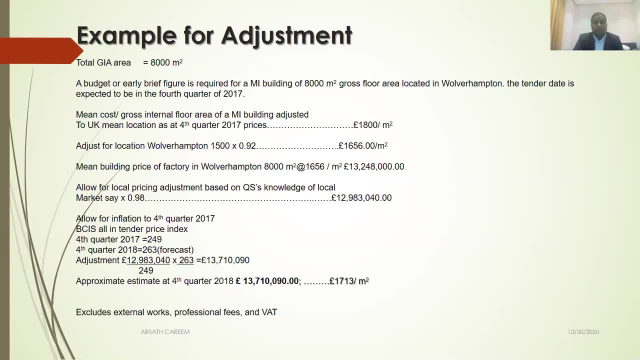 example. normally this part of the world we don't do, but we have to do for inflation, inflation. qatar statistics authority, you can get the cpi consumer price index for this adjustment. other than there is no location factor, also no local knowledge or risk assessment. we do this part of the world. so this is the example. 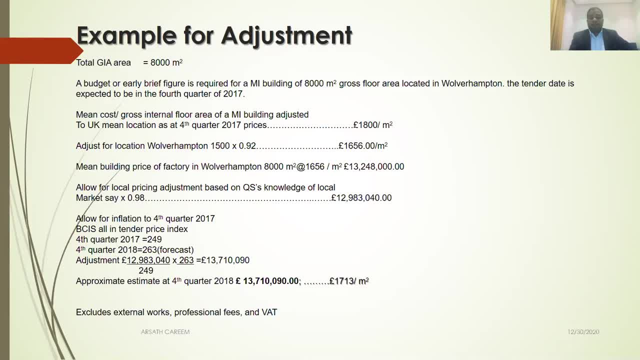 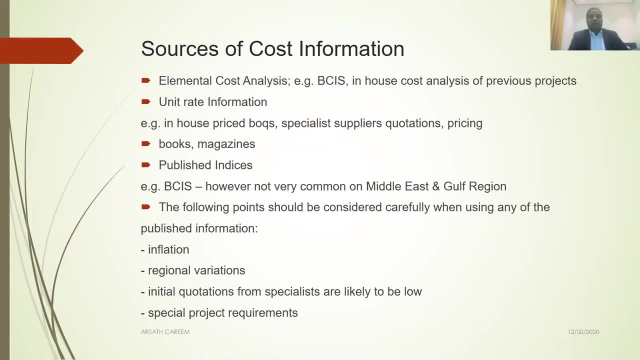 how you need to do the adjustment for cost analysis. so in order to prepare cost plan, you should have a cost information. without cost information is impossible task to prepare a cost plan. so what are the sources available with us to prepare elemental cost analysis? for example, bcis available in-house. cost analysis of previous 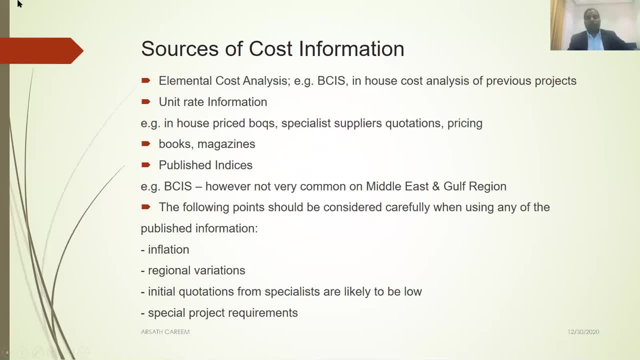 projects unit rate information. these are from previous projects. also, the following point should be considered carefully when using any of the published information: inflation, regional variation, initial quotation from spell specialists are likely to be lower special project requirements. so how you will get the cost information from these sources. 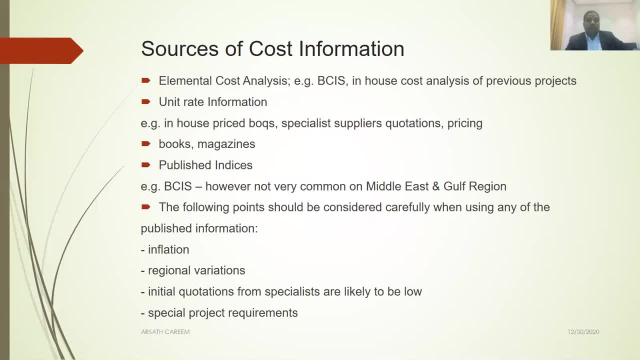 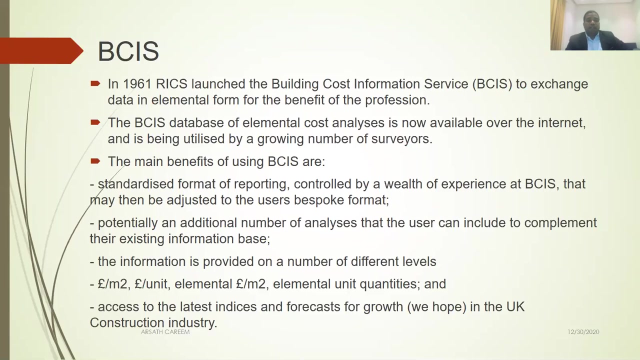 especially in Medellin. we usually have in-house cost data quotation from supplier. these are mainly used but there is no proper structure of state are not available this part of the world. just briefly about BC I S. it is launched cost information service services based on core cost information from the channels in the world. 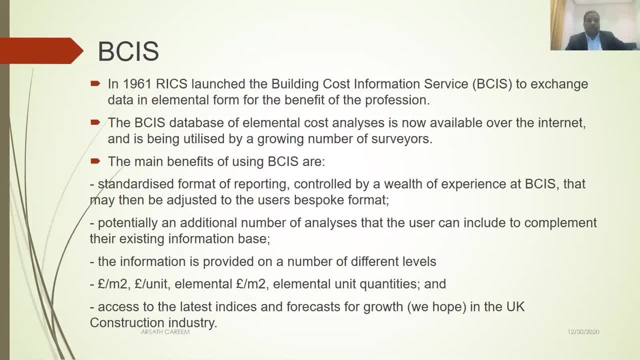 Building Cost Info Services, which is launched in 1961.. The main benefits: it standardized the format of reporting controlled by wealth experience at BCIS that may then be adjusted to the user bespoke format. Especially this, very useful in Europe, Just for your information. 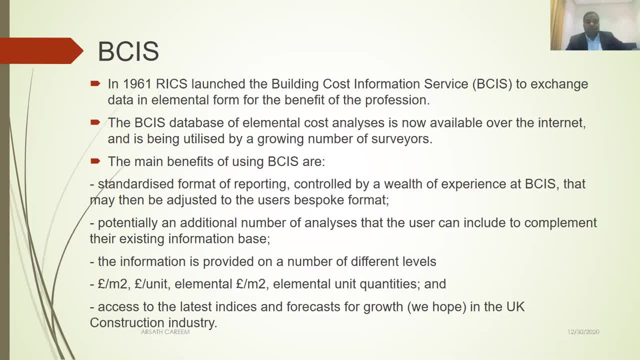 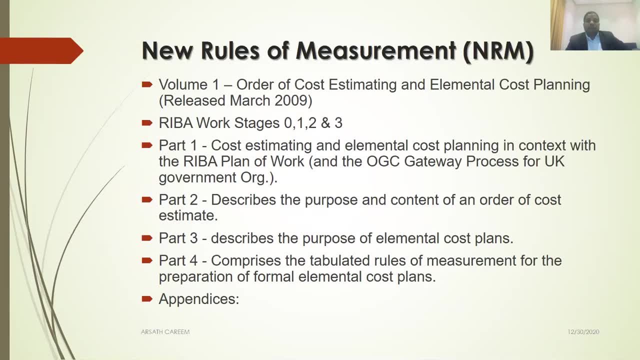 you should know these kind of services available. It's part of your APC process. Also, another guidance available: how to prepare a cost plan from RICS, New Rules of Measurement, which is called NRM, which has three volume: The first volume. how to prepare a order of cost estimating. 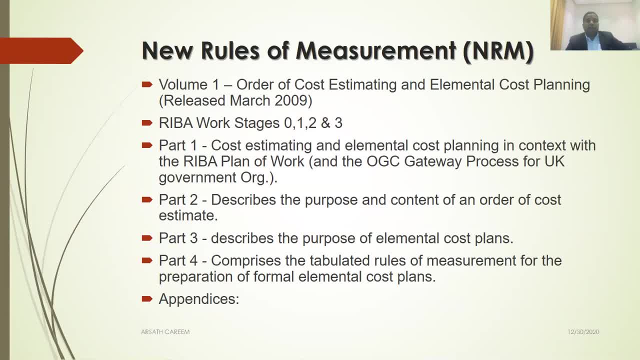 and then cost planning, elemental cost planning. This is useful for work stages zero, one, two, three, which we discussed before. So part one, part two, part three, part four and appendices. This is just for information. 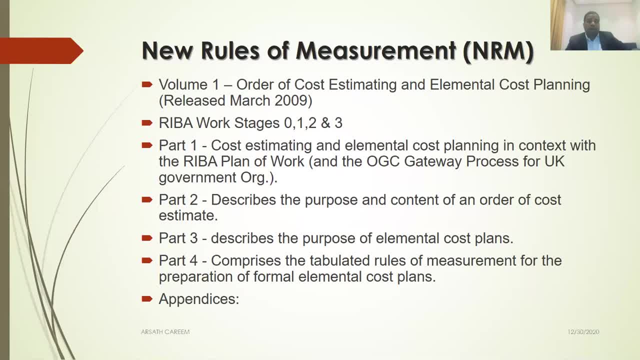 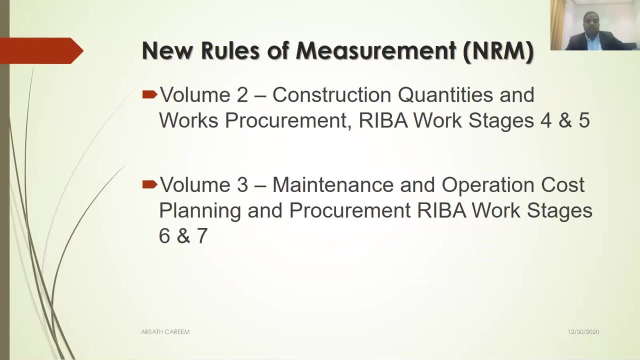 If you want to enhance your knowledge more about cost estimating and elemental cost planning, we can go through this volume Also. volume two for construction quantities and work procurement, RIBA, work stages four and five, which is usable. Volume three: maintenance and operation. 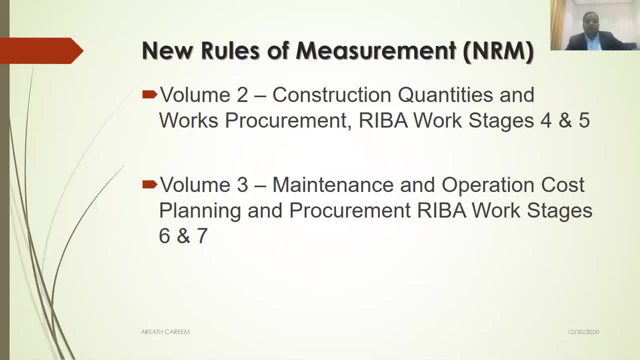 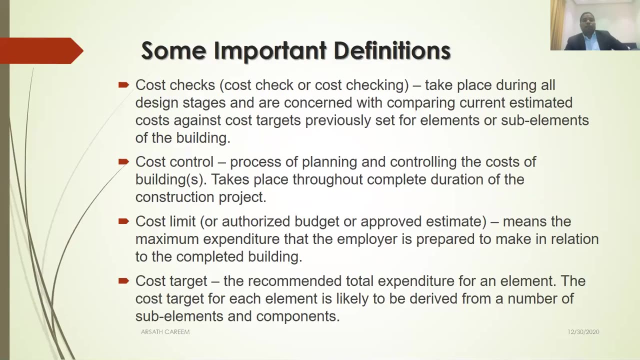 cost planning and procurement. RIBA, work stages six and seven. You will study detail in quantification and measurement competency. Just for your information, I just make these slides. Also, you should know some important definition: Cost checks, cost control, cost limit, cost target. 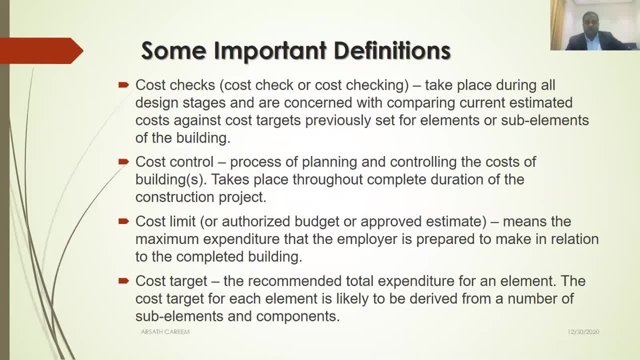 You remember important words of this. I already discussed this in detail. No need to further explanation. What is cost check When you need to know? What is cost control? cost limit, cost target? I explained with the design process in the diagram as well. 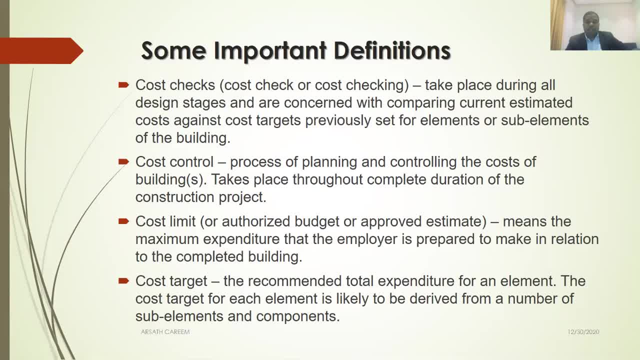 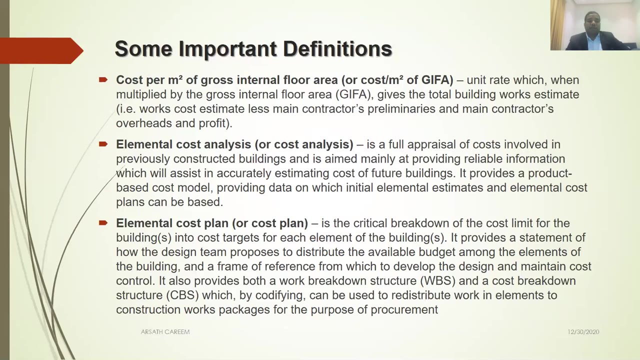 So if you want further information, you can. the same definition which is available in RIC's website, RIC's partway, the volume one, NRM, one you can read and you can understand further to enhance your knowledge. Also, some definition: what is cost per meter square? 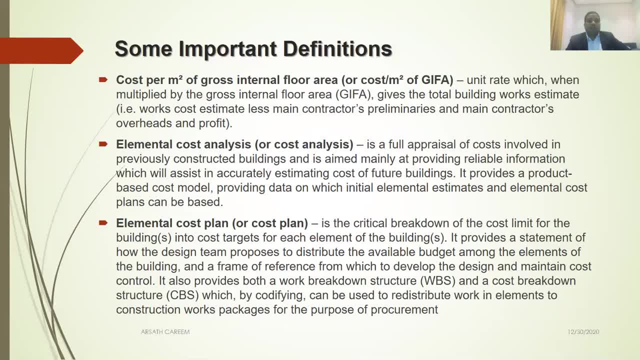 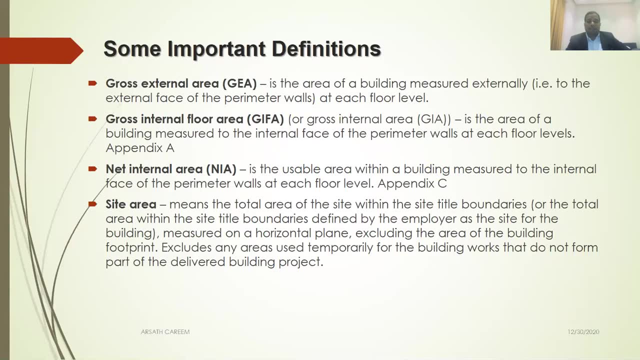 What is elemental cost analysis? What is elemental cost plan? These are definition from RIC's standard definition. You're not necessary to remember everything, Just make sure you know the important things. The same. it's continue So. related question for level one: 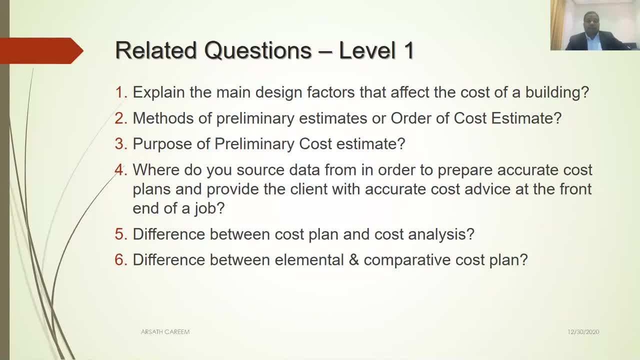 Now we completed cost planning. They may ask the related question. Level one is direct question, just theoretical part. Directly they may ask: explain the main design factors that affect the cost planning? Affect the cost of building preliminary estimates? What are the types? 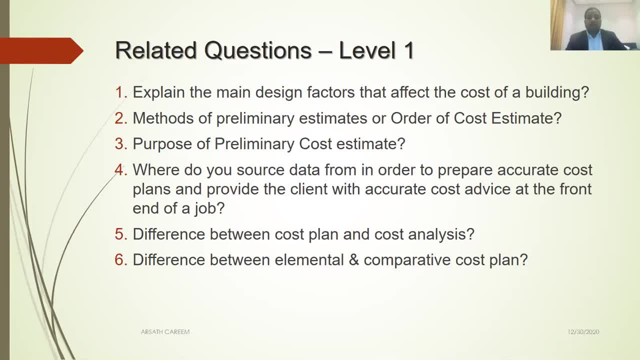 Purpose of estimate? Where do you source data from in order to prepare accurate cost plan and provide the client with accurate cost advice at the front end of a job? Difference between cost plan and cost analysis, Difference between elemental and comparative cost plan: These are the things I have already covered in my slides. 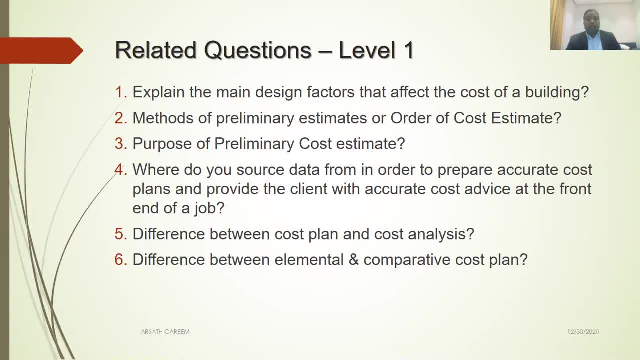 These are the direct question. There is nothing to think about it. Just you remember what it is By understand, by the process, rather than remembering. just understand what is cost plan, What is cost analysis? What type of cost plan available, What is elemental. 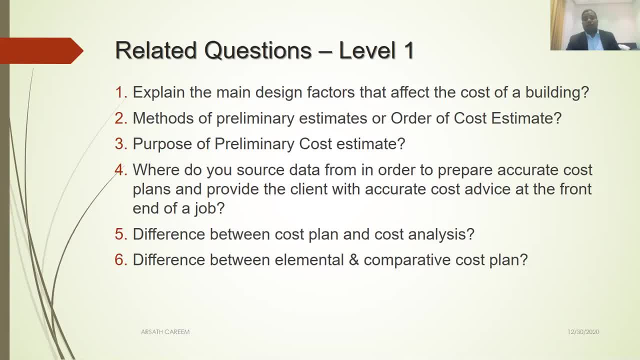 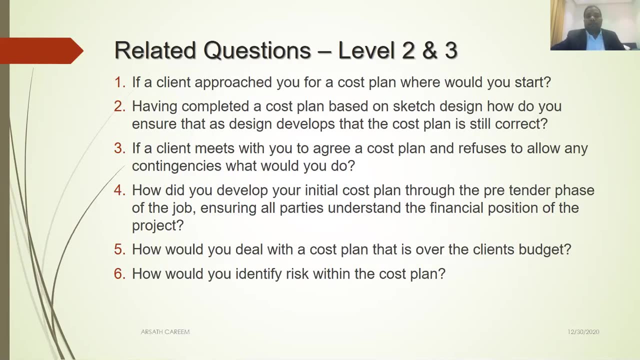 What is comparative? How many types? What are the order of cost you made available. Think the process and understand Easy to remember So you can find easily answer. These are the level one question. COMPLAIN somehow on your questions Level two and three. 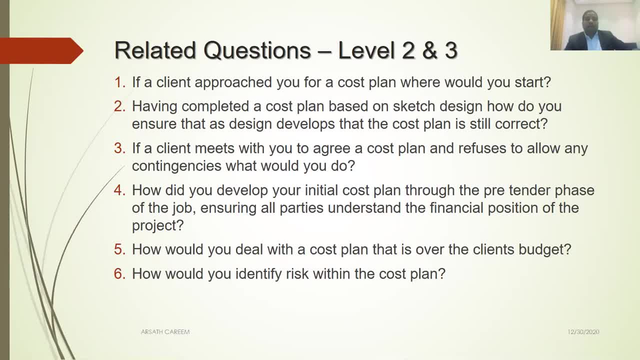 Level two and three. they will not ask directly, They will create, they will create scenario. So you, when they create the scenario from your submission, you have to First you have to understand what they're going to, what they meaning, what they're expecting from you for 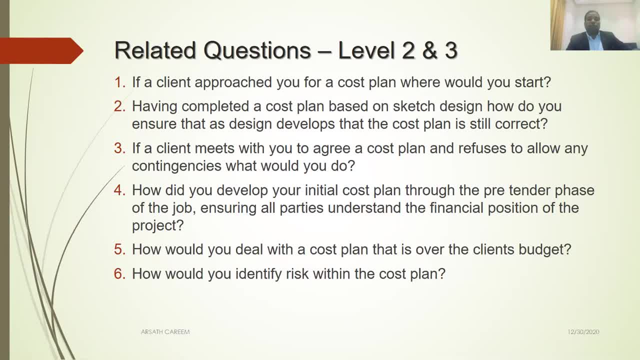 example question here: if a client approached you for a course plan, where would you start? second one: having completed a course plan based on sketch design, how do you ensure that the design develops that course plan is still correct if a client meets with you to agree a course plan and refuses to allow? 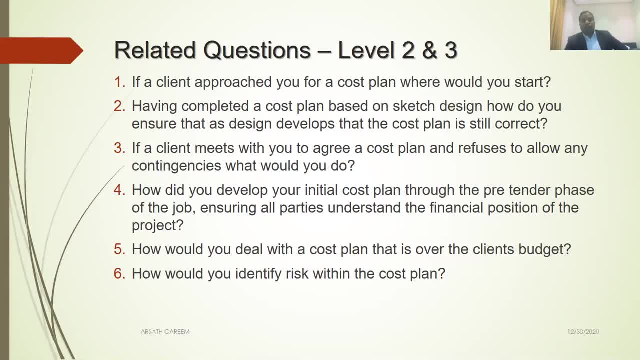 any contingencies. what would you do? how did you develop your initial course plan through the pretender pace of job, ensuring all the parties understand the financial position of the project? how would you deal with the course plan that is over the clients budget? you identify risk within the course plan. so these are the level two and three. 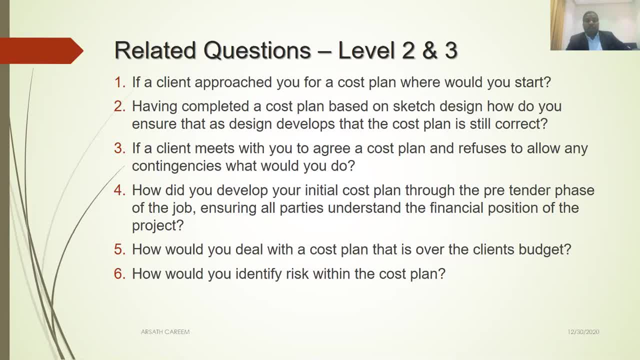 question, sometimes the tricky, but if you know the theoretical part, according to the scenario you should able to answer. now we have limited time, only 20 minutes available. I need to cover value engineering in value management. if you able to answer you, can you try to answer yourself. if not, you can contact me. 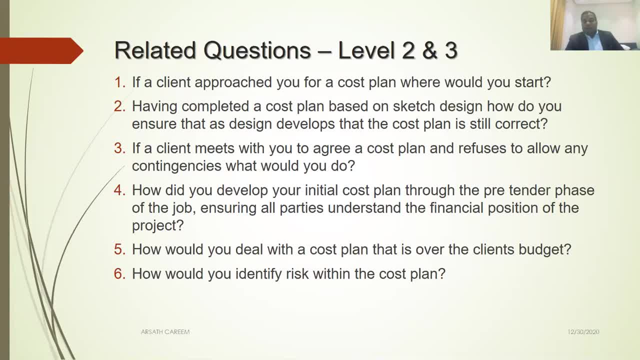 through the. you can contact me through the email ID provided or we have to. we have to set the session for question and answer and separation, because we need to cover value engineering, value management techniques also. so just put on your mind once this webinar finish, and try to answer yourself if you find any difficulty or if you have any other. 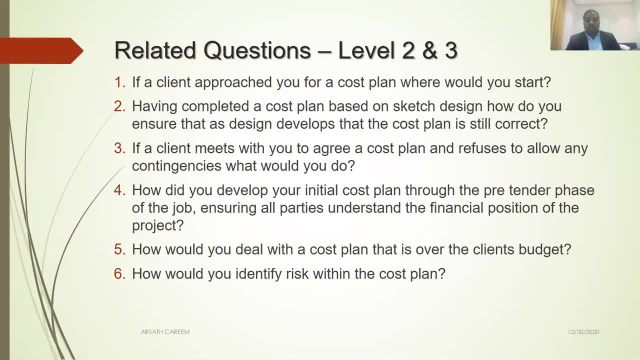 option. another chance to discuss question and answer session. we will discuss further how to answer in a structured way which is expected by the RICS panel. that is very important you are. you are now trying for a chartered qualification, professional qualification by Lancelor. you have to be smart and structured manner. that is what RIC is. 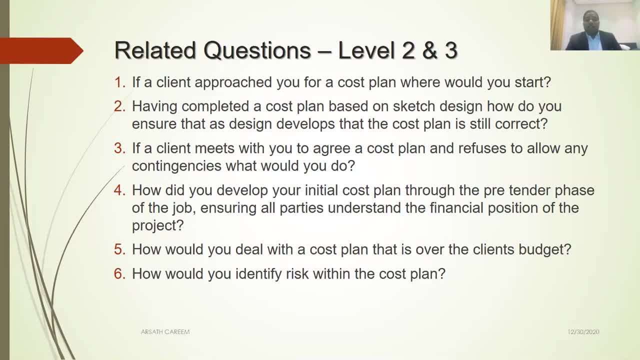 all about confidant answer. you have to answer very confidently and you will notuu. you have to answer very confidently and you will notuu. Also, sometimes, when you ask you have to tell example. during this project, I did this. I give this advice: create more confident yourself to the panel. 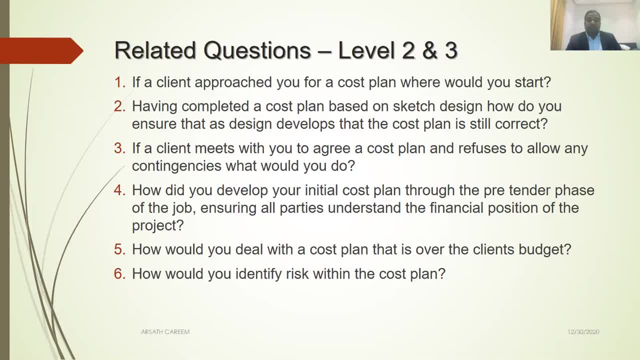 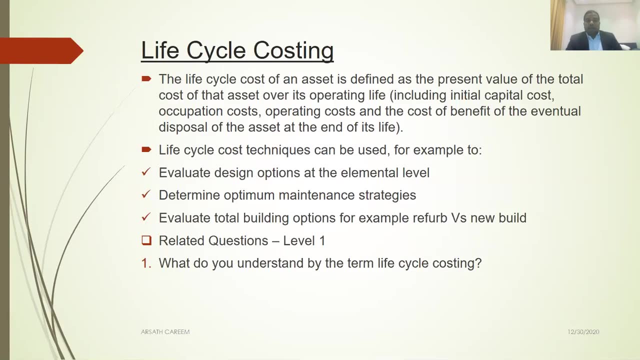 So questioning, answering is a. it's another process. it's a tricky process. structured process we have definitely. we have to arrange another session if time permit. Okay now, so far we have discussed about what is affect, what are the factors affecting. 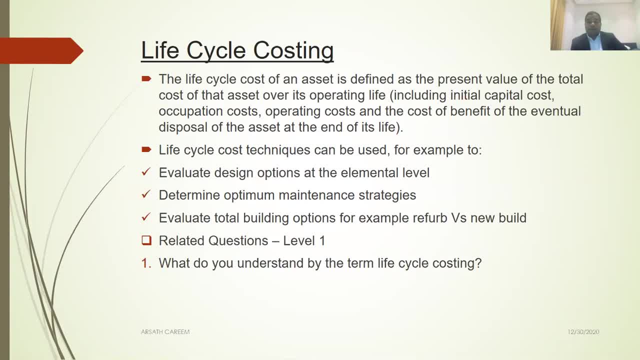 the cost of the building and cost plan process, how to control the cost cost management throughout the pre contract passes. Another terms: you should know what is life cycle costing. In the design economics this is very important word as well, Because every product have a life. 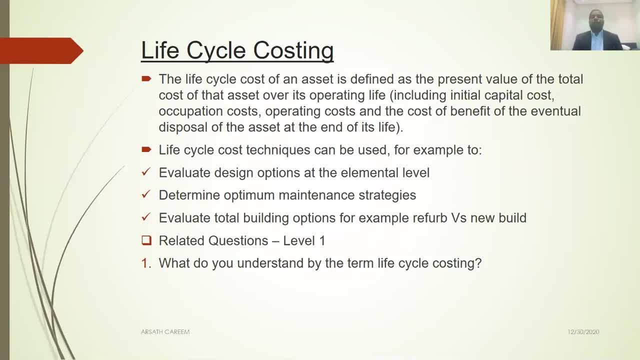 Similarly, the building product also has a life. So you should know the construction part. until you build the building, your part is finished. But still there is a cost, operation cost, maintenance cost, This mental cost. So while you design, designer should consider this one as well sometime when you design. 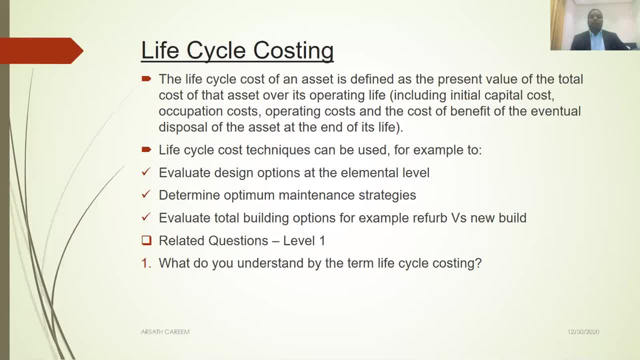 you. if you consider the capital cost for a particular item in the later stage, you might have a operation maintenance cost more than throughout the lifetime of the building. that will cost more to the end user or client. depend on the client objective, for example, if you. 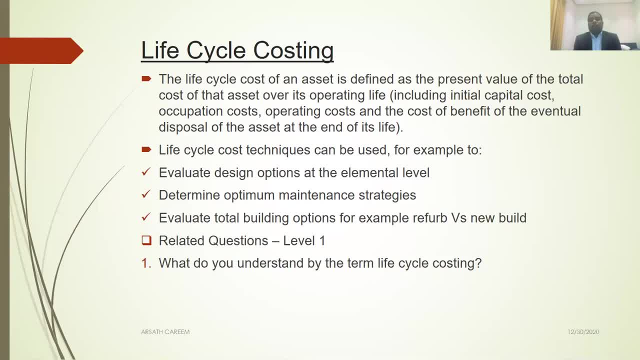 want to rent out, You should have consider maintenance operation cost. if you want to sell out, you have some time- you may consider the capital cost. So these things should communicate with the designer throughout the design process, as well as with the client as well. 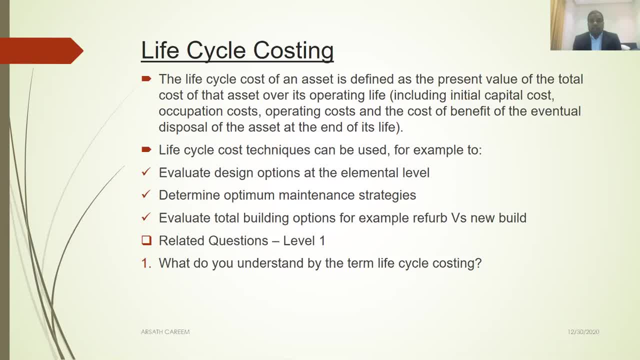 So life cycle cost of an asset is defined as the present value of the total cost of the asset over its operating life, Including The initial capital cost, occupation cost, operating cost and the cost of benefit of the eventual disposal of the asset at the end of its life. 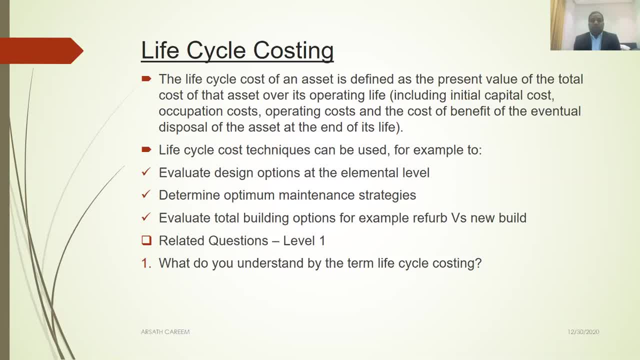 So it's clearly say what I described to you. Life cycle cost technique can be used. for example, evaluate design option at the elemental level. Also determine optimum maintenance strategies. Evaluate total building option, for example refurbishment or new build. So, based on the life cycle costing, exercise as a quantity server. some time you have to. 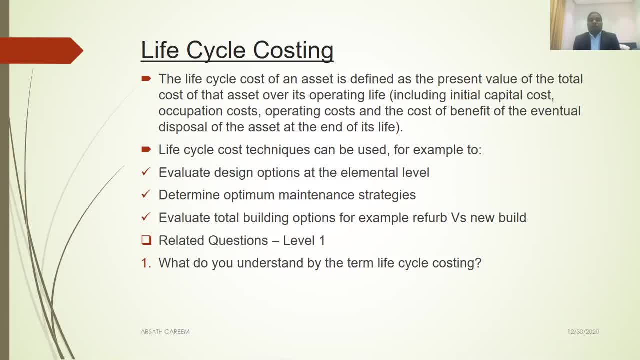 do. For example, I can say: you have, you are designer, you are, you are designing your QS, your designer giving to build a AC, split AC For reduced Time, The cost He. There is two option You can put: non-inverter and inverter. 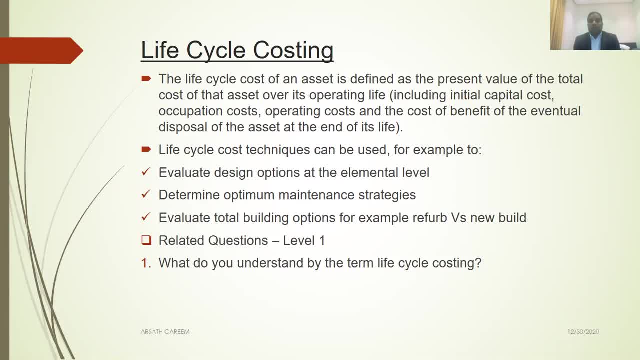 Okay, Non-inverter: Usually the capital cost is less, inverter The capital cost is more. but operate, operation, maintenance cost less for inverter because it will save the electricity. So these are the one example for life cycle costing exercise. So you can calculate how much additional electricity, how much monthly cost extra you will get for. 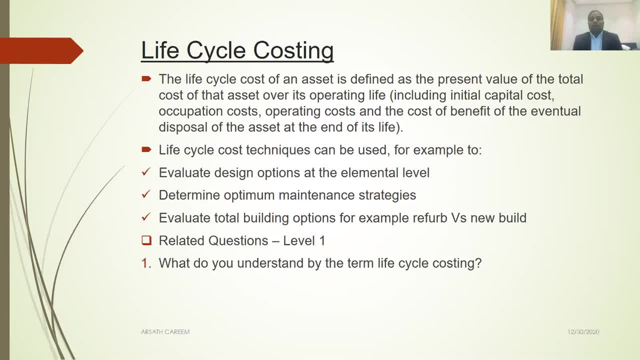 the non-inverter, and for one year how much? for so you can and it is a quantity server. You have to do analysis and you have to advise your client later to life life cycle costing. There will be level, usually level one question. 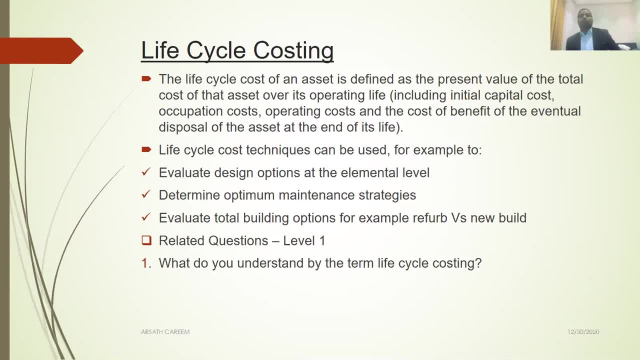 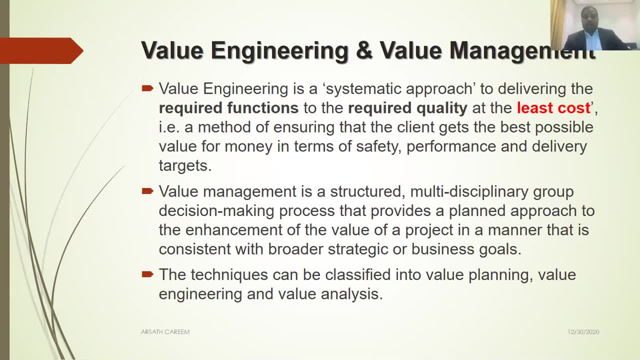 What do you understand by the terms of life cycle costing? So you can elaborate simply. finally, we are moving to value engineering and value management. Value engineering is a systematic approach to delivering the required function to regard quality at the least cost, method of ensuring that the clients get the best possible value. 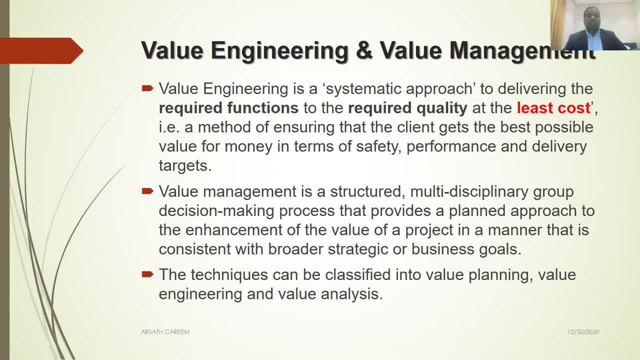 for money. Okay, Now we are coming to our engineering management. Now we discuss about the design economics. what factors are affecting the building cost? what is cost planning? What is cost analysis? What is preliminary estimate? Suddenly, why we need what is value engineering and value management? 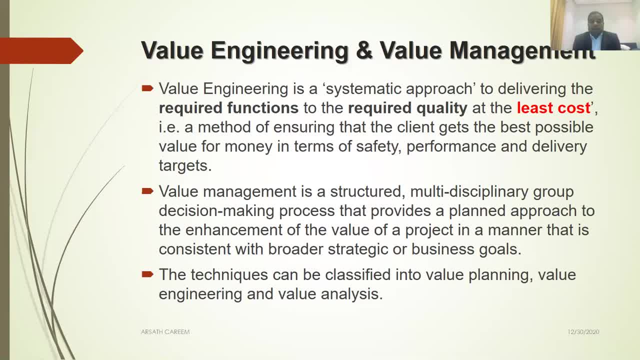 What we are discussing: pre-contract cost control mechanisms. one of the mechanism: mainly, we use cost planning. okay, we use cost planning throughout the design process. unfortunately, your budget over over. you not able to design the building within the budget, so what mechanism available to reduce the cost? that is how the value engineering taking place here, the value engineering. one of the 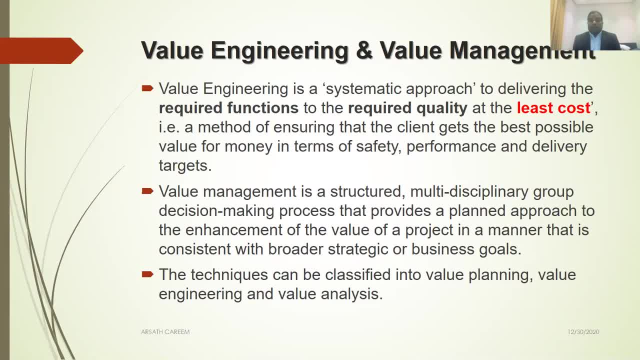 major tools to bring the budget back. so basically, for rics, apc process. they may ask: well, what is value? what is the difference between value engineering, value management, how you have any experience with value engineering in your, in your project, when the budget is over to your, when the budget goes over to your limited cost limit, what you will. 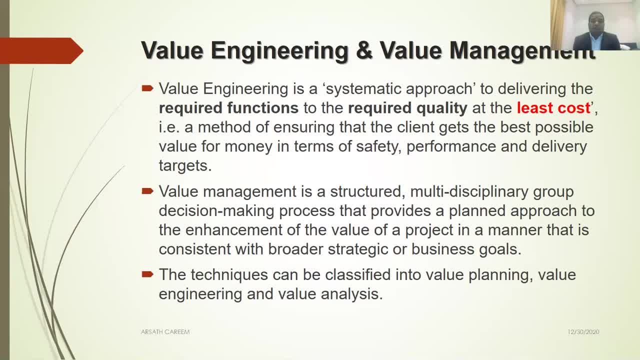 do so you, you have to answer using the value engineering techniques. okay, to remember what is value engineering, you should know delivering the required function to the regard, quality at the least cost is very important words to remember that function. look at quality for the least cost. so, value management, volume management, including, which is include, value planning. 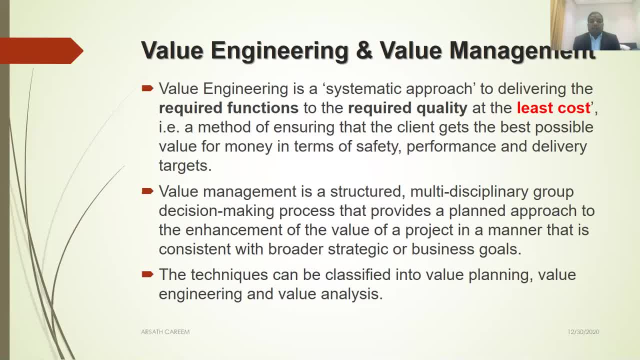 value engineering and value analysis. value engineering: part of the value management. so what? volume management is a total process, value engineering part of it. what is definition? you can read and understand that the techniques can be classified into value planning, value engineering, value analysis. this is a very important part of value management. 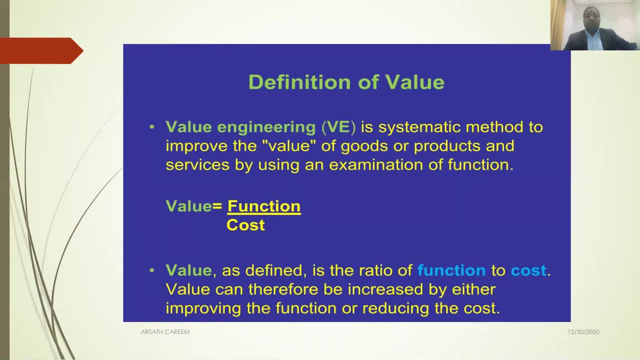 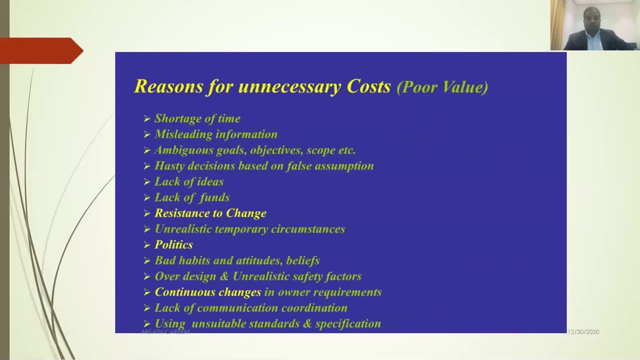 there is another definition available for value engineering. it's a systematic method to improve the value of goods or products and services by using an examination of function. what is value? function over cost? okay, now reason for unnecessary cost generally: why we cost overrun, cost our more than our budget. why, why? what are the reason? as a human, it can happen. 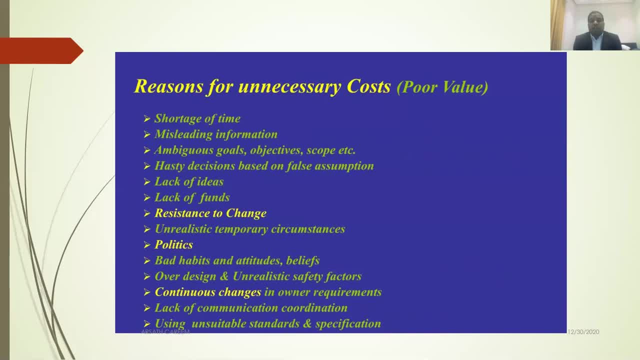 generally when you are, when you do investigation, what are the reason for unnecessary cost happening in the construction? shortage of time? usually we're trying to complete the project short period, misleading the information. as a human, sometimes the information in inaccurate is theissions loosening the image of the female. for even by creating 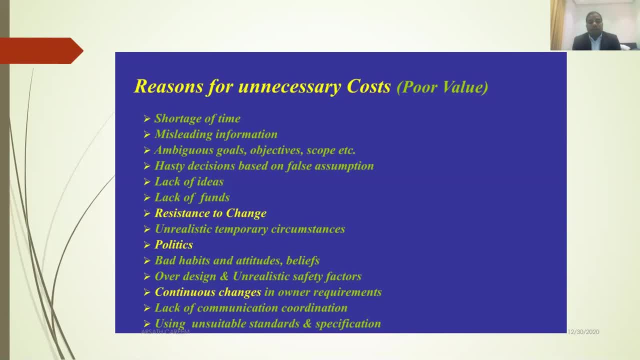 the species's stuff. it also continues to hire if you head directly from what is called arms decision some. what are the issues about? giving up lesions, but not for the only access? they G balls. objectives, scope, lack of ideas, lack of funds, resistance to change, unrealistic temporary circumstances, some internal politics, bad habits over design, unrealistic safety factors, continuous changes to owner requirements, lack of communication, temporary domestic geral. 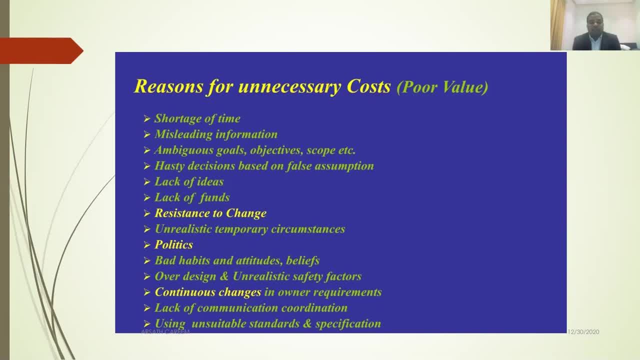 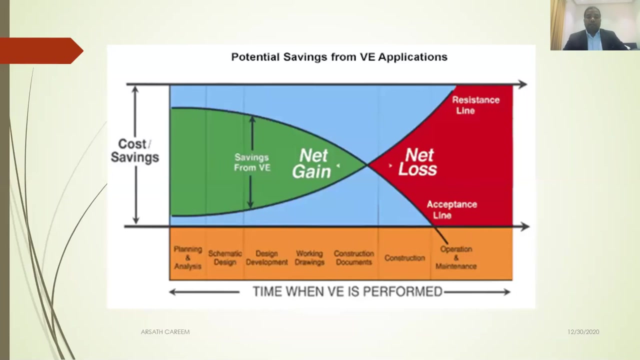 policy, net coordination using unsuitable standards and specification because of the reason there may be cost overrun. so how to bring back cost within the budget? that is what value engineering coming to application. this is the potential serving from value engineering application here. these are the stages of the design. maybe that name is different from the current name, which? 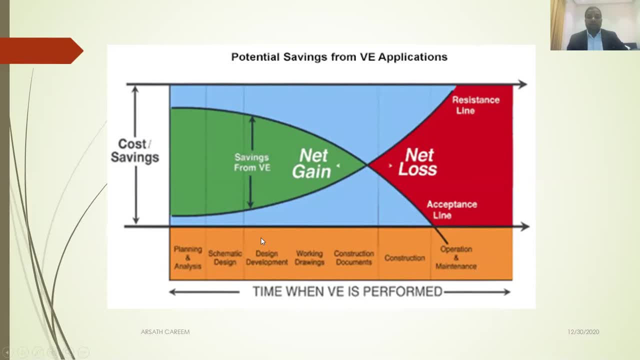 strategic definition plan and brief concept design. this is previously used name, however, the same. there is a potential serving from value engineering in early stage. if you do value engineering from concept stage, there is 10 to 20 percentage chance for reducing the cost. this is from research, so value engineering should be carried out early. 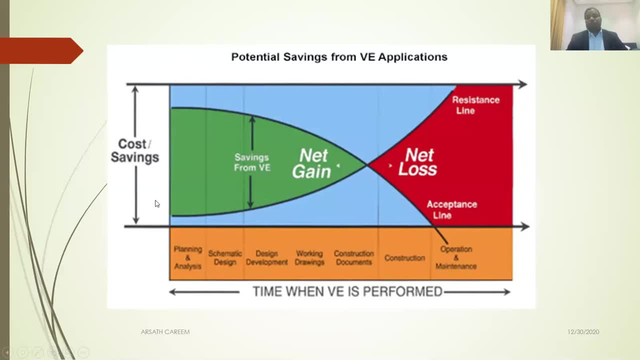 stage depend on the project value, because for a small project if you establish a value engineering, the initialization of value engineering, that will cost more than we are saving. so it's most suitable for a big project if you want for a big saving. how you can do value engineering, I will give one example below. so later stage, if you do. 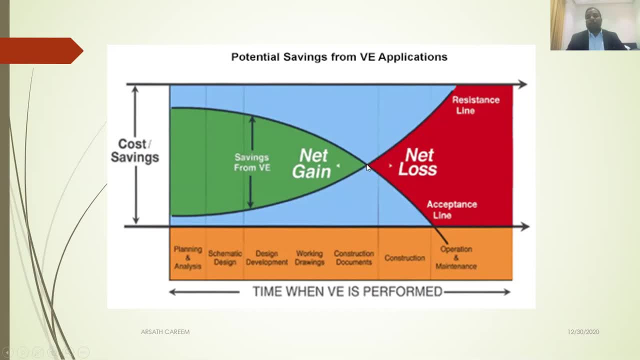 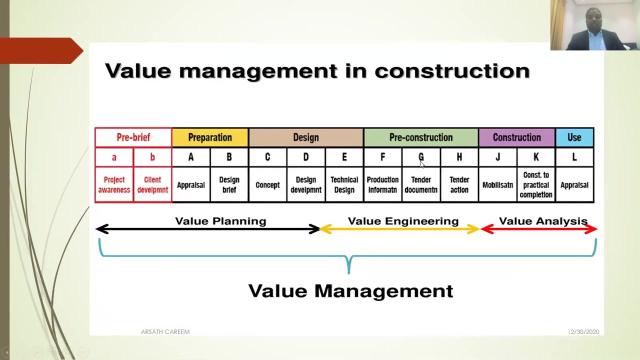 in the construction, the saving chances very less. however, recently introduced FIDIC is suggesting for value engineering in the construction stage, even though the best time to do conducting value engineering for best performance is early stage value management in construction. we study about value engineering, environment and by theoretically, these are the design. 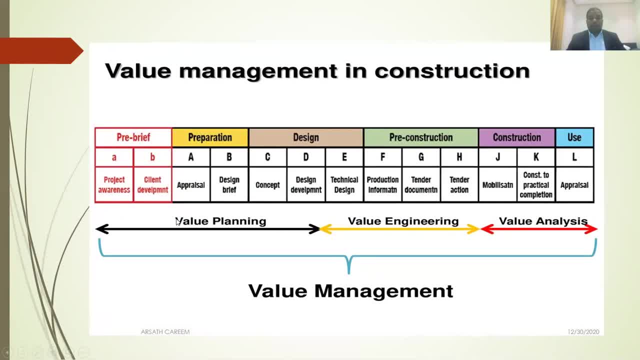 stages, usually the value planning, start from this brief and it will go up to design development. this, this design stages- not applicable for current design stages. not applicable for current design stages. not applicable for current scenario: current RIBA plan of work, but it's a name changed. now only eight. 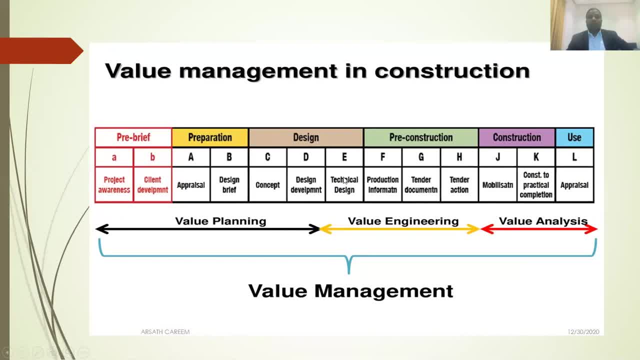 stages, previously around 13 stages. however, what I trying to say here, value management, is a combination of value planning, value engineering, value analysis when you have to do value, and value planning during the initial design stage. when you have to do value engineering, you can do from concept. 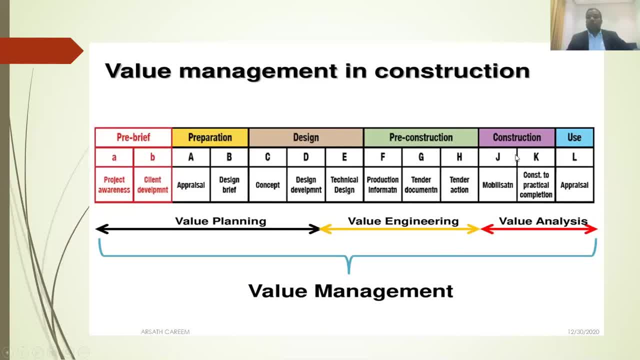 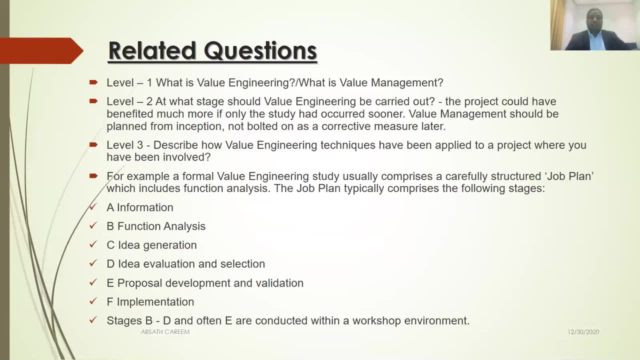 also design development, technical design. when you have to do value analysis, you have to analysis you what you design after construction. related question to value engineering directly: what this value engineering? what is value management? level2? they may ask what stage value engineering to be carry out. you the project would have benefit much more if only the study had occurred sooner. value management. 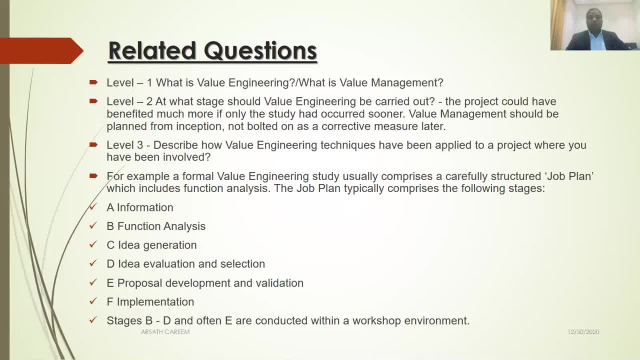 should be planned from inception, not bolted on as a corrective measure later for a level three question. describe how value engineering technique have been applied to a project where you have been involved. so you have to give example. where are you involved with value engineering? for example, a formal value engineering study usually comprises a carefully structured job. 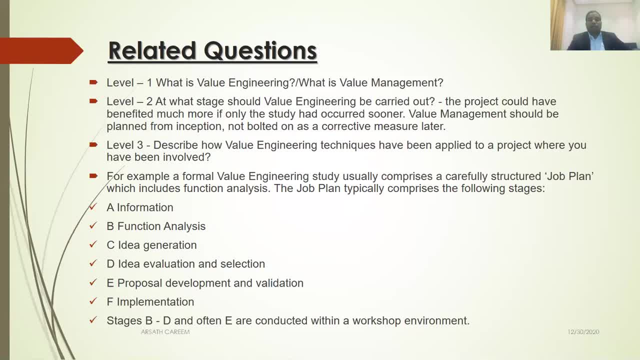 plan, which includes functional analysis. the job plan typically comprises the following stages: the initial step of the value engineering- there is a. six steps is here. first, you have to get the information of the project. the initial step of the value engineering: there is a. the initial step of the value engineering: there is a. 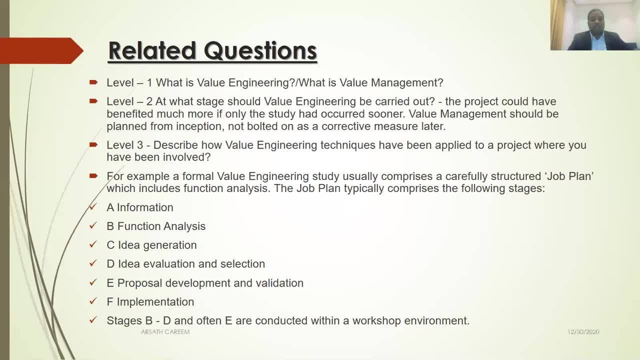 then you have to analysis, you have to do analysis of the function, then you have to get the idea, you have to generate the idea and idea. evaluation and selection, then proposal development and validation, implementation. these are the steps of value engineering for you as a level three, in order to 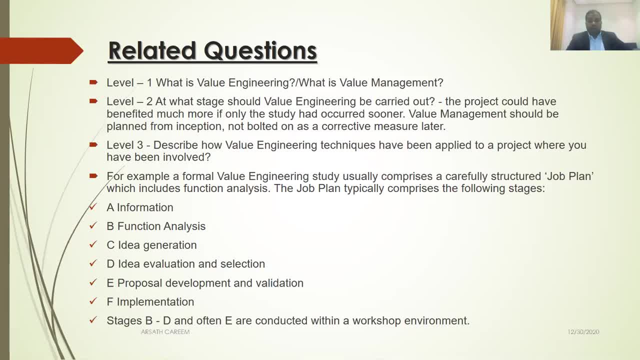 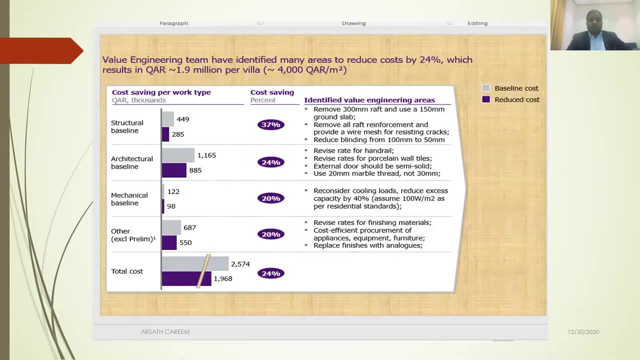 answer level three, that question. first you have to tell the steps of value engineering. it better to answer: start from what is value engineering, then steps of the value engineering, then you have to give example where you have been involved. this is the project i have involved. for example, when you, when you read this: 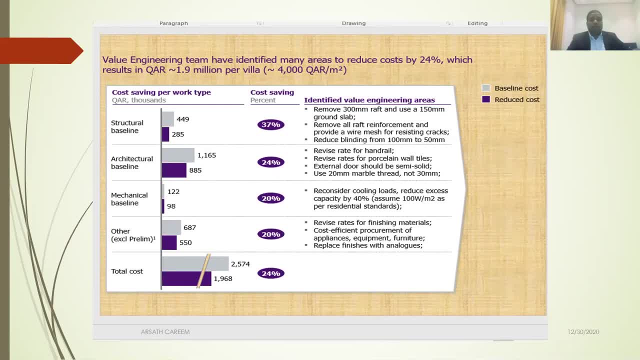 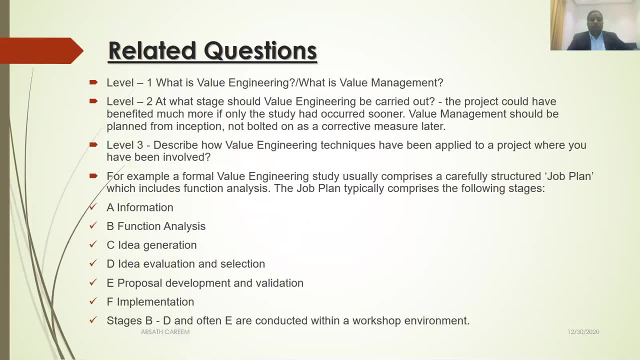 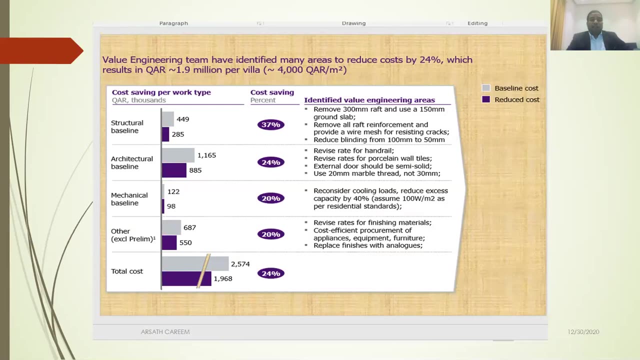 slides, you will understand usually how it is. what is value engineering, where i work, for example, if if assessor ask with me where are you involved in the value engineering, how you conduct it, i will answer like this: i involved in a villa which is. i have to reduce the 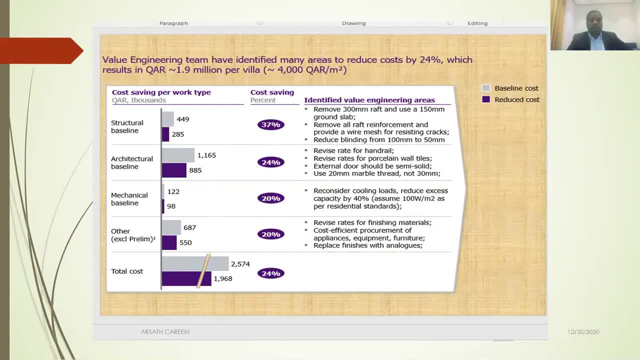 cost by 24 percentage after technical design. when i checked my cost cost update, my budget was to be cost 2 million, which is here, but when i, when i measure the cost, it is come 2.5 million. so i advise my design team, which is over budgeted. 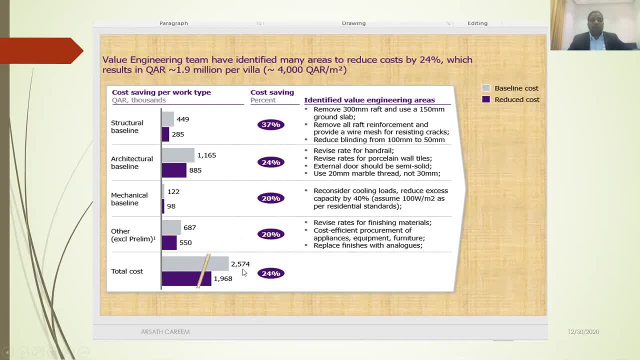 so i have to reduce to 2 million. then only this project feasible to me because i am an investor, because i have to, i have to build this villa and i need to sell it. already the project value set out selling price was 2 million. i had my profit 10, so my selling price 2.2 million. after design i identify: 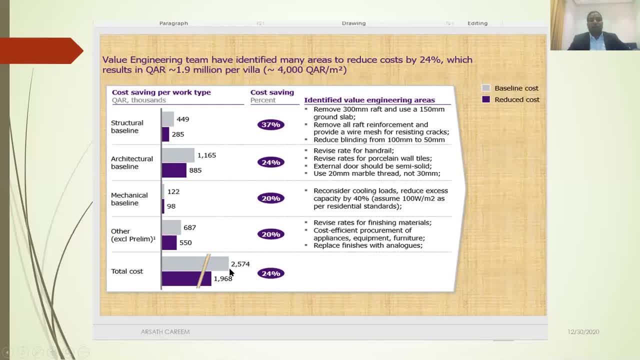 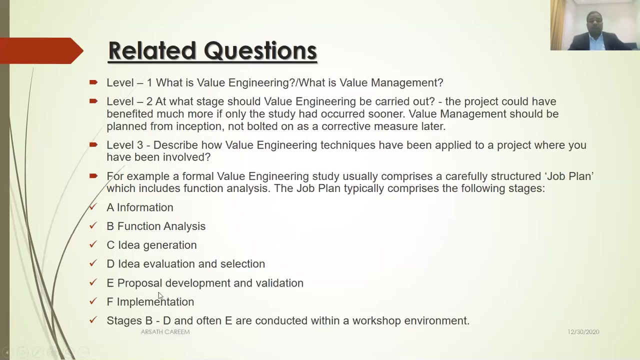 i evaluate my cost 2.5 million, so i have to reduce 24. so in pre-contract stage, what mechanism we have to take? I have so the best mechanism which I can use: value engineering. how I did so? I follow these old steps A to F as a quantity surveyor and the I am a part of. 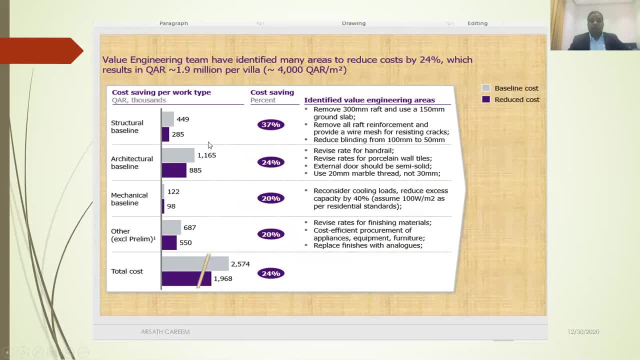 the project team. it is include project manager, my company. what they did? they appoint a consultant to to conduct a value engineering exercise, because usually value engineering should be guide by the experienced people. normal even we are quantity surveyor. we only do the estimating on cost plan part. we can. 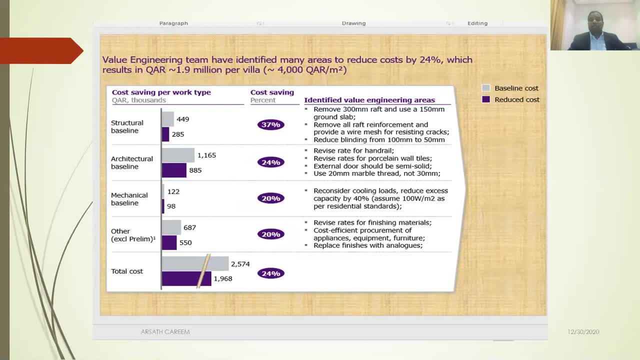 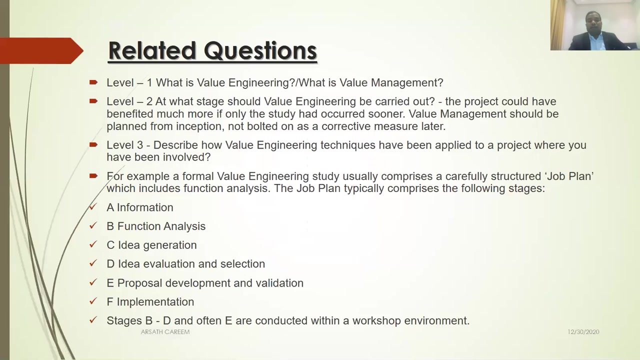 advise regarding the cost only. that is our expertise. we don't lead the value engineering. what we are part of the value engineering. so my company appointed a consultant who are specialists in value engineering. they collect the information. but they did. they collect the information and, as a team, I am part. 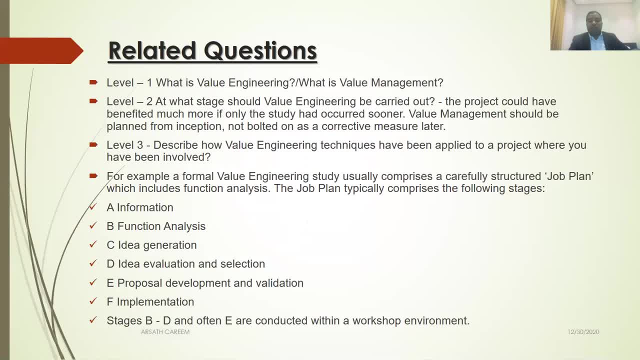 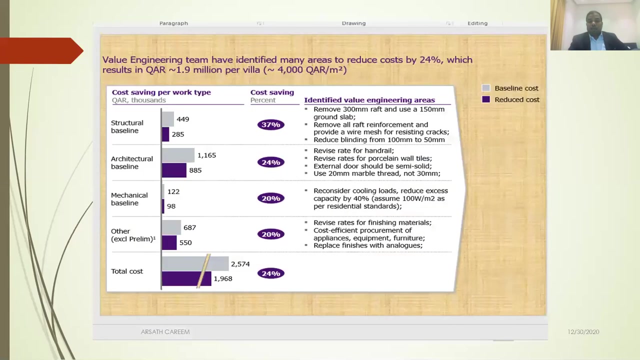 of the team I, what are my function, cost, cost advising also my project manager or the design team? structural, electrical, mechanical, we all together we did functional analysis, every function, substructure, foundation. so we, after analysis, we identified ideas where we can reduce our design, where we can provide best value for money through. 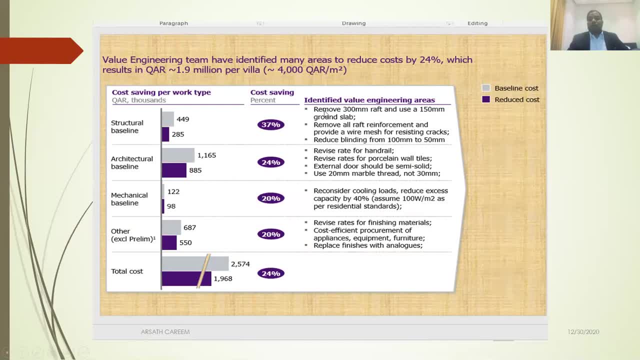 the design. so our team identified: we use 300 millimeter draft, which is over over design. so instead of that, one hundred and fifty millimeter ground slip is enough. so these are the things we identified: remove all raft reinforcement and provide a wire mesh for resisting cracks. reduce blinding from 100 millimeter to 500 millimeter. so 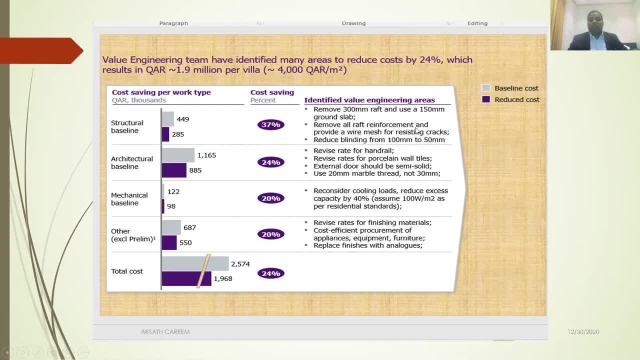 we identify: structural, these elements to reduce the cost. architectural rewired in order to reduce the cost of the craft from the design. and they work. and we also have fixed a quarter meter and mister line. we have finished them and this is the only time we can do a check it now, so it is done in five minutes. 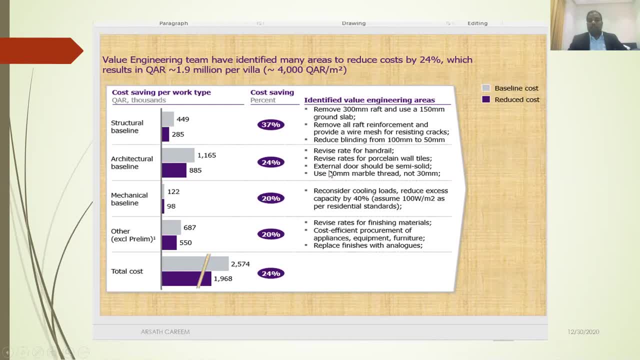 after we finish the system, we decide that we are going to finish this. we have to finish this after the construction and finish it for five minutes, and also in the two days after the construction we have to finish it for a third of the day to be able to finish it again. so we have to finish. that work is finished. 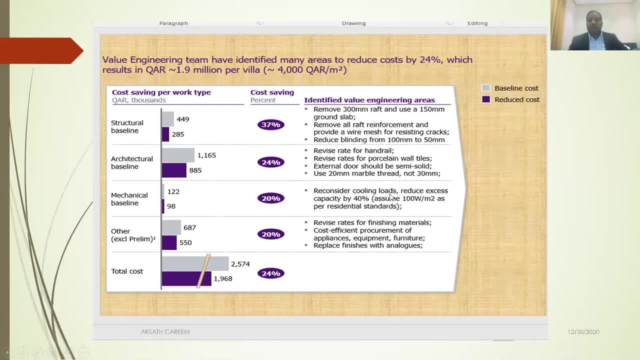 this work is complete. we have to complete it. we had to finish it. we are going to finish that work anyway. we have to finish it now. so the half hour we are required, quality, least cost, so whichever we can. also for mechanical, we consider reconsider cooling loads. excess capacity also for other item, revised rate for finishing material. 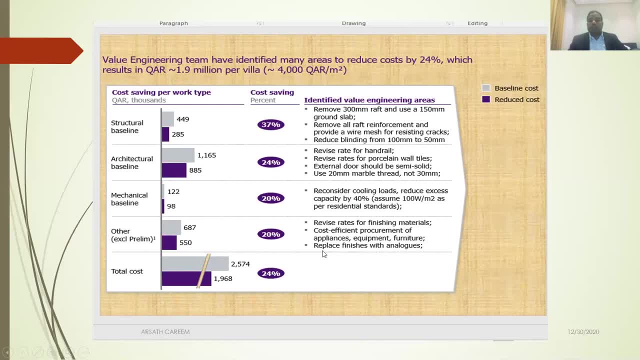 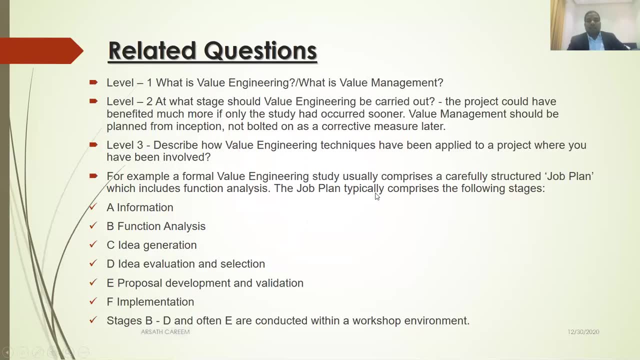 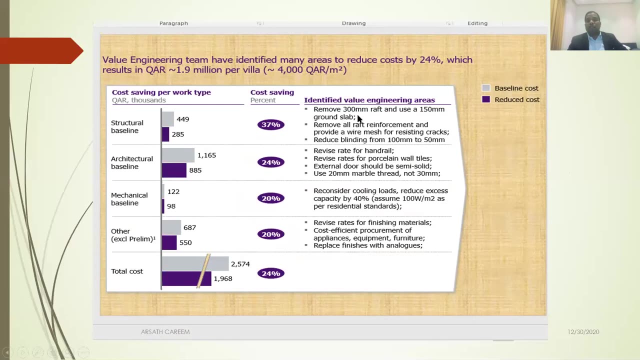 cost efficient procurement: appliances, equipment, furniture, replace finishes with analogs. so after we generating these ideas, then we did evaluation: once we change this ideas, how much we can save each item. so after when architect design team generated the ideas, my task is to cost check again, cost plan again, cost estimate and cost check continuously. 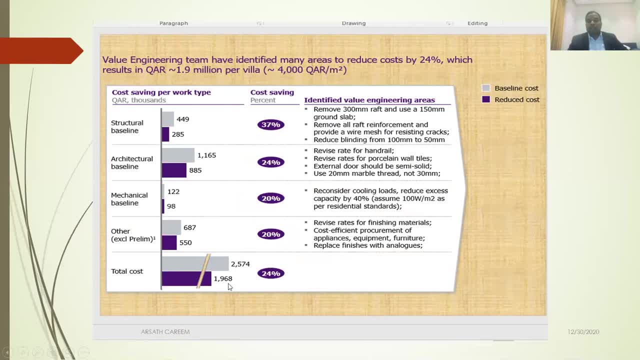 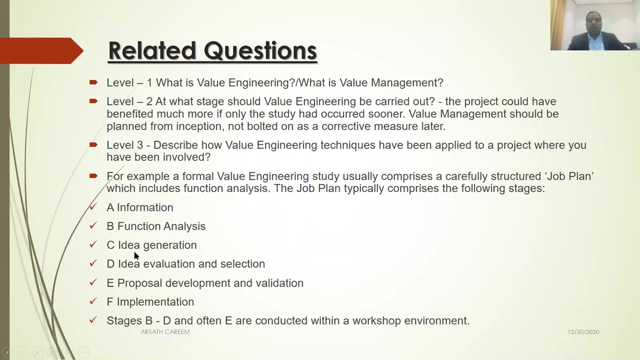 each item. then we arrived 1.96, which within our budget. so this is one of the example. so these are baseline cost and the dark color this one radius cost. so you have to simply answer, using this job plan, how you idea generated. if you did exactly, you will remember the steps. you can easily 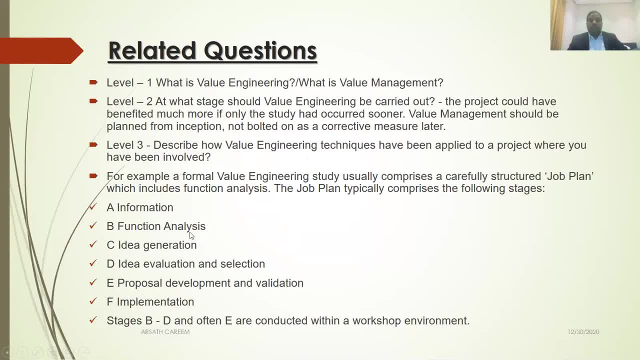 answer if you write in your summary of experience: i conduct a value engineering for my project in order to reduce the cost. that is a definitely ask: how? how did you conduct? what is the process? or they will ask they will also. they will create some scenario after evaluation: proposal development. 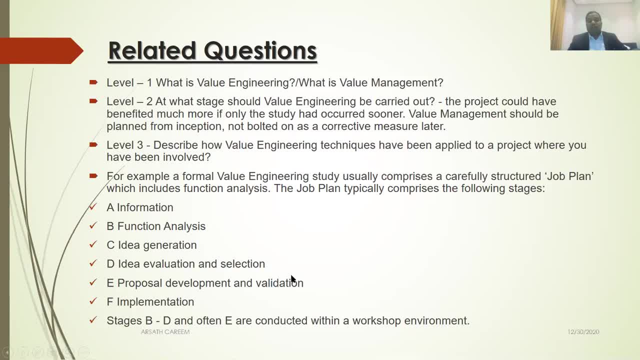 and validation. so the the designer will check the design codes and everything in the validation which is which affect anything or how it will impact when you redesign these things. when everything confirmed, we have to implement this will send to client. after client approval, we will. we will change the design and resubmit. so this is all about value engineering. 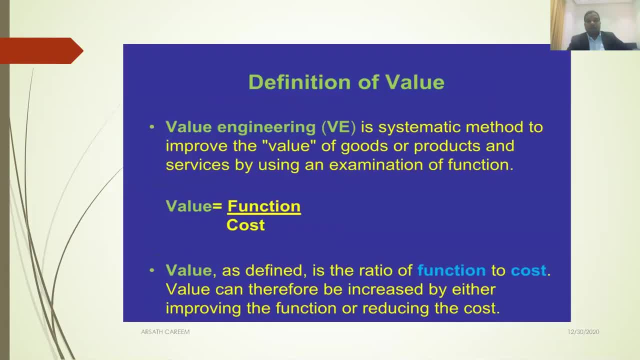 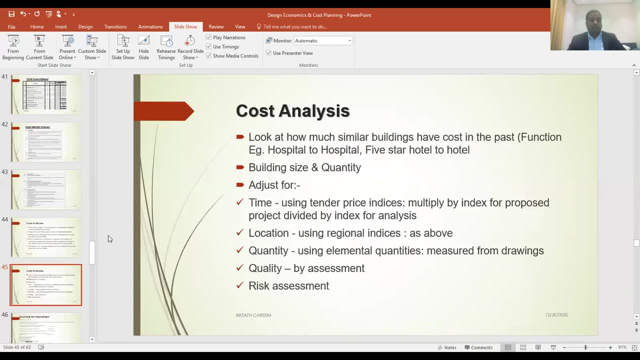 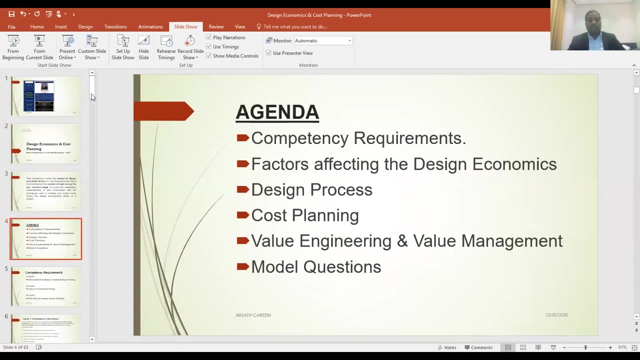 so last two hours. i hope i cover all the topics which i i put in my content. so only thing i didn't explore the question and answer in detail, i just went roughly. so when you look at this agenda, i covered everything. i hope you learned from this session.